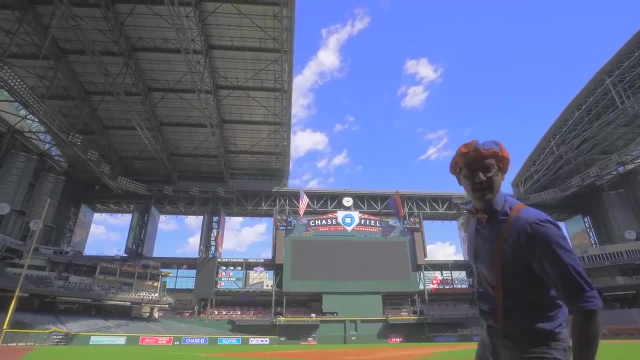 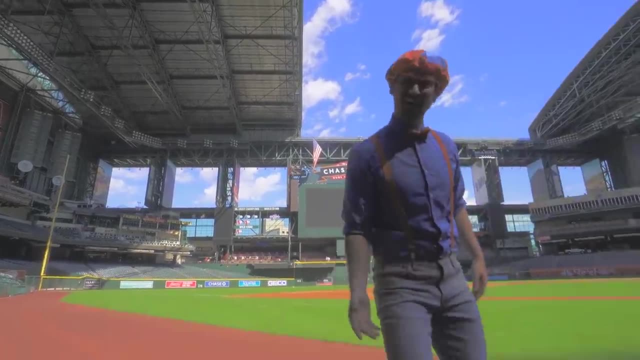 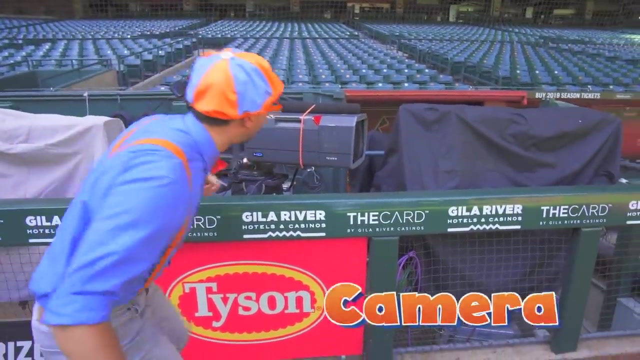 One side is closed and one side is open. They can close it if they want shade and they can open it if they want sun. Pretty cool, Come here, Whoa. Look at this. This is a giant camera. All right, Hopefully I'll- they're not coming to see me take out the lights. 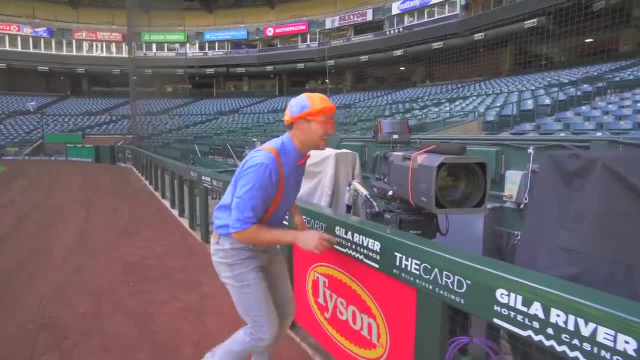 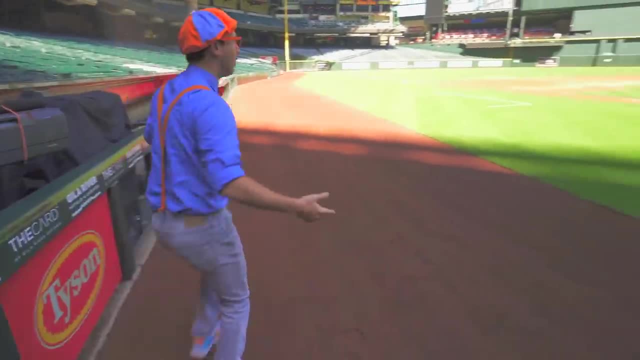 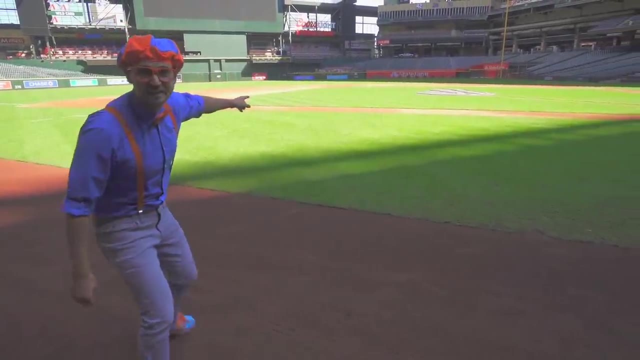 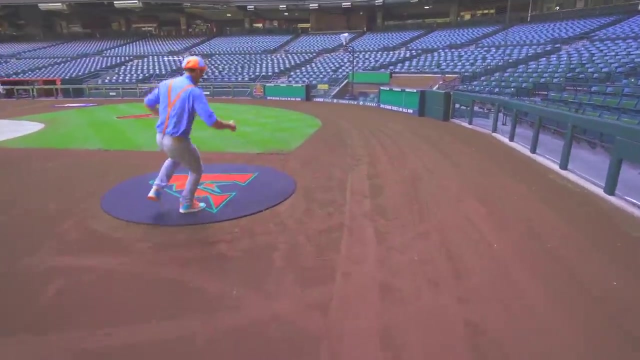 Hello, Hello. This camera is used to be able to see all the players really far away: The players in the outfield, The outfield, Whoa- Look at how far away it is, Whoa- And then the infield. It's a lot of cool dirt and over here. 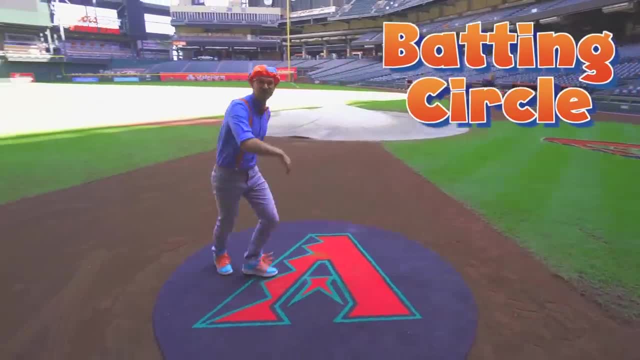 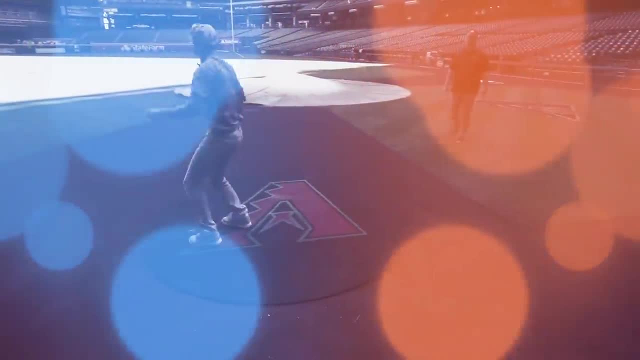 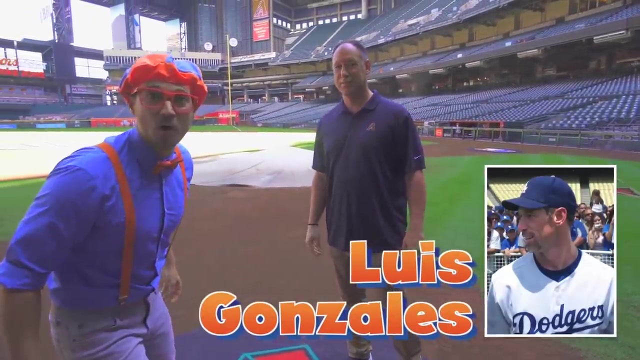 Batting circle. Whoa, This is where the players warm up and bat. Whoa, hey, who are you? Hi, Blippi, Hey, I'm Luis Gonzales. Whoa, Luis Gonzales, Do you play baseball? I used to play baseball. now I win baseball. 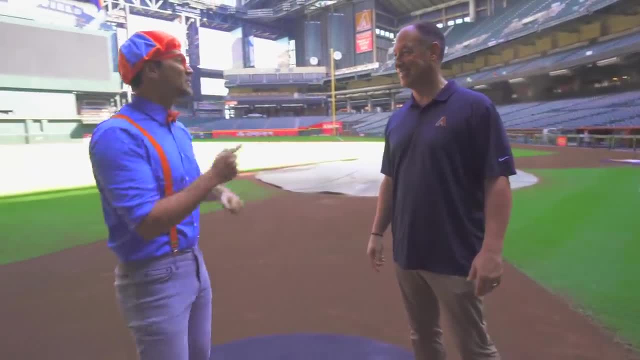 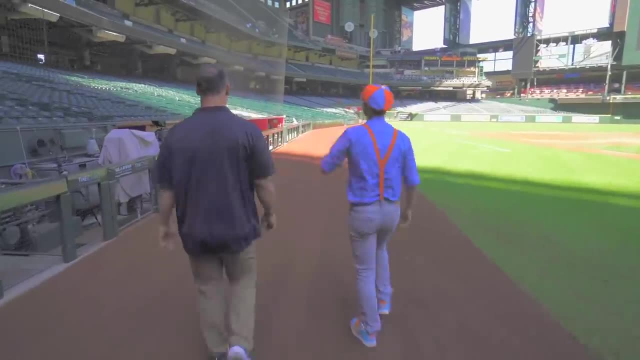 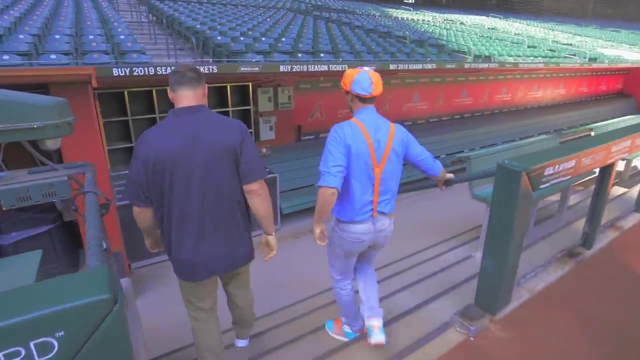 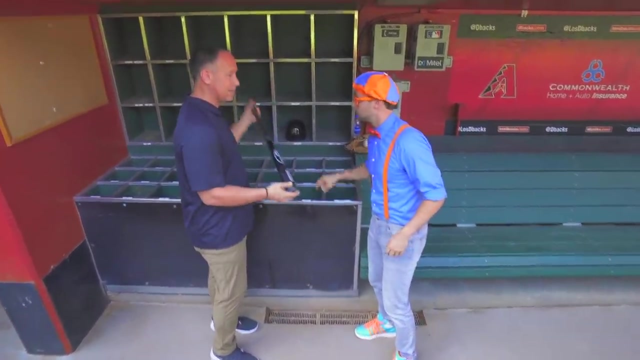 Oh, he win baseball. Will you teach me some tips and tricks? Sure, let's go. Okay, come on. Okay, back to the dugout. Whoa, pretty cool. Well, Blippi, to play baseball you need a bat. 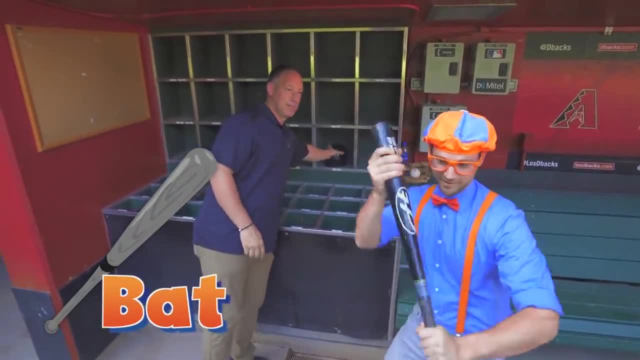 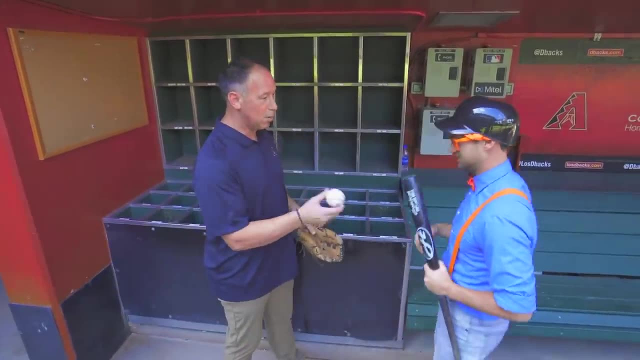 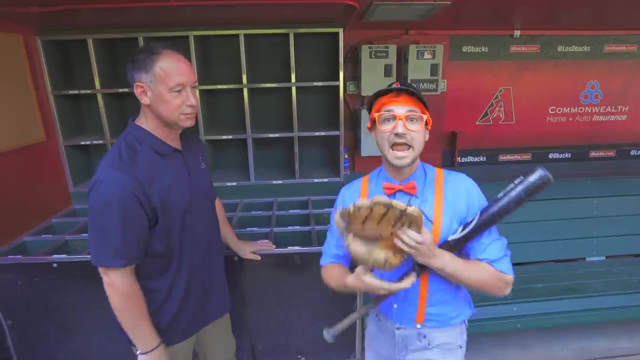 Ooh, a bat, check it out, Pretty cool. And a helmet- Ooh, a helmet, sweet, All right. A ball Ooh, a baseball, Wow. And a glove: Ooh and a glove Ooh, pretty cool. now what? 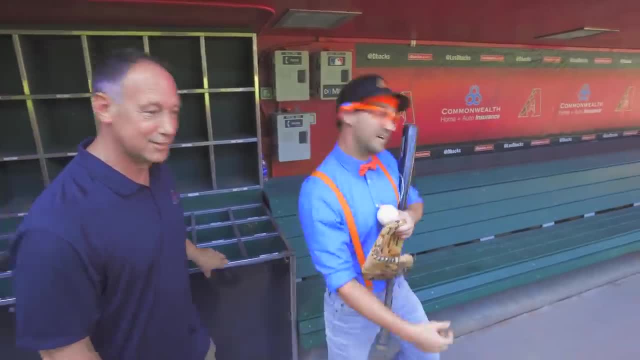 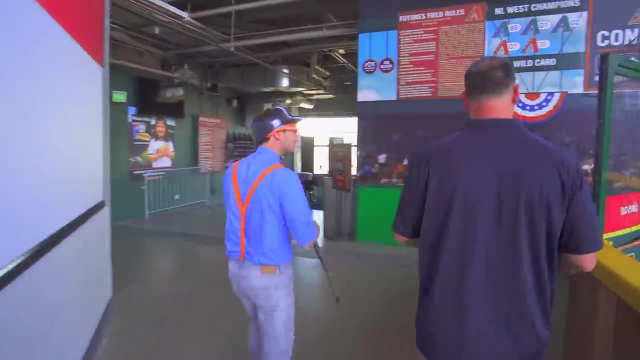 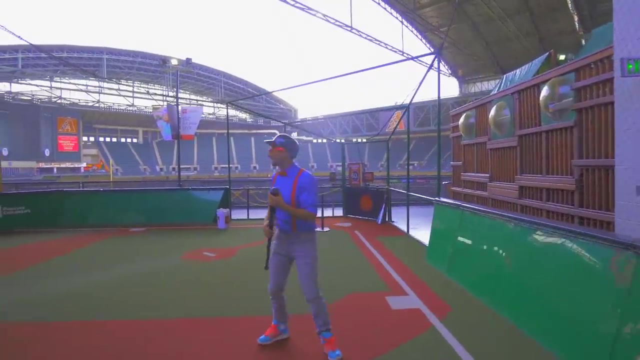 Now let's go to the sandlot so you can play baseball. All right, let's go. Thank you, Whoa, whoa. what is this place? Blippi, this is our sandlot. This is where we're gonna teach you how to hit. 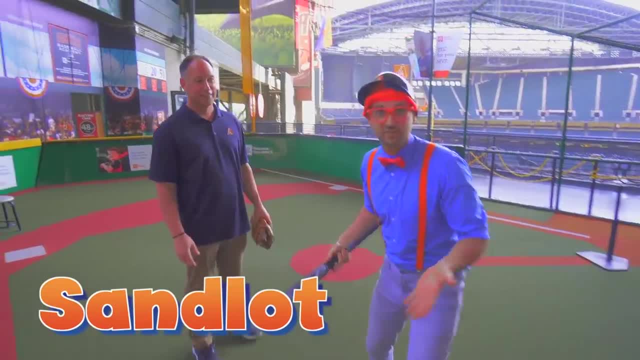 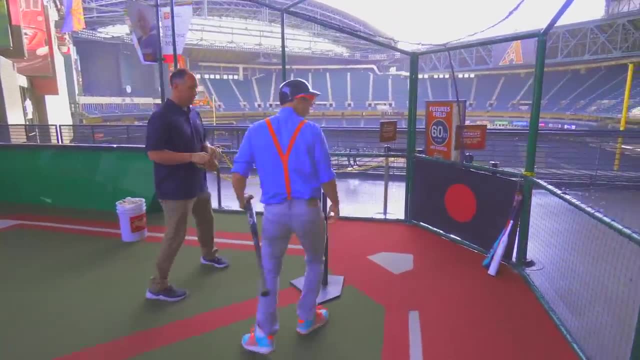 Ooh, this is the sandlot. he said It's a small version of the baseball field and I'm gonna learn how to hit. Okay, Are you ready? Yep, Oh, what do I do here? This is a tee. 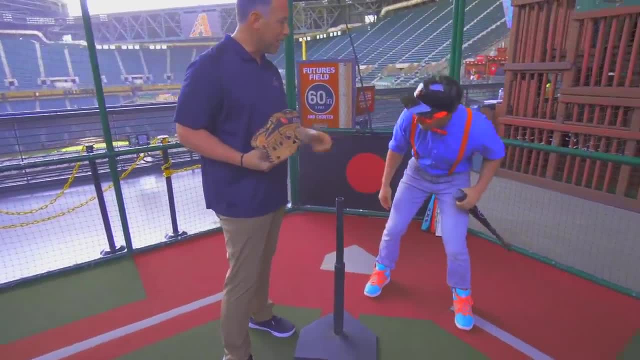 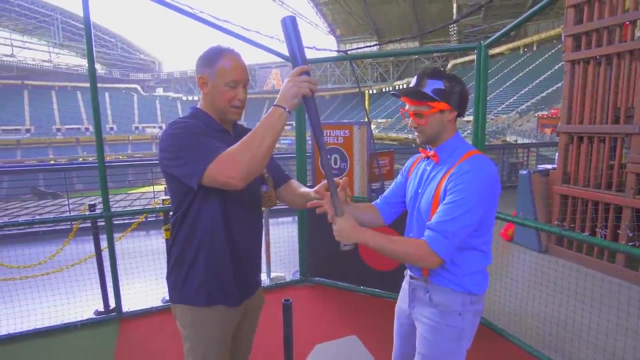 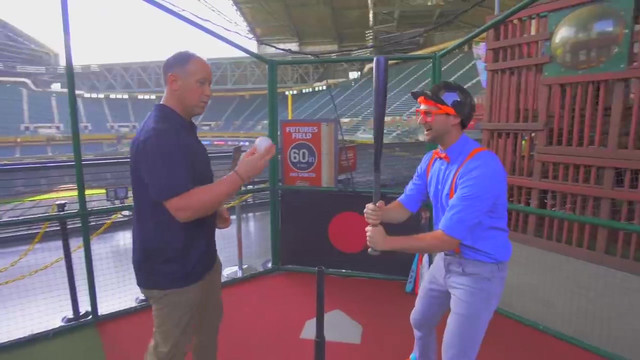 Oh, okay, a tee. Now you grip the bat. Okay, No, not that way. Blippi, Okay, This way. Oh, okay, Put your hands together. All right, And now, Yeah, Check it out. We put a ball on the tee for you to hit. 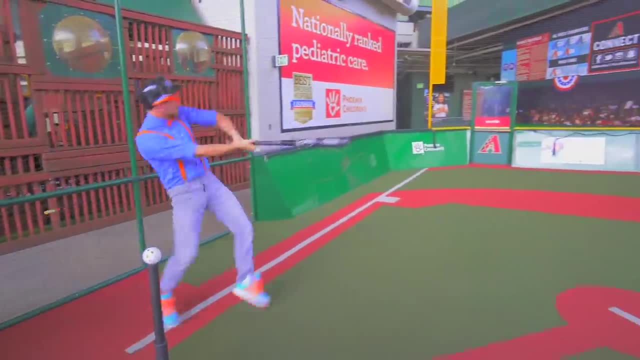 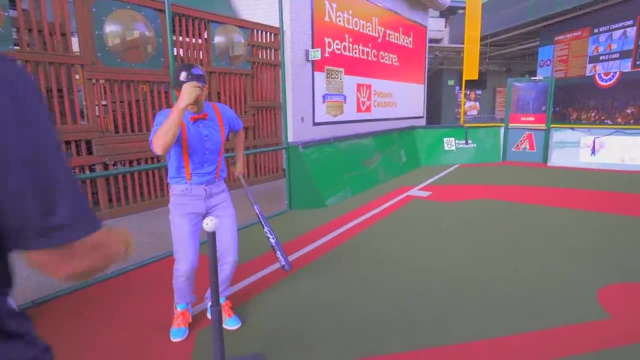 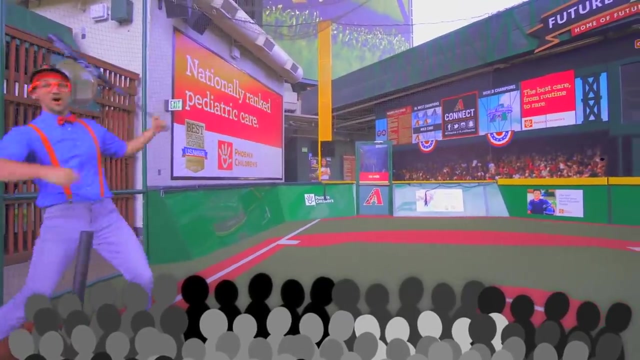 Okay, here we go. Whoa, Okay, let me try again. Put the helmet back on. Keep your eye on the ball Blippi, Okay, eye on the ball. Whoa, yeah, home run. Okay, that was so much fun. 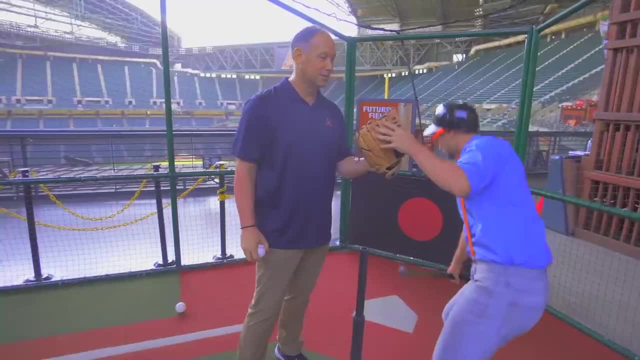 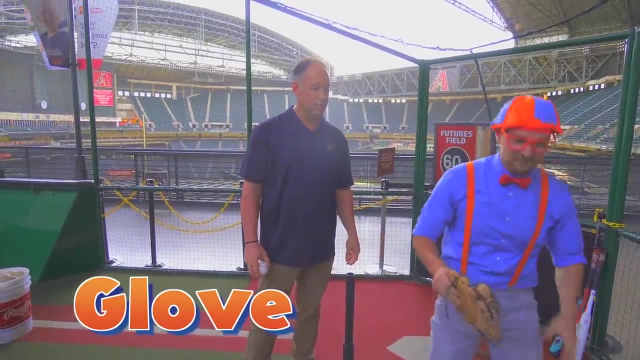 Thank you, Blippi. looks like you're ready to play catch now. Ooh, catch, Okay, all right. Oh yeah, the mitt, the glove. Okay, let's take this off and let's put this on. 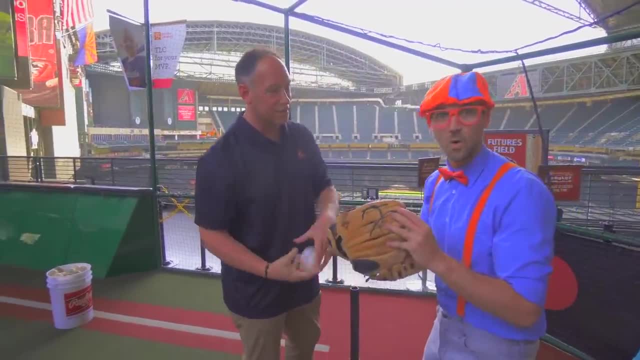 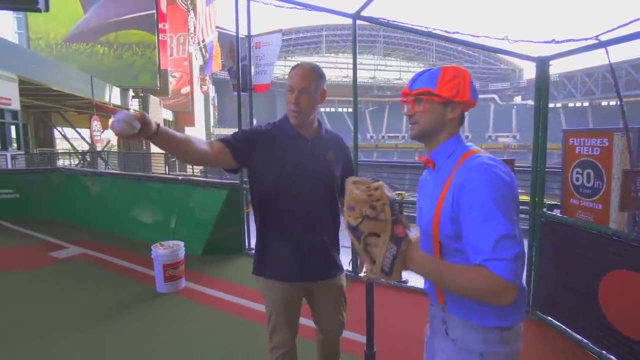 No, Blippi, the glove goes on your hand. Oh, the glove goes on my hand. oh yeah, Okay, all right, here we go. I'm ready, You ready? Yep, Okay, go out there. Okay, All right. 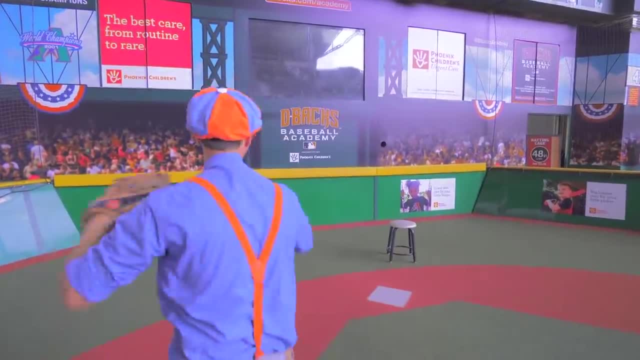 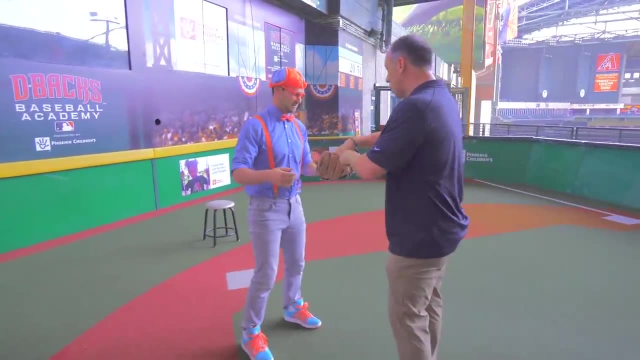 You ready, Ready? Whoa, I missed. Okay, what'd I do wrong? You have to try to catch the ball in your glove. Oh, the ball goes in the glove. Okay, all right, let's try again. You ready? 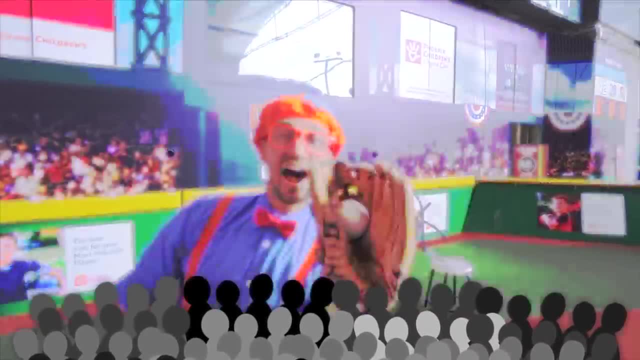 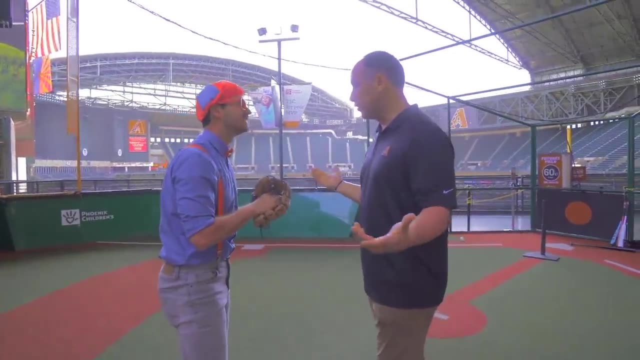 Yep, Nice. Oh yeah, I did it. Whoa, that was awesome. Thank you so much for teaching me. Blippi, looks like you're ready for the big leagues. Oh, Big leagues. What does that mean? Where do I go? 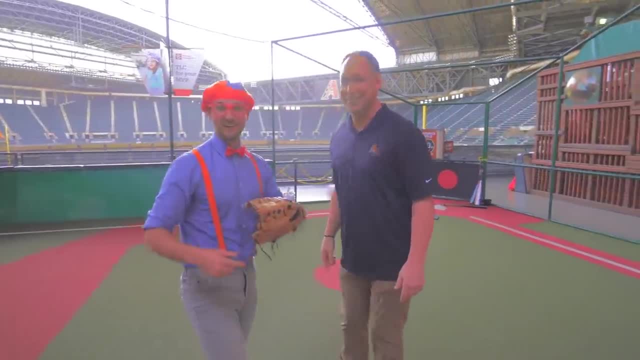 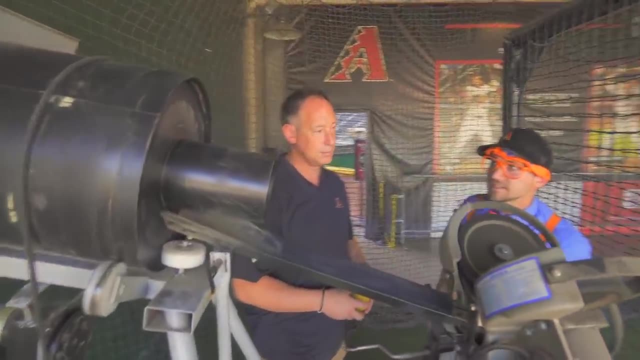 To the big field. Let's go to the cage and get ready. All right, let's go. Whoa, what is this thing? Hey, Blippi, this is the pitching machine. Ooh, the pitching machine. What does it do? 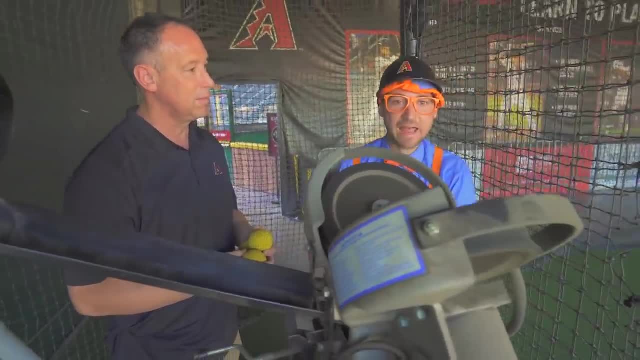 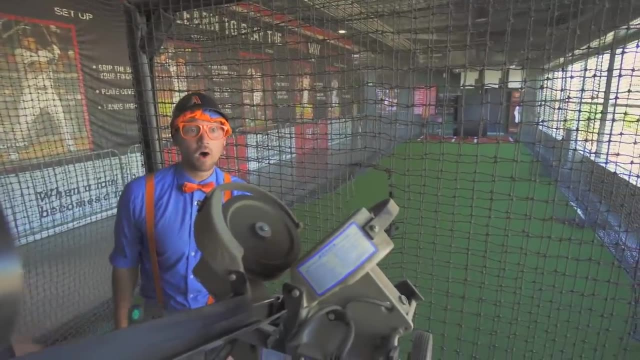 It teaches you how to bat. Ooh, teaches you how to bat. How does it work? You put the ball in the machine. Whoa, that was cool. Will you do it again? Sure, Whoa, did you see that? 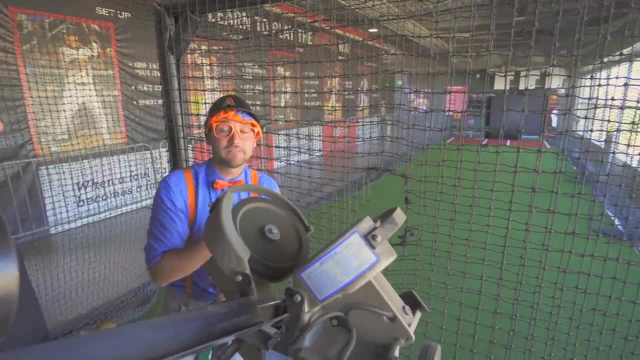 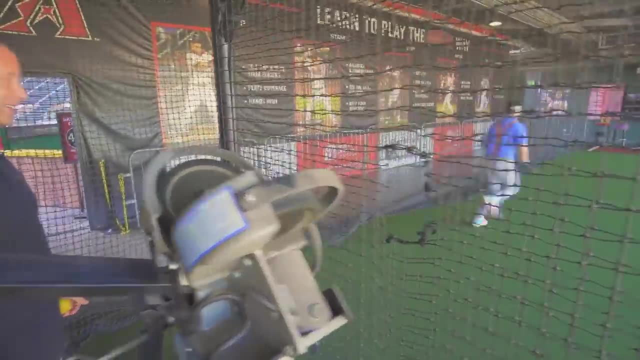 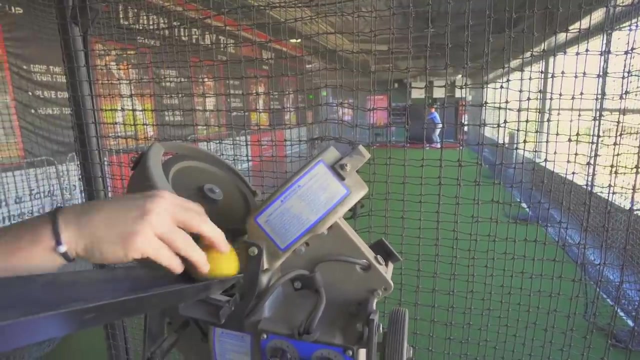 When you put the ball right here, these spinny things throw it out really fast. And then what do I do? You gotta go hit. Okay, All right, I'm ready. Okay, Blippi, here we go. Good job. 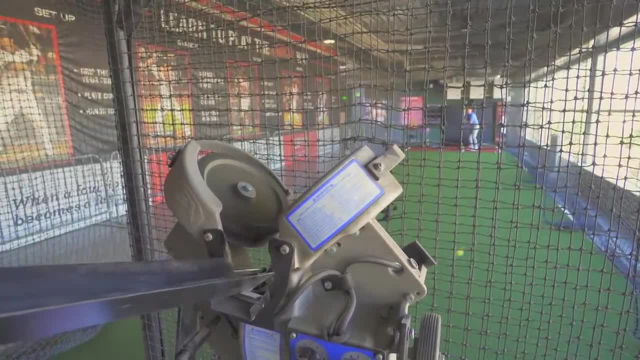 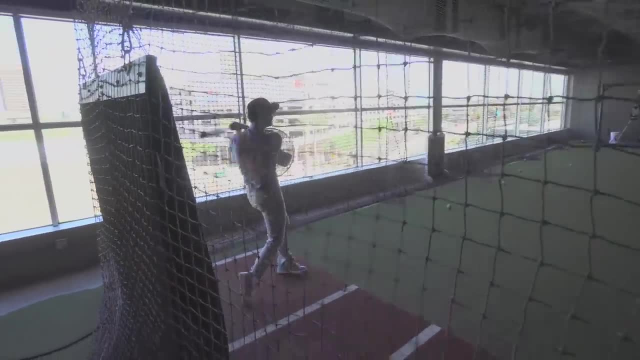 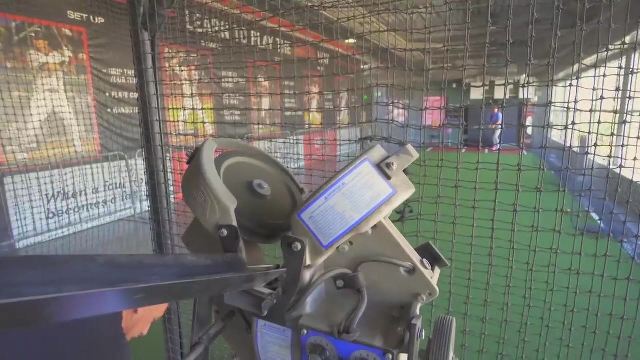 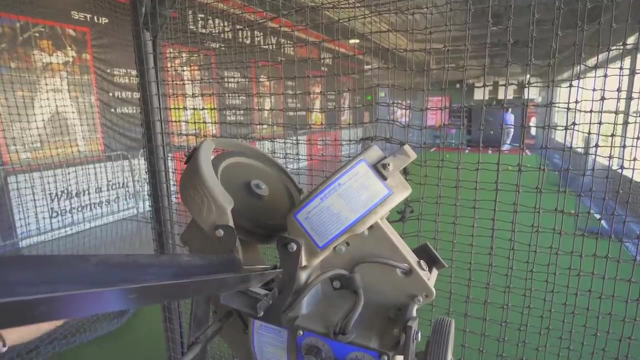 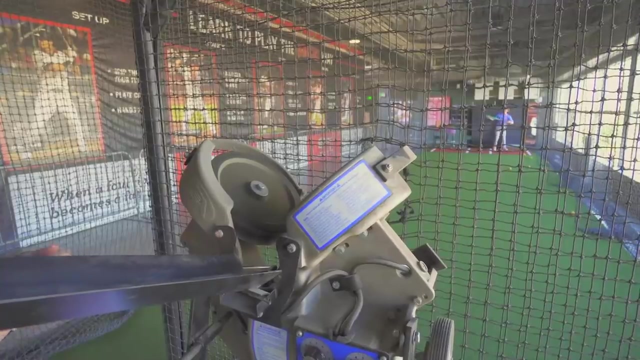 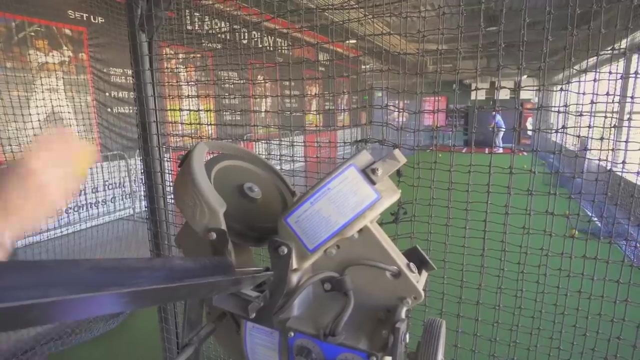 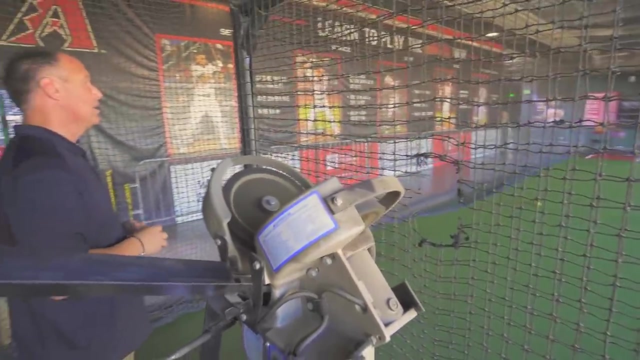 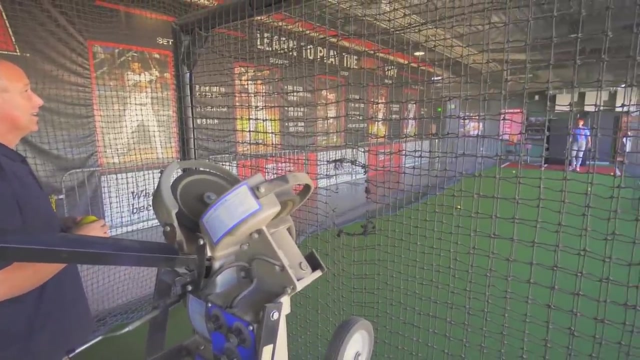 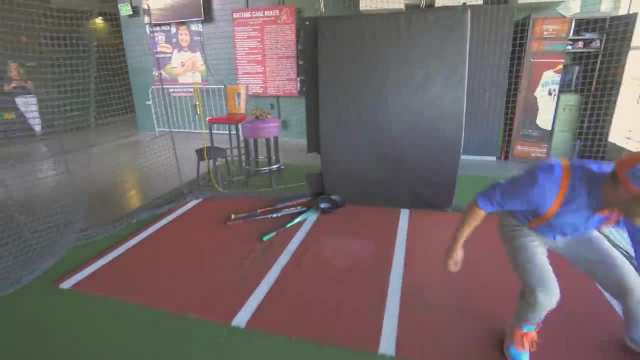 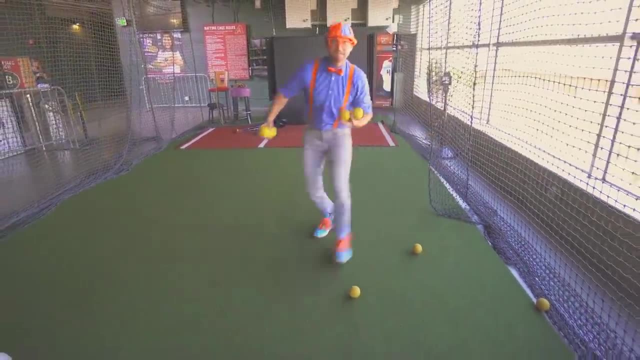 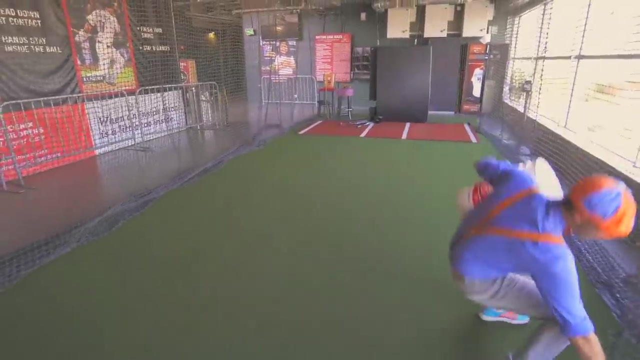 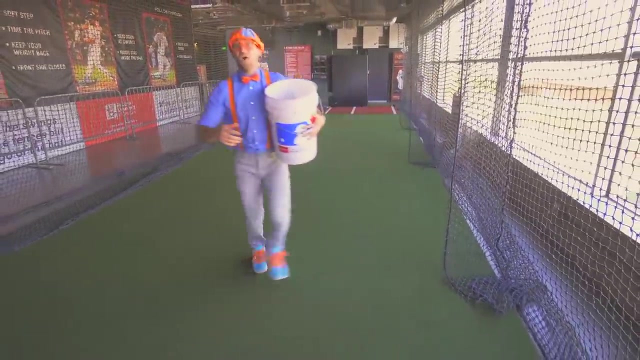 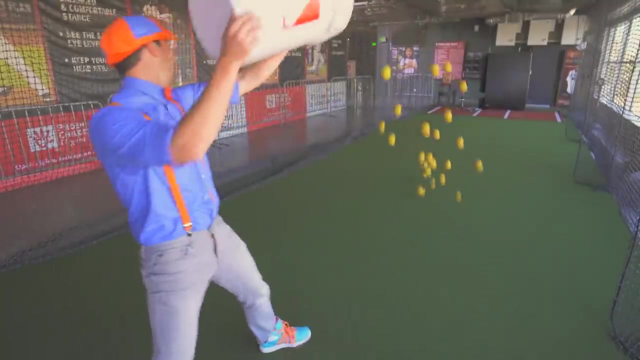 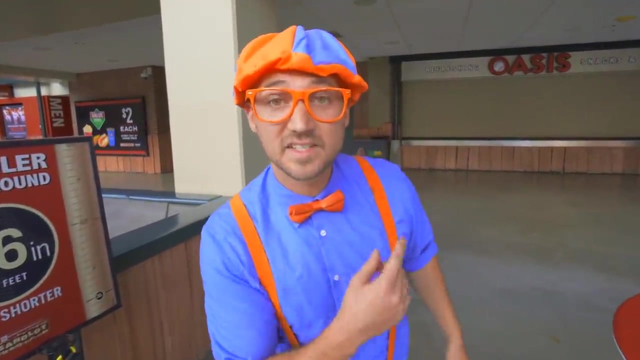 sounds fun. really important to be nice and organized and stay clean after yourself. whoa, look at all these balls. that was so much fun. I kind of want to clean up again. clean, hey, did you see that that says the Sandlot born. check it out. the Sandlot is a place where kids, just like you, can 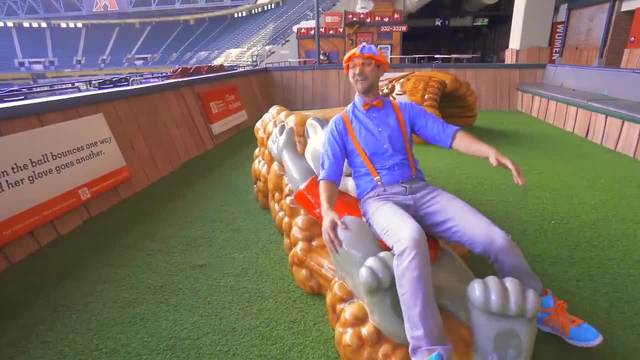 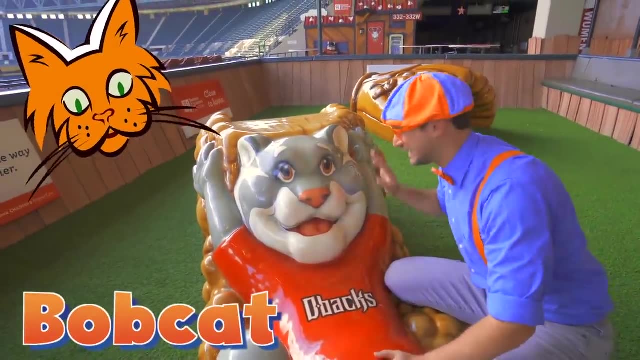 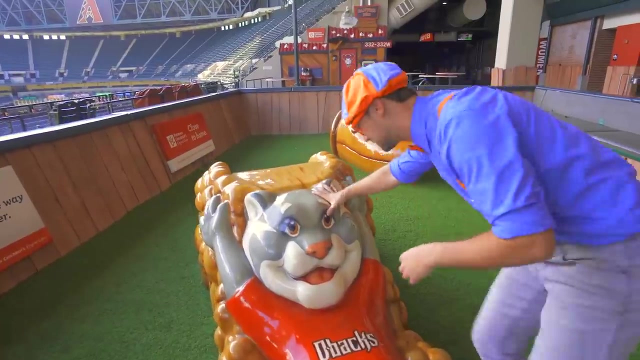 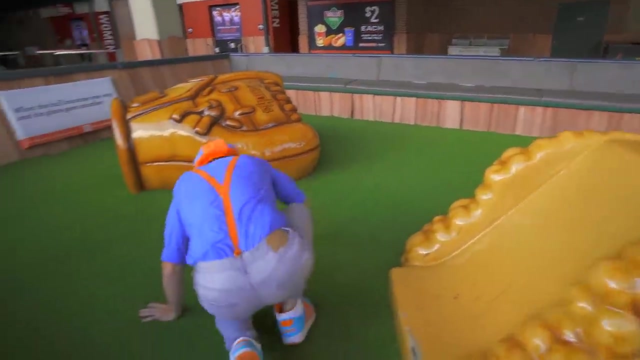 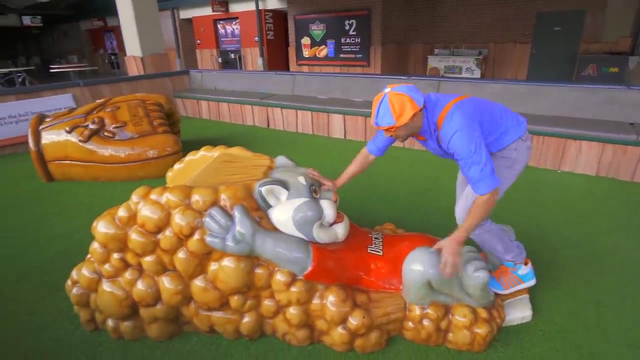 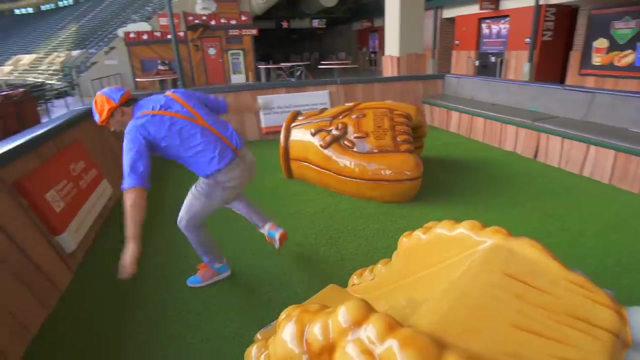 play at the Diamondbacks game. there's a Bobcat right here. hello Bobcat. yeah, Oh, and it's a slide. check it out. whoa, all right, here we go. whoa, oh, that was fun, I want to do it again. whoa, all right, here we go. this is cool. here we go. 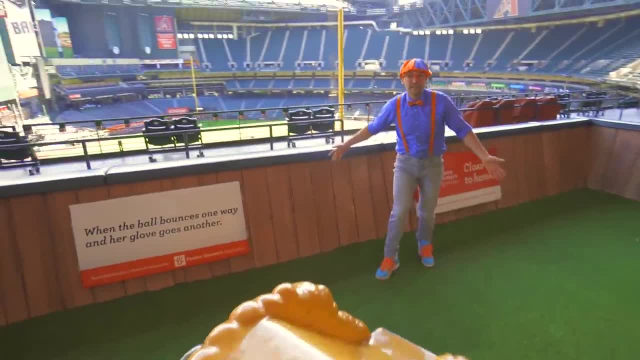 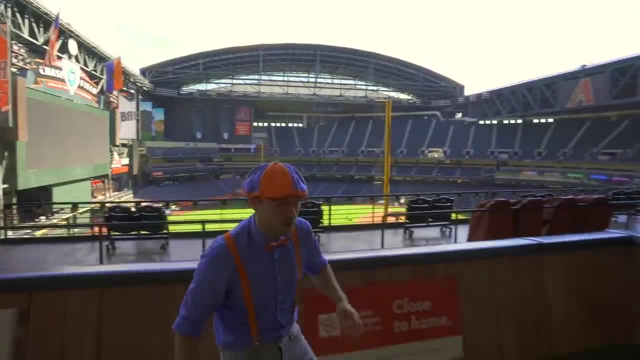 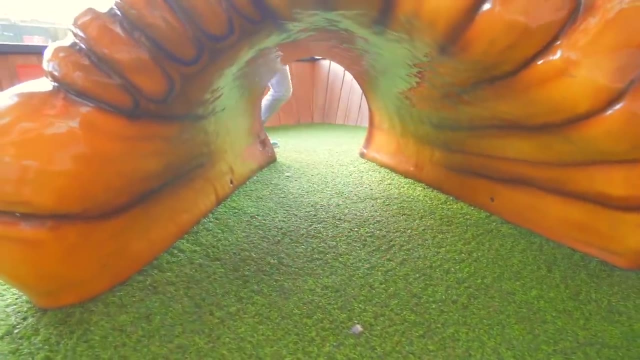 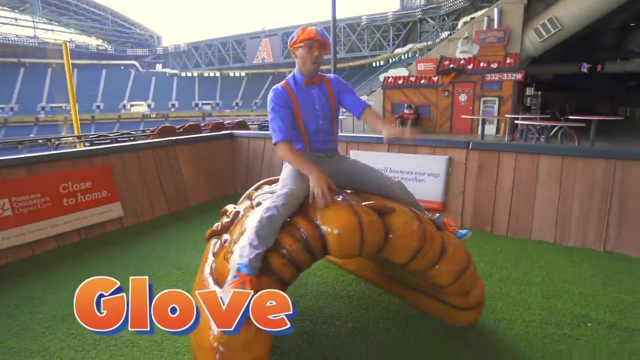 Oh, and look, while playing, you can even watch the baseball game. hello, hello down there. oh, that's awesome. whoa, what is this? whoa, hello, hey, what are you doing down there? look, it's a baseball man. yeah, a glove, I got the ball. I'm gonna. 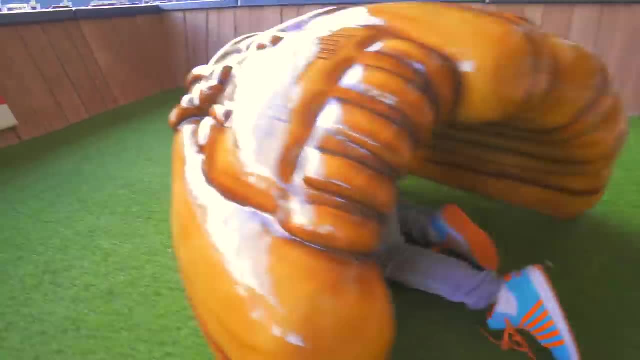 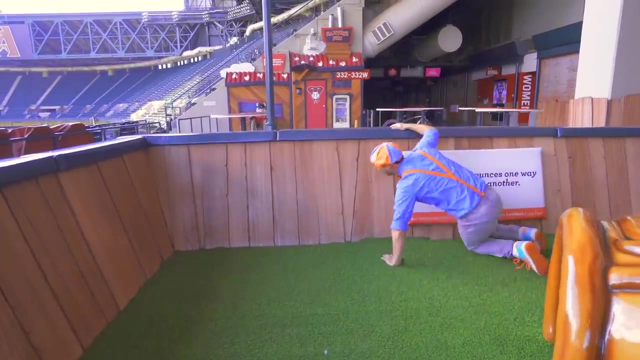 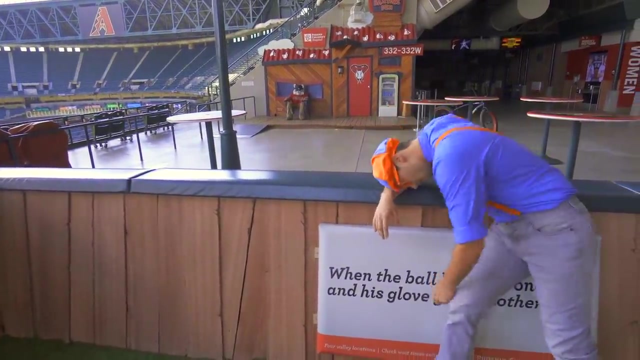 crawl through now you hello, hello, hey. this is so much fun. I am getting so tired with all this playing. oh, do you see what I see? come here, look, there's a Bobcat over there. let's go meet it. whoa, I am so excited. a real Bobcat. 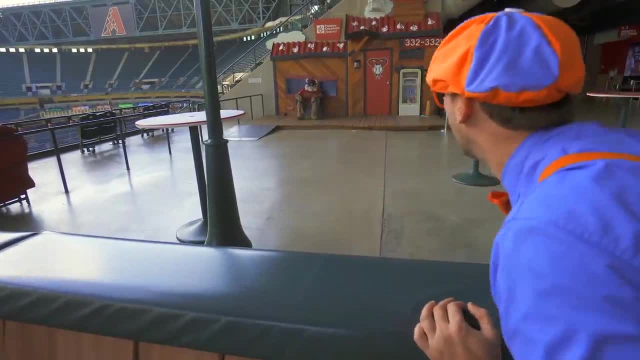 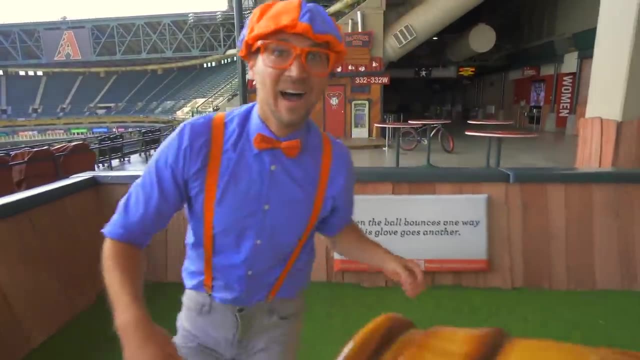 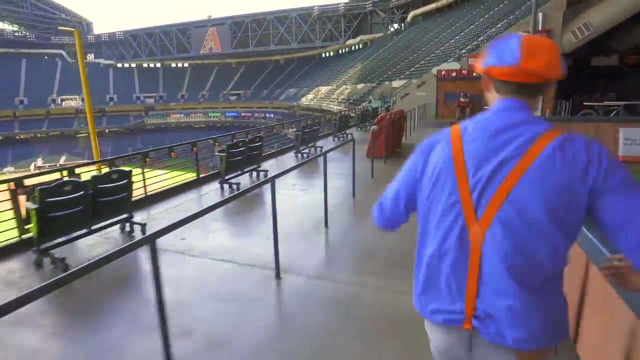 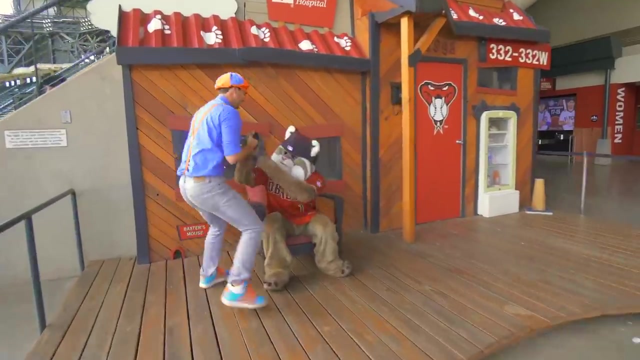 come here. look, there's a Bobcat over there. let's go meet it. I am so excited. a real Bobcat. hello, Come on. Whoa, Whoa, Look, Hey, How are you? I want a hug. Whoa, This is Baxter And Baxter. 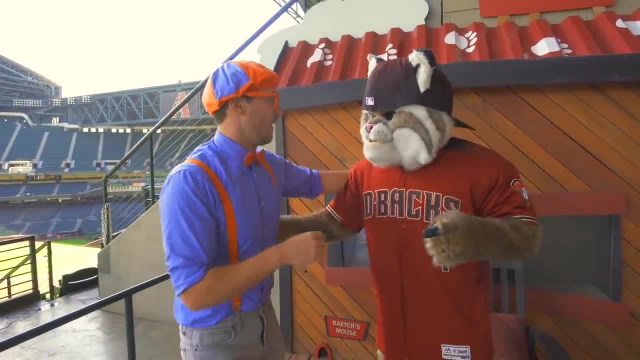 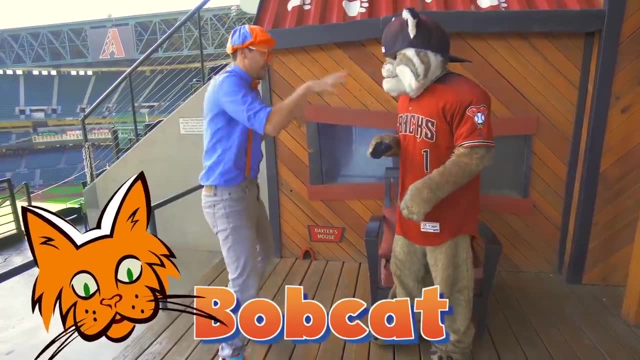 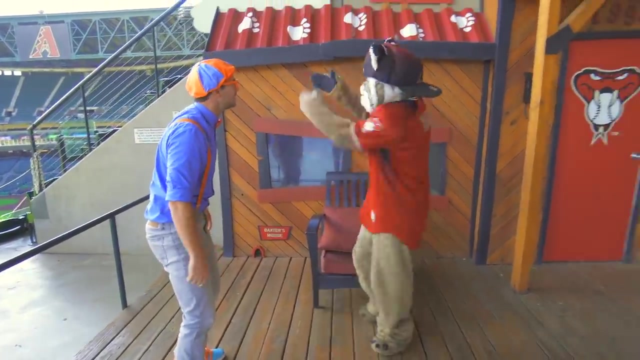 is the mascot for the Diamondbacks? Whoa, And what are you? Oh, This is a bobcat. Are you a bobcat? Oh, Meow, Oh, Is this your house, Baxter? Whoa, It's really cool. Check. 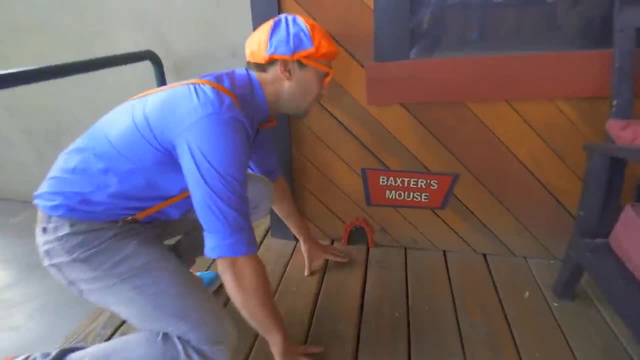 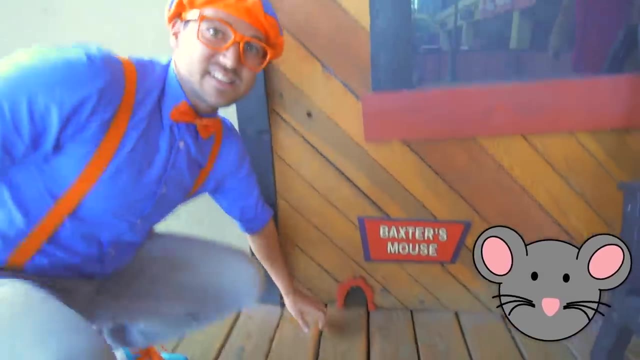 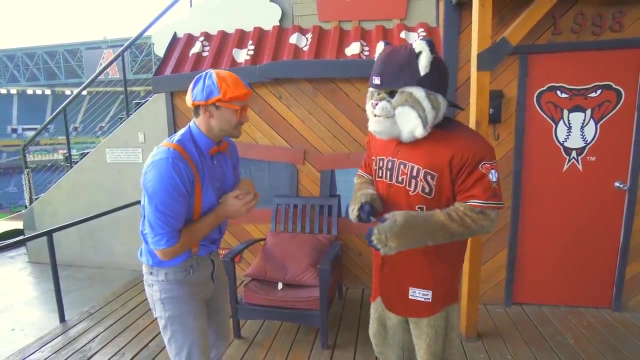 it out. Whoa, What's this? Oh, It's Baxter's mouse. Hello, How are you? Oh, I guess it's not here right now. Oh, Is the mouse your pet? Oh, That's a good one. Oh, It's a. 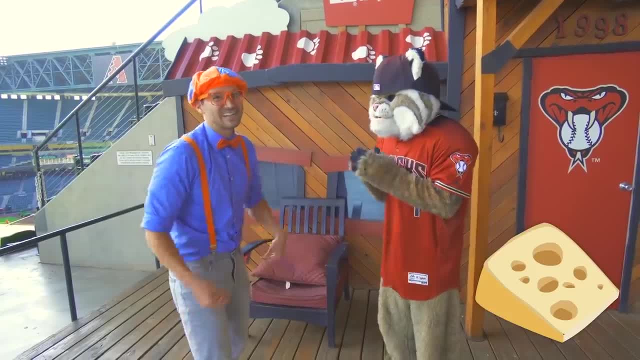 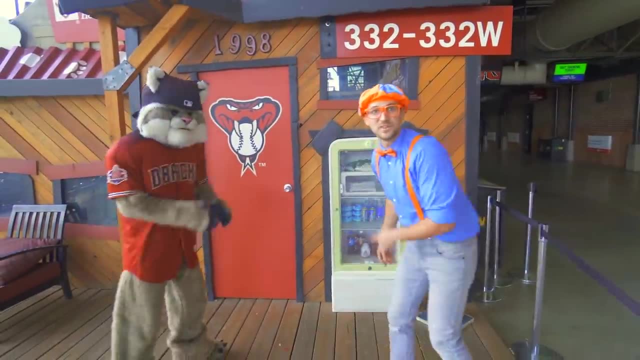 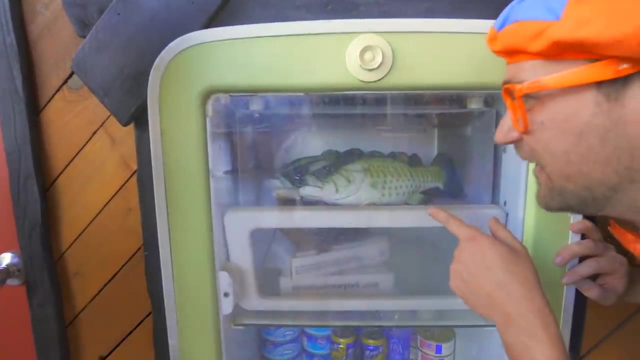 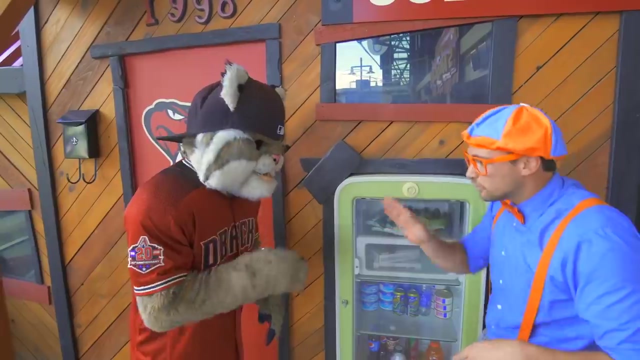 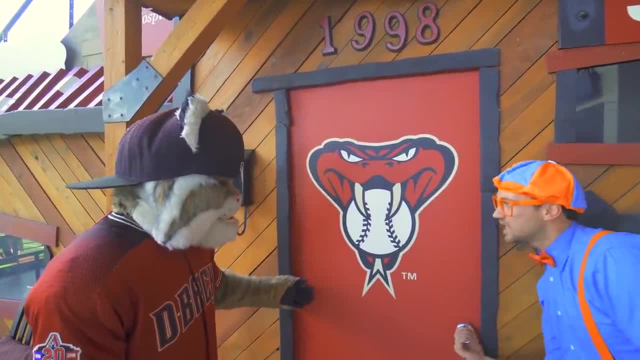 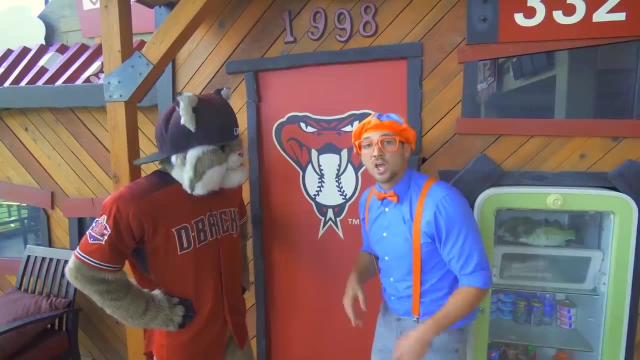 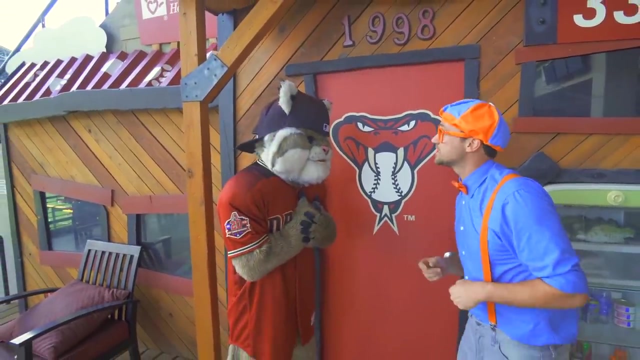 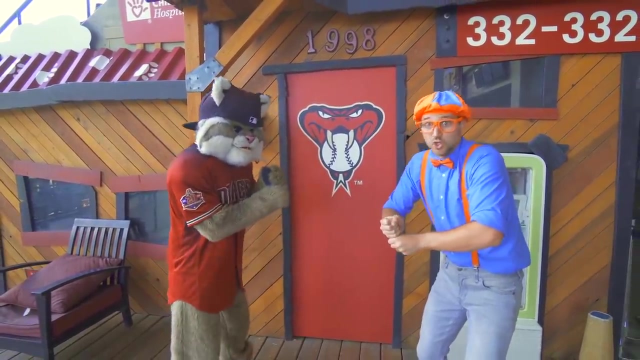 a door right here. Ooh, Does this go inside to your house? Whoa, Pretty cool. Oh, It's locked. Hey, Let me ask you a question: Do you like to dance? Awesome, Can I teach you the baseball dance? Okay, All right. So you act like you grab a bat, okay, And then you. 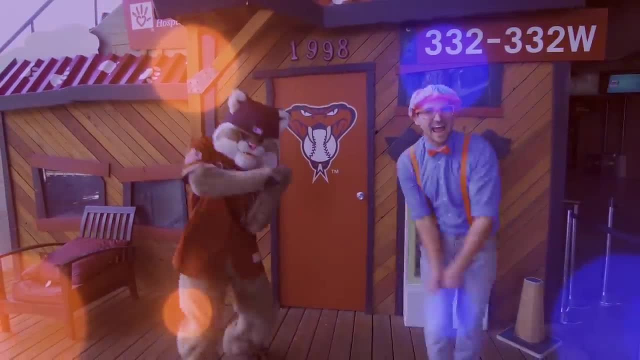 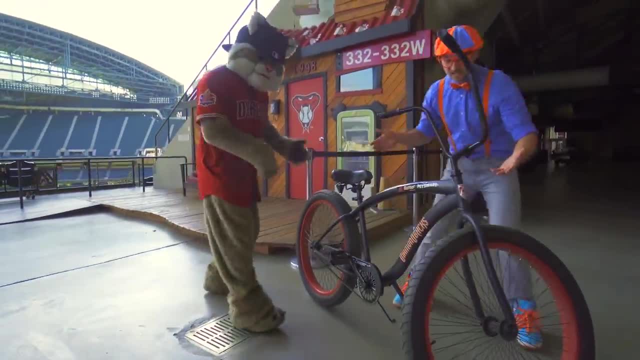 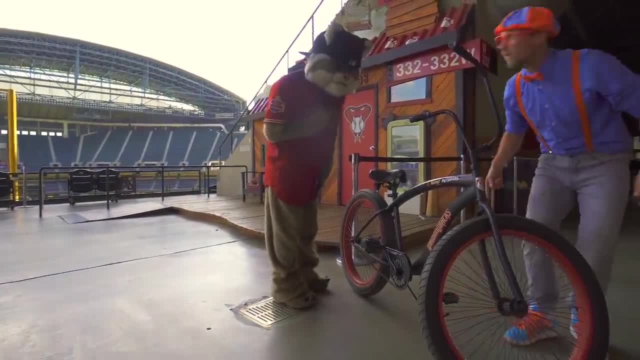 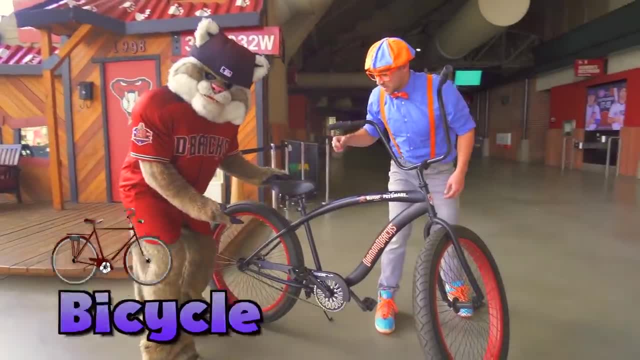 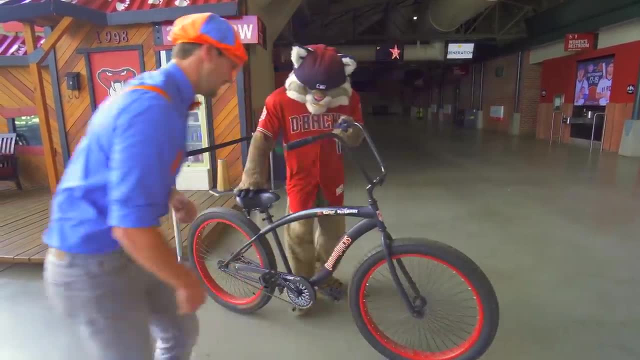 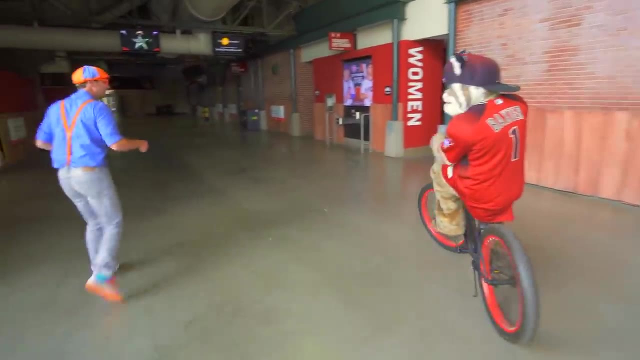 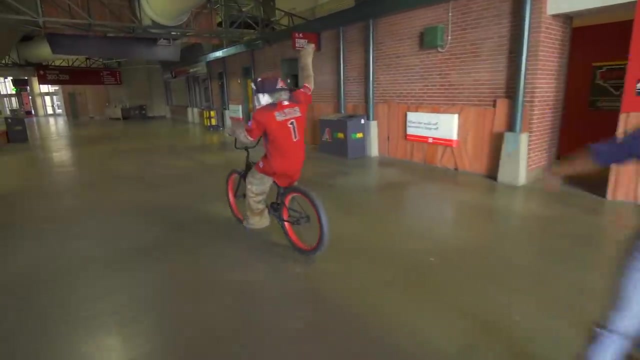 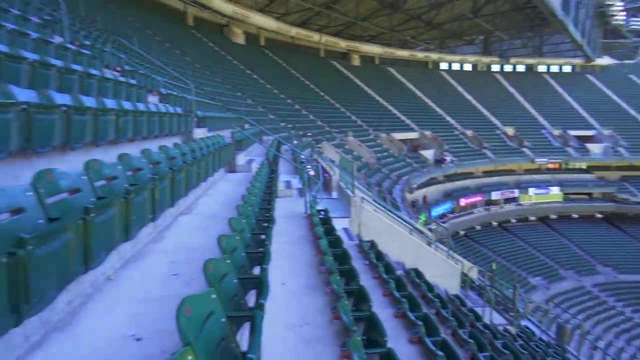 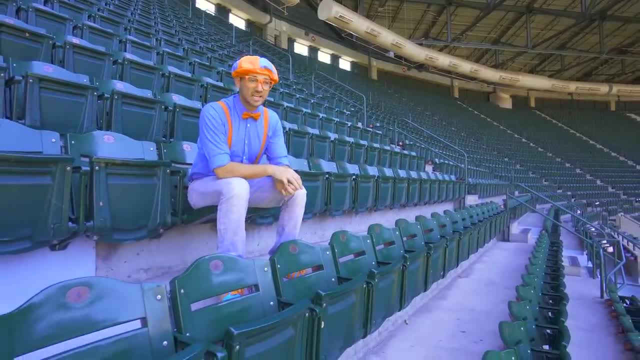 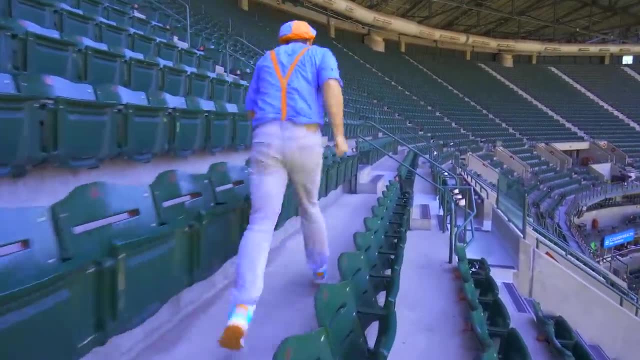 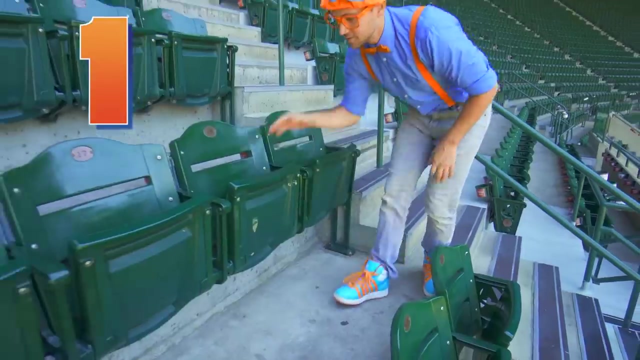 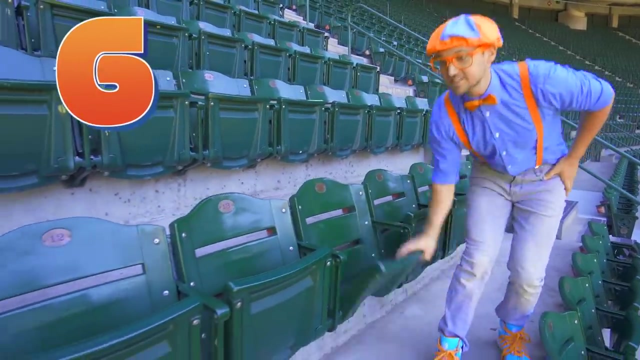 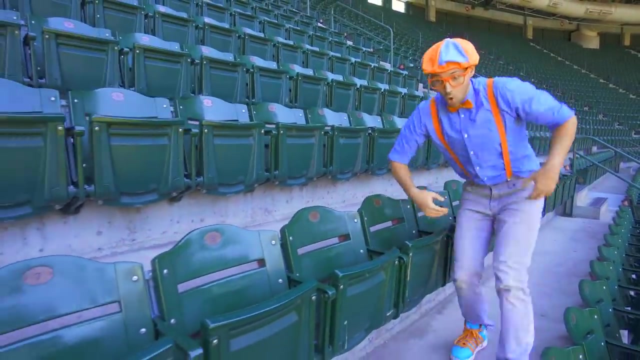 Whoa, there's so many seats in this stadium. Hey, I have an idea. Why don't we count them? Okay, let's start down here. Okay, let's count this way. row of seats Ready: One, two, three, four, five, six, seven, eight, nine, ten, eleven, twelve. 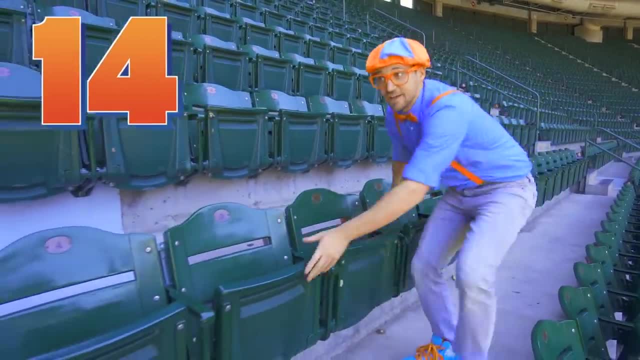 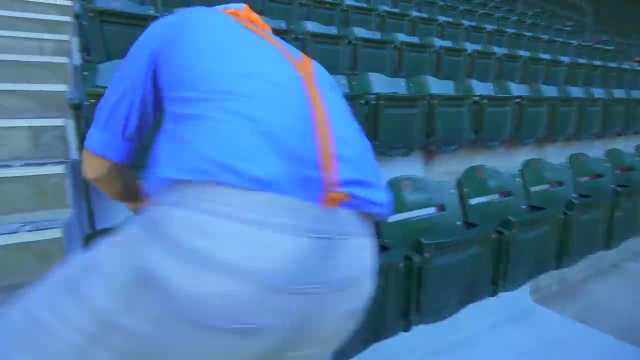 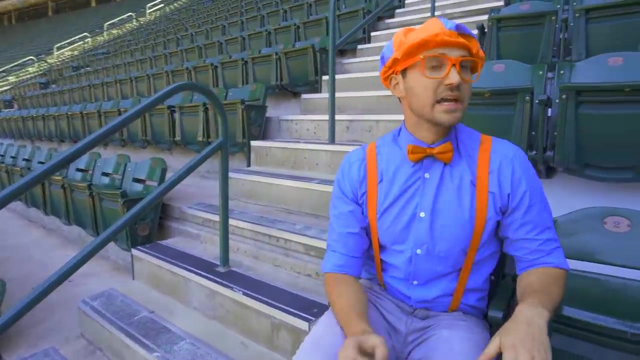 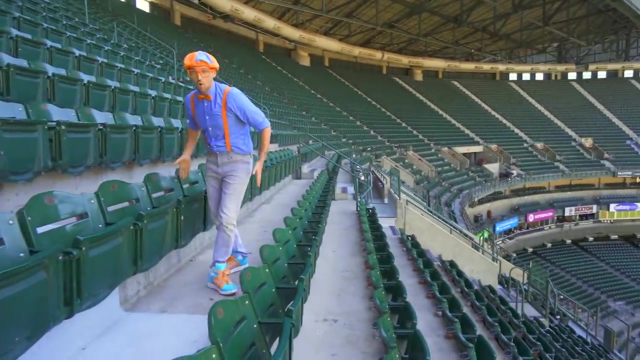 thirteen, fourteen, fifteen, sixteen, seventeen, eighteen and nineteen. Whoa, that's a lot of seats in this row. Okay, to find the total number of seats in this whole stadium, you just take this row and multiply it by the total amount of rows, Okay. 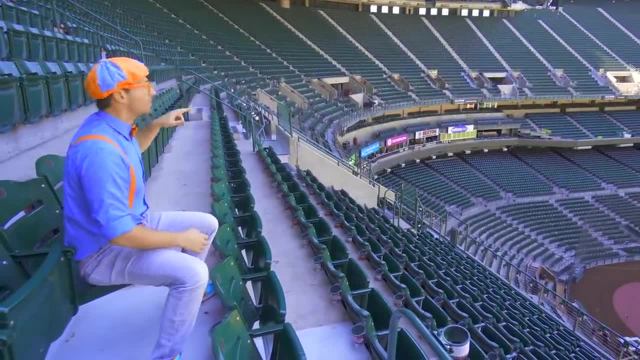 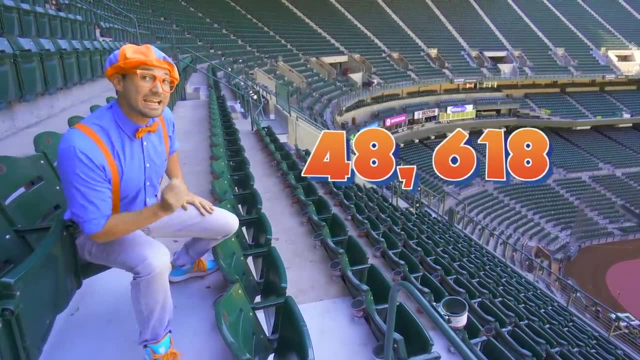 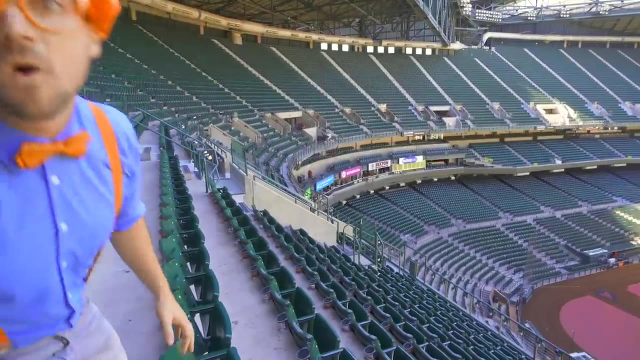 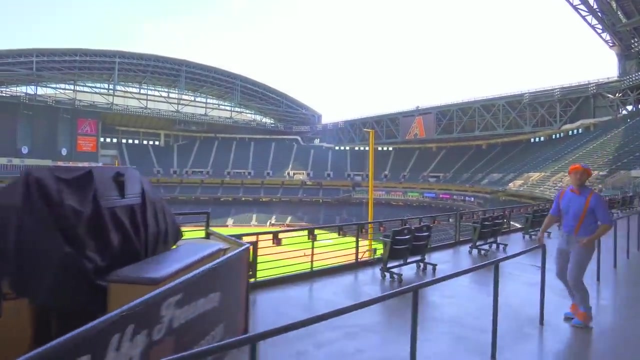 Let's see Whoa. Okay, it looks like there's 48,618 seats in this stadium. Yep, that's right. That's a lot of seats. Whoa, Whoa, Baseball fields are so cool. Whoa, come here. That's. 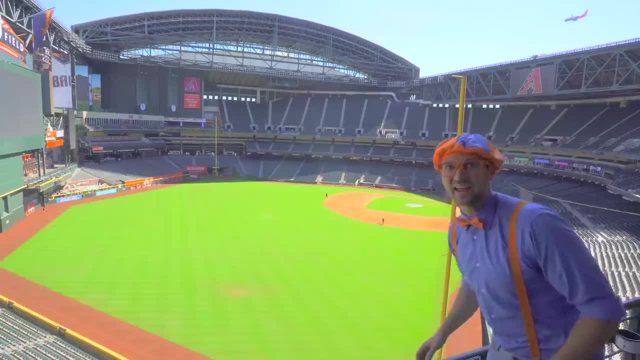 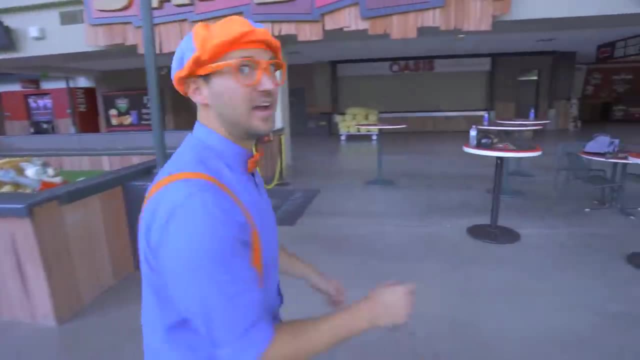 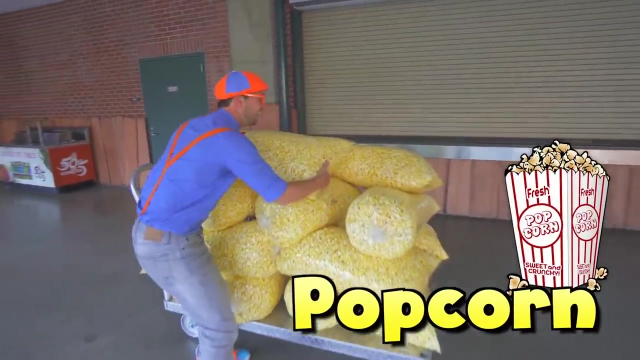 a lot of grass, Whoa, Hey. do you know one food that every baseball game has? I'll show you. Yeah, it's over here, Whoa, Yeah, popcorn, Whoa. Look at all of this popcorn. Whoa, Okay, let's. 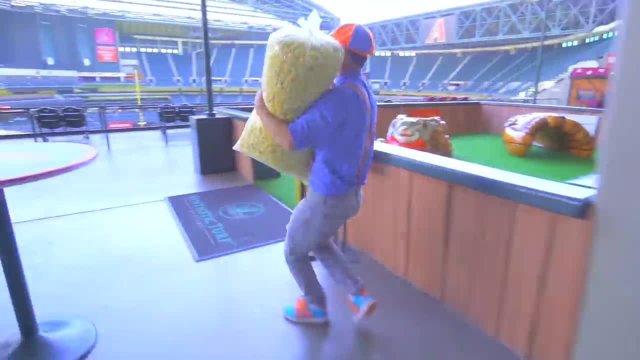 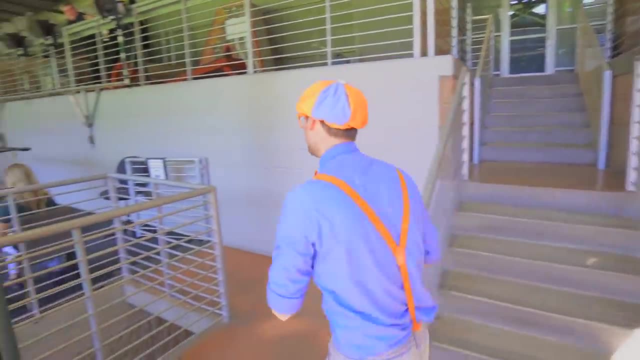 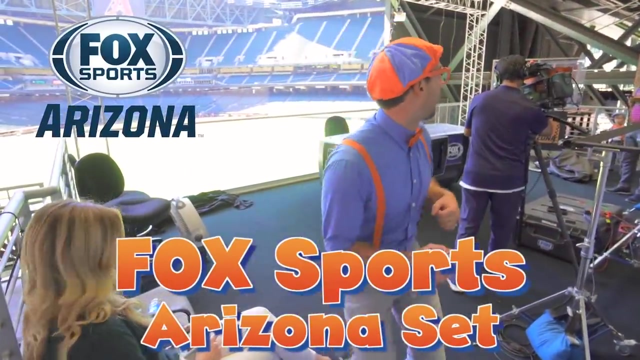 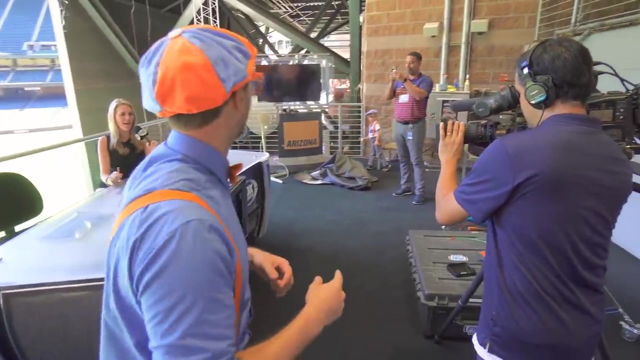 go enjoy the game. Whoa. Hey, I have another thing to show you. Come over here, Whoa. This is the Fox Sports Arizona set. Whoa, So cool. This is where they do their show, Ed. Oh, look a camera. Hey, come. 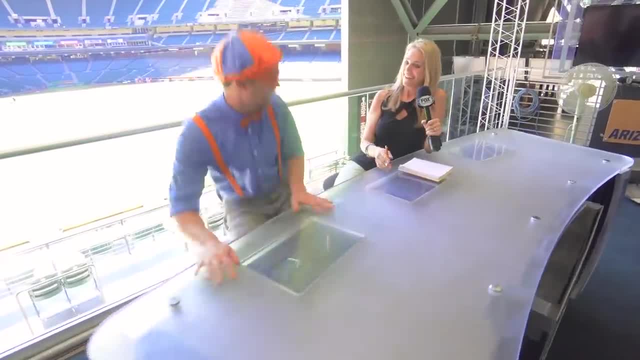 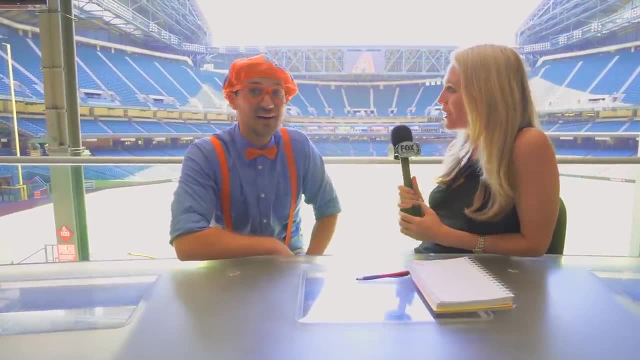 over here. Whoa, Hey, Hi there. What's your name? My name's Kate Longworth. Nice to meet you. Nice to meet you too. So what do you do? I'm a reporter. I go down and talk to. 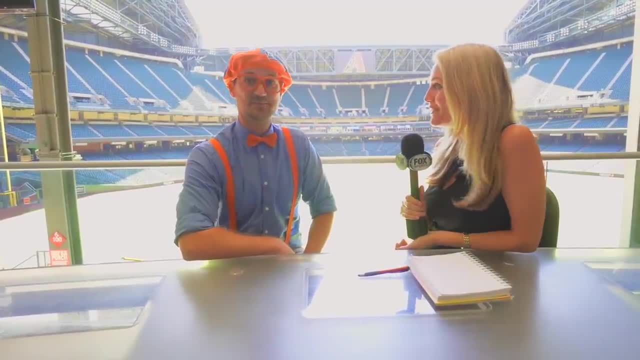 the baseball team. I go down and talk to the baseball team. I go down and talk to the baseball players and then put it on TV so folks at home can see what they're doing. Whoa, What's that thing? This is a microphone. When I talk in here, it helps people at home. 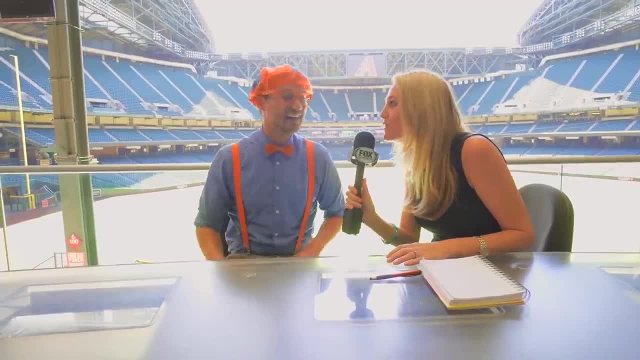 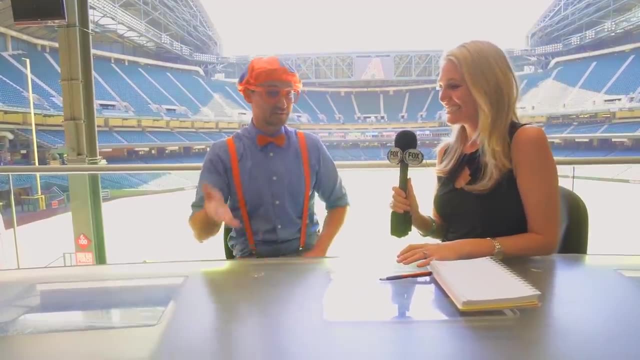 hear me? Oh, hello, Can you hear me? Even when you whisper, they can hear you. Hello, Can you hear me? Oh, that's silly, Well cool. Thanks for showing me your spot. Yeah, Anytime. 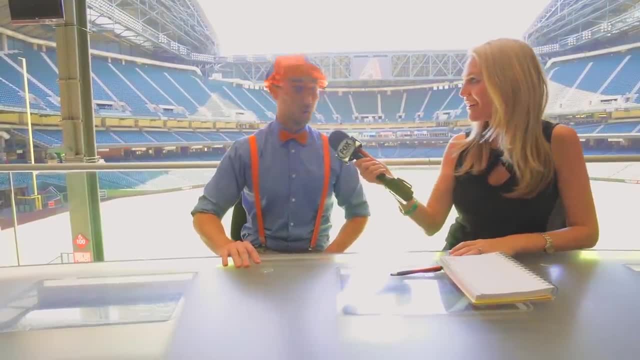 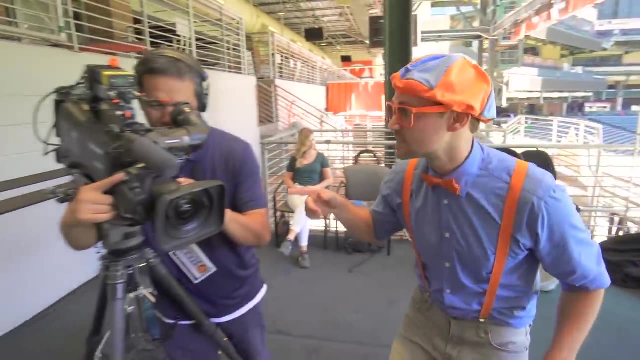 Stop by our desk and I'll send you down to interview some players. Oh cool, Hi Hi Mom, Okay Here, come over here. Whoa, Look at this, A giant camera. Hey, what's your name? My name's Rusty. What do? 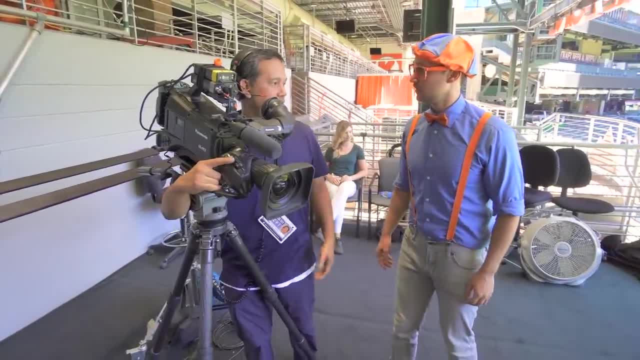 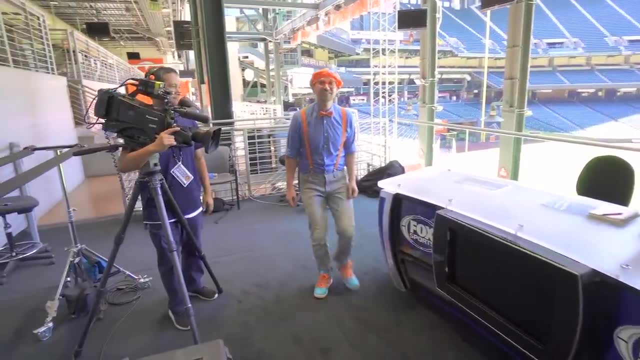 you do. I'm a cameraman, I take videos of Kate and I take videos of the players when they're playing. Oh really, Here's a little tip: Be really nice to them, because they'll make you look good. Oh, did you hear that? That's silly, Well, cool. Thanks for showing. 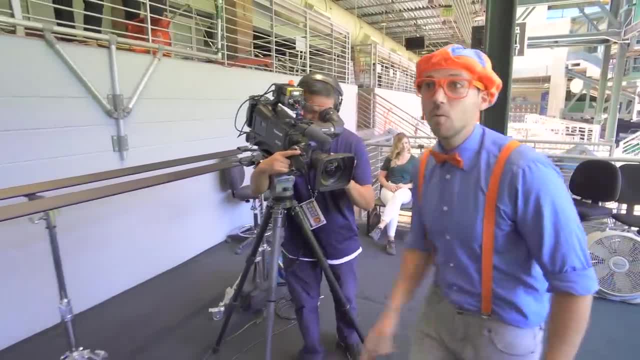 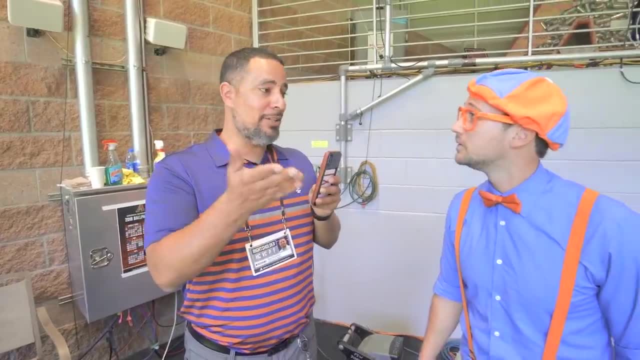 us your really cool camera, Rusty, Anytime, All right. Whoa, Here's another person. Whoa, Hello, Hey, What do you do? I'm in charge of our social media network, so everything they do on TV we try to put on Facebook, Twitter. 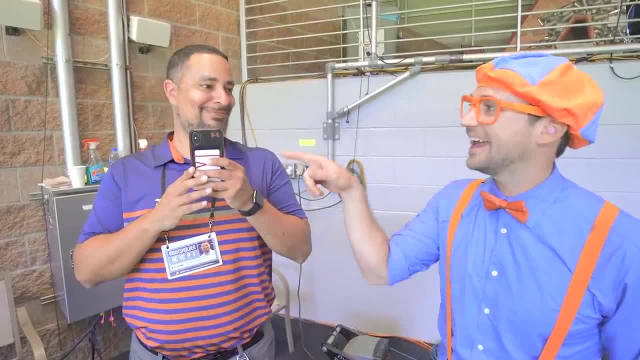 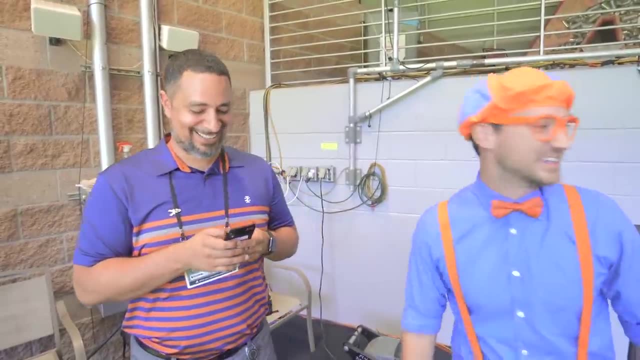 YouTube and Instagram. Whoa, That's really cool. Hey look, He's on his phone on the job. That's a no-no unless you're him All right. Nice to meet you. Oh look, There's. 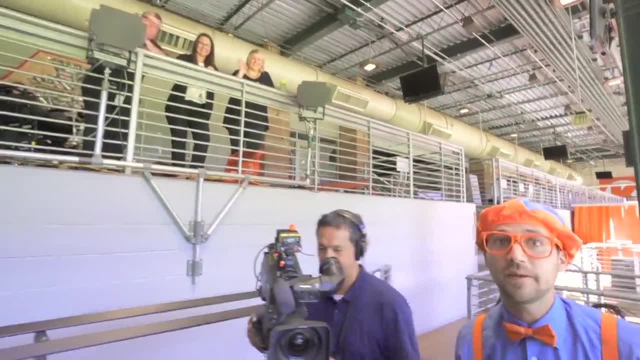 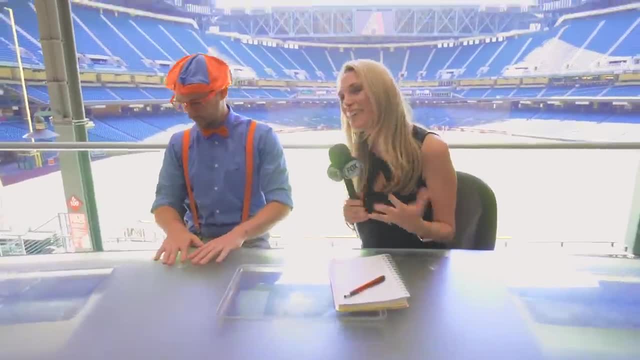 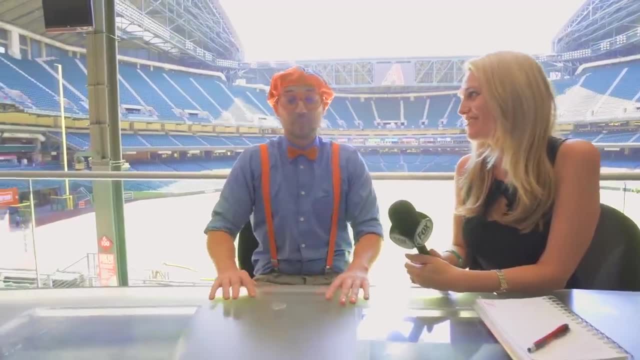 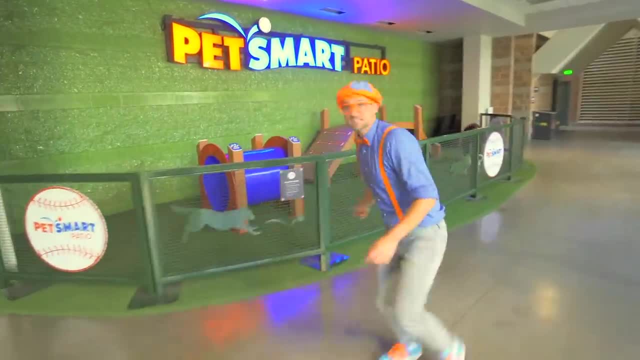 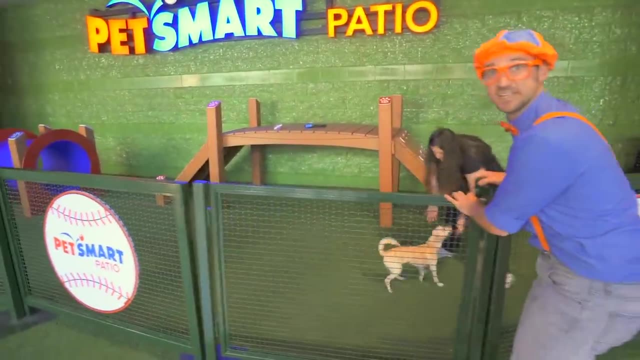 Whoa, check it out. It's like a miniature dog park here. Chase Field even has a place for dogs. Hey, you want to come in and meet Sadie Whoa, Come on in, Whoa. Hey Are you? 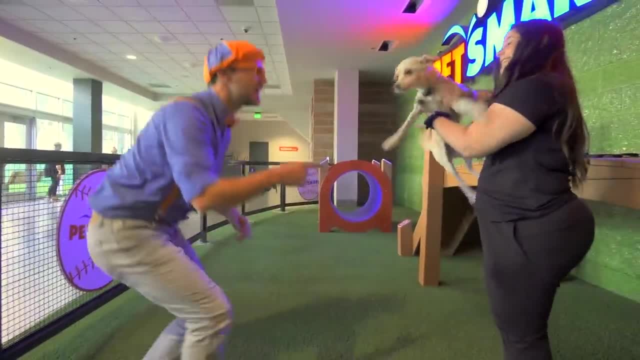 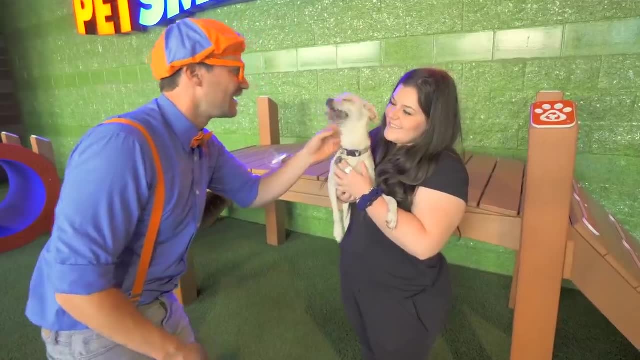 Sadie, Hi, Sadie, Whoa. Did you see how high Sadie jumped? Hey, Sadie, I'm hired. Whoa Blippi, how are you? Are you having fun? Yeah, What's your name? 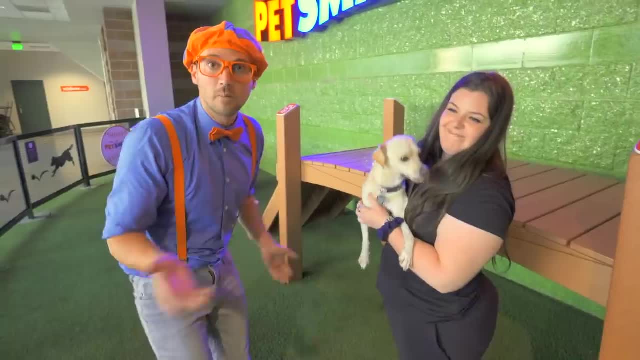 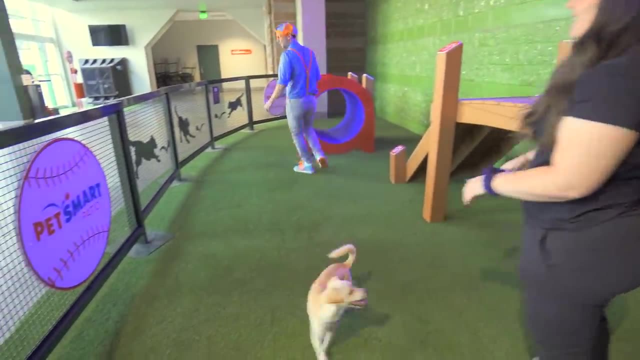 Sarah. Ooh, this is Sarah and Sadie. Both of them start with the letter S. Okay, let's see you run around, Sadie. Okay, Whoa, Whoa, Whoa. That's a really big jump. 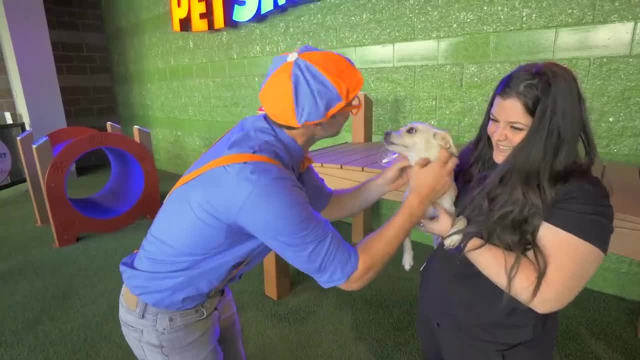 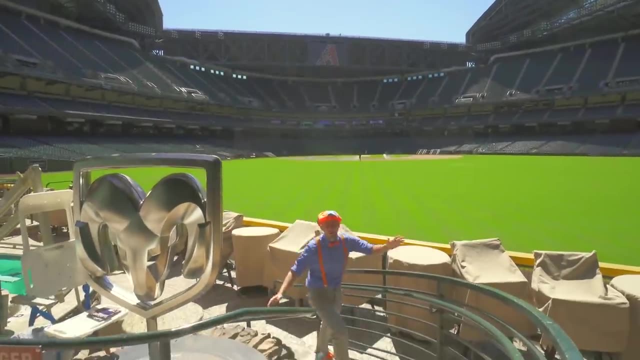 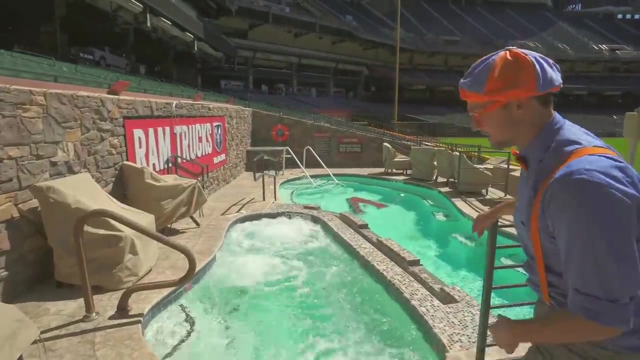 Whoa, good job, Sadie, Yeah, Yeah, Yay, Oh yes, Can I say hello, Whoa Hello. Baseball is so cool. Ooh, and this is really cool. This stadium even has a pool over there and a hot tub. 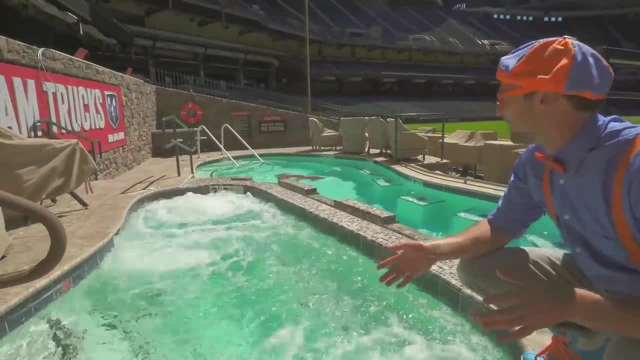 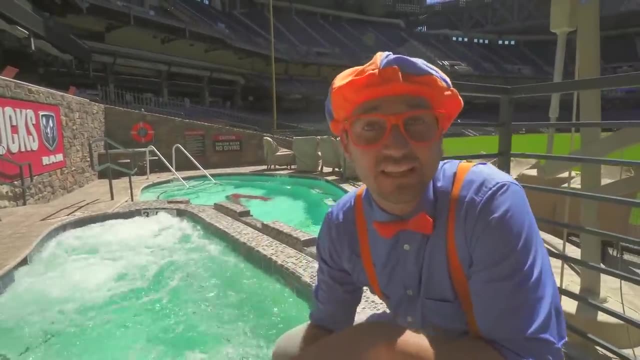 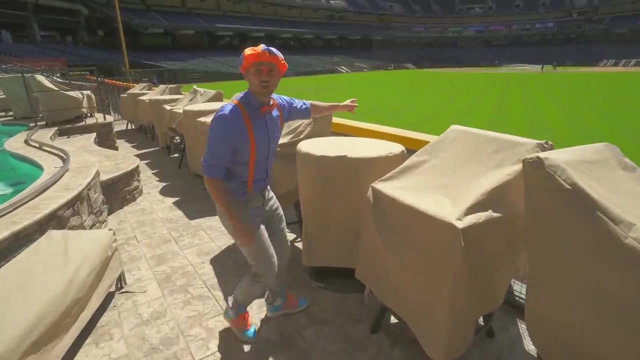 Whoa, You can sit in these and watch the game. Whoa, it is so hot here in Arizona. Hey, let's put our feet in the pool and cool down. Whoa, Whoa, Yay, Whoa, check it out. 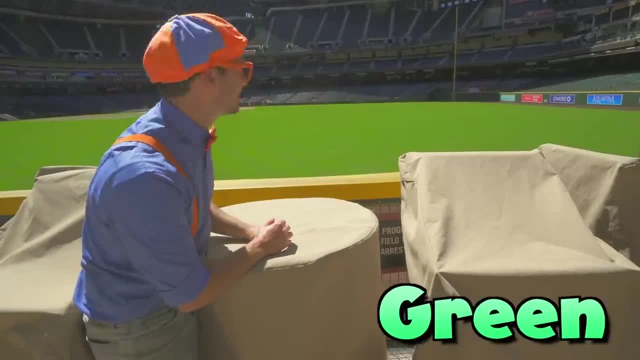 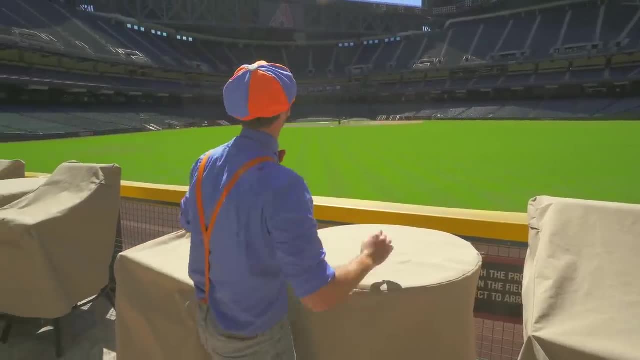 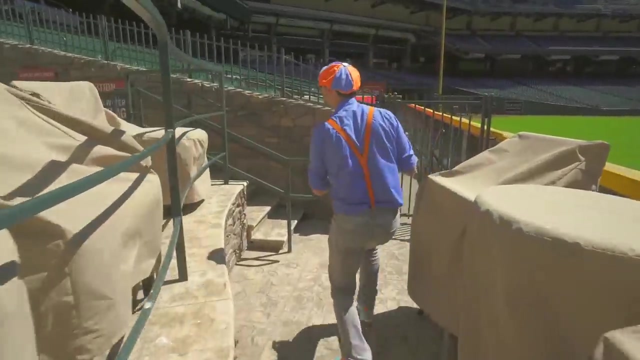 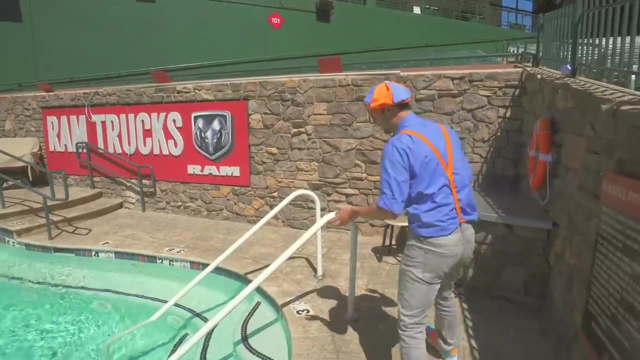 Look at the field, Look at how green the grass is. Oh, and there's people out there watering the grass. Hello, Whoa, Okay, follow me. Whoa, I am so excited, I am so warm. This is going to feel so good. 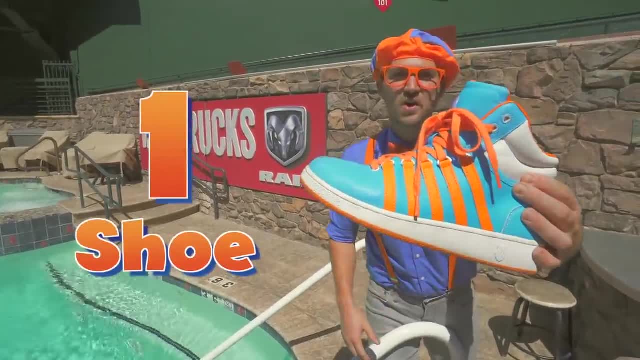 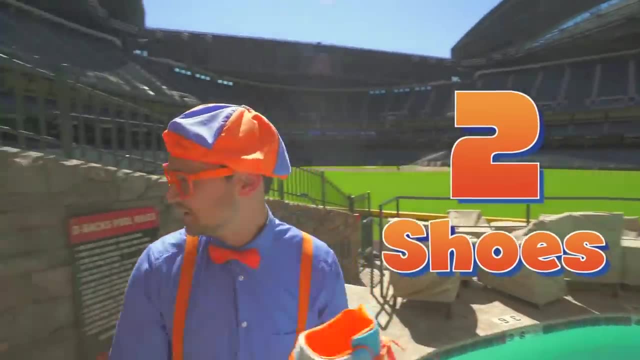 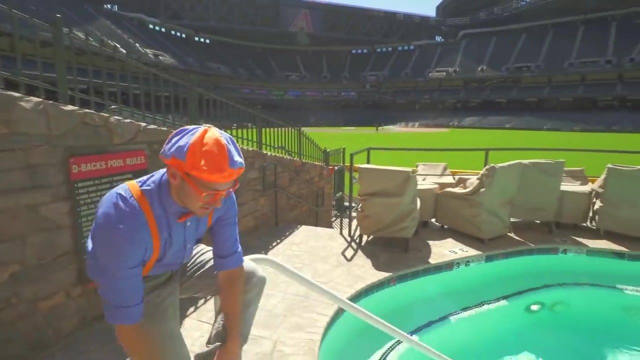 Okay, First let's take off our shoes. One shoe, And here is the second shoe, Check it out. One, two, because I have two feet, All right, Okay. Oh, one stinky sock, Two stinky socks. 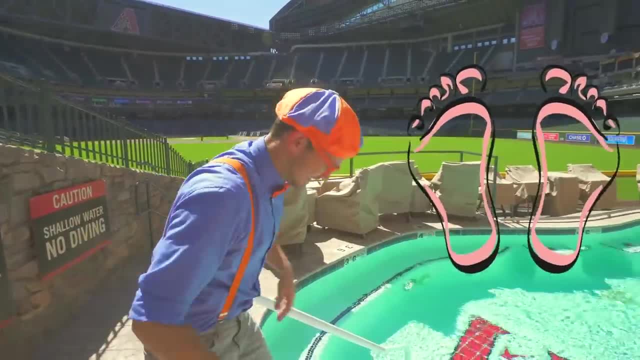 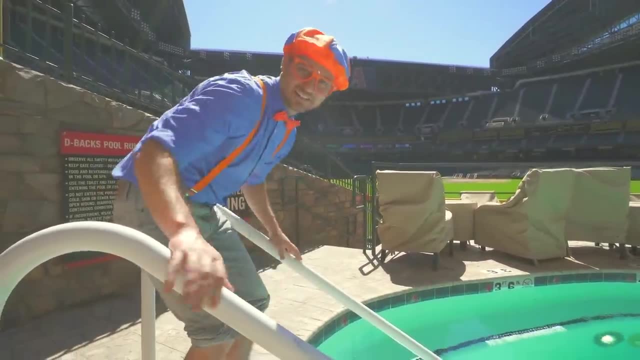 Oh, because I have two stinky feet. All right, Let's roll up my pants, Perfect Okay. Now let's take a dip. Oh yes, Oh yeah, This feels so good. Oh, I hope someone hits a home run. 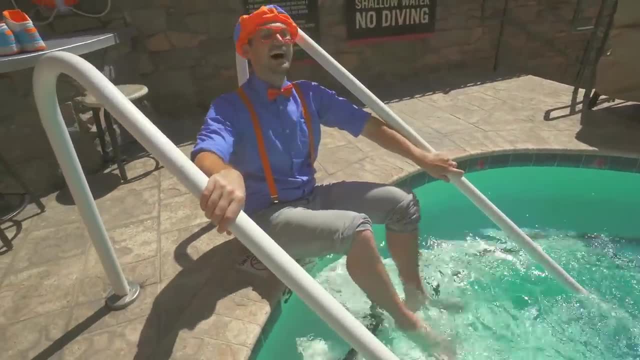 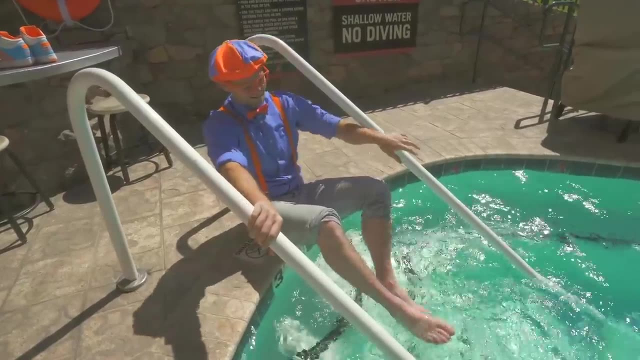 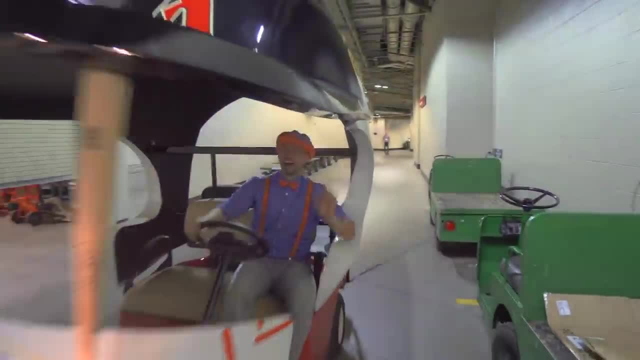 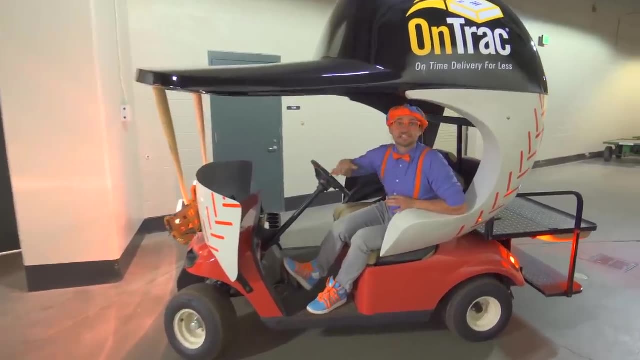 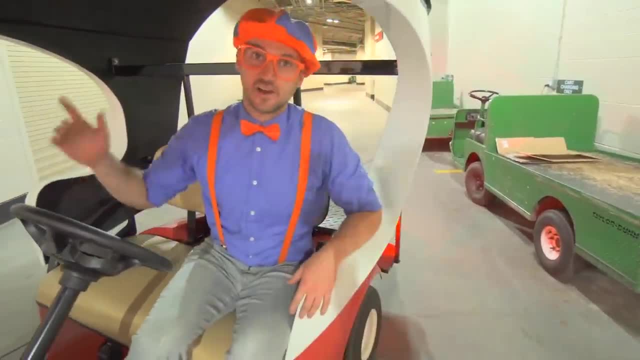 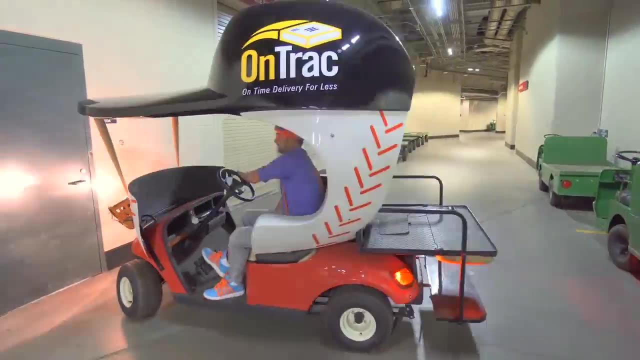 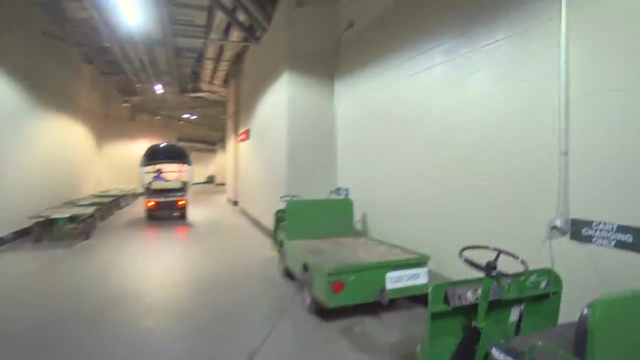 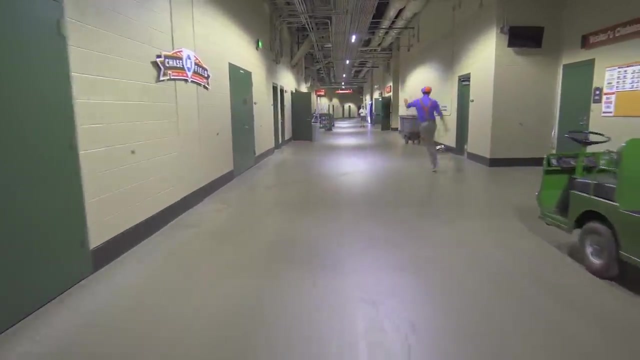 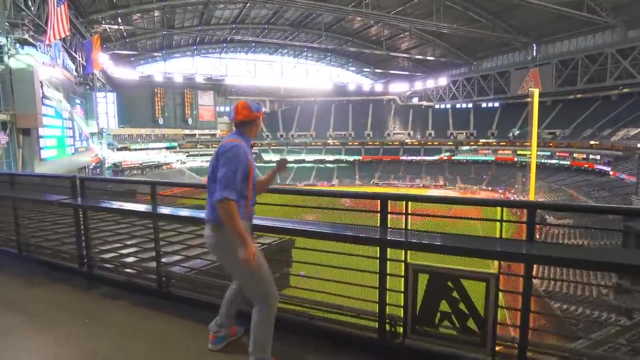 can even get around with them super fast. All right, I gotta go get Dr Evil. now I've got to go with the guys. After the game I had a happiness break. Is that a accordion? Mhmm, Oh, I was just watching the players warm up. 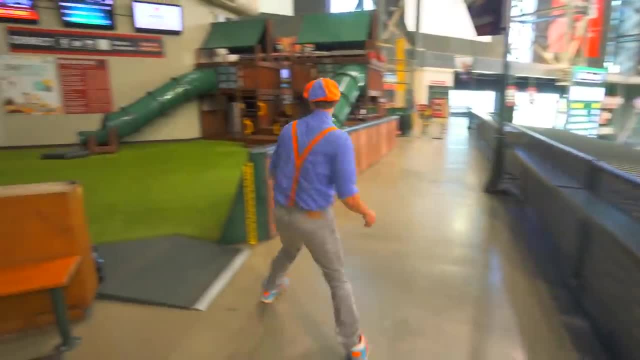 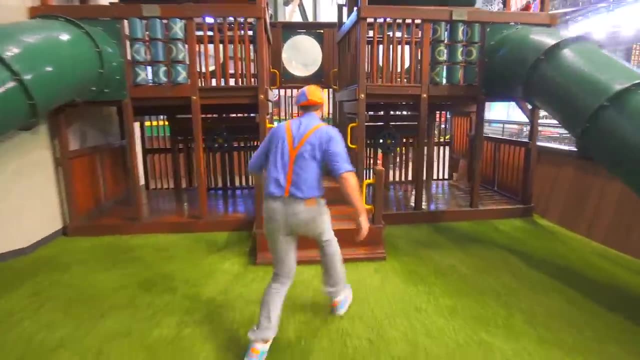 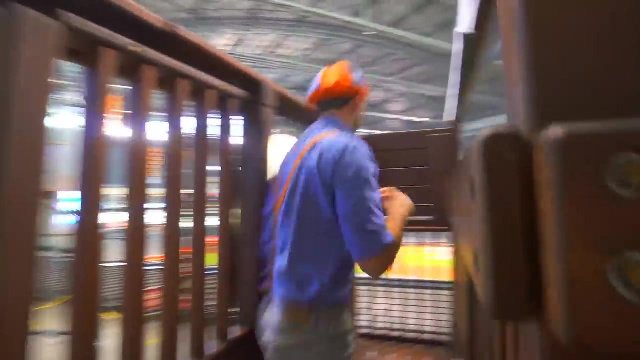 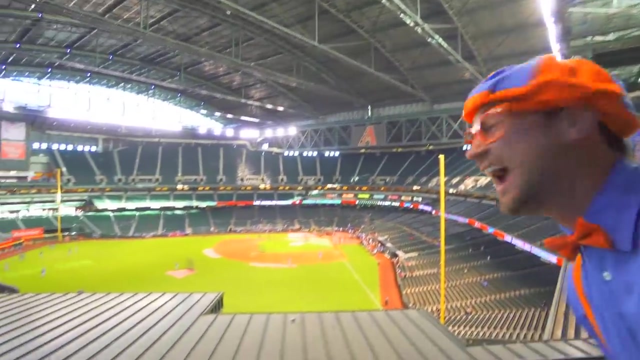 Whoa, pretty cool. Hey, check it out. Ooh, a playground. This stadium rocks. Whoa, come on. Whoa, look Whoa, we're so high in the air. What a great view. All right, now let me go down the slide. 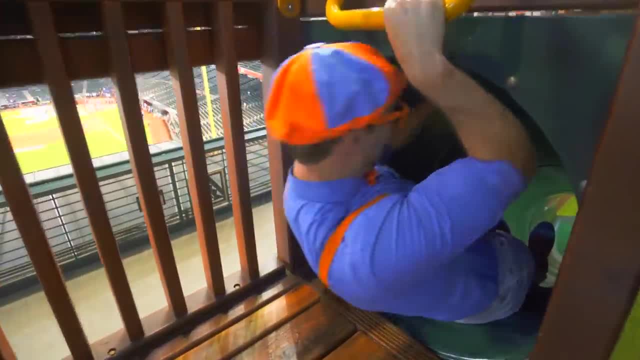 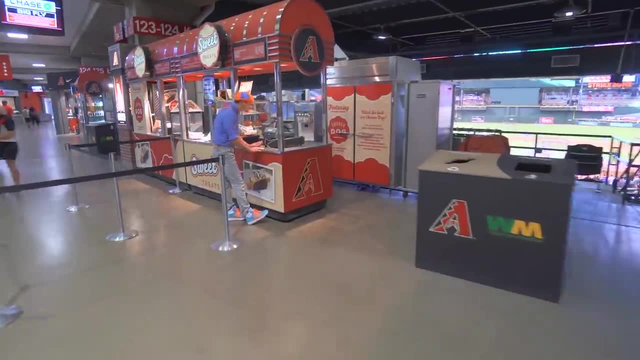 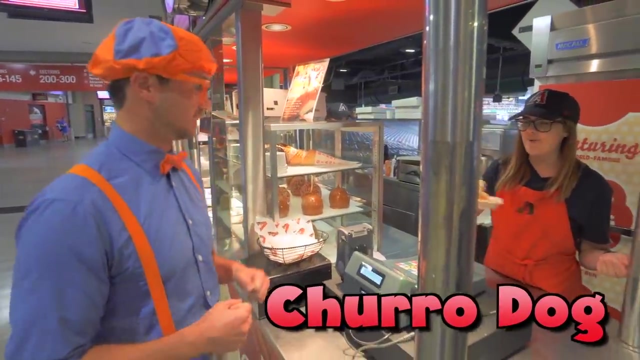 Okay, here I go, Whee Whoa. Oh hey, I'm just waiting for a churro dog. It's their specialty. Here you go, Blissy, Enjoy Ooh. thank you, Whoa, check it out. 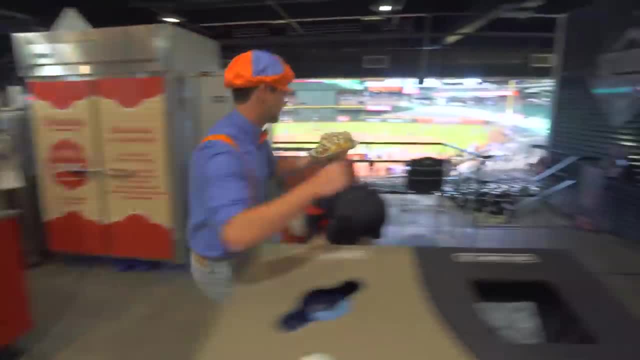 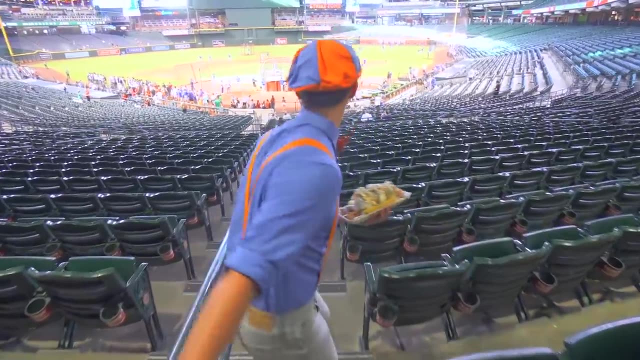 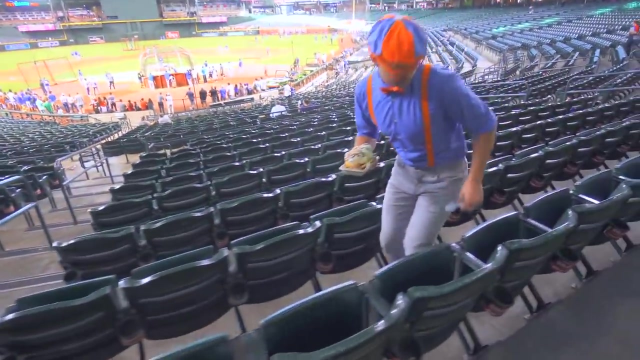 It looks so yummy. Okay, let's go take a seat. Whoa, Whoa, check it out. They're warming up. Okay, let's take a seat. Ooh, this seat looks good. All right, Whoa, look. 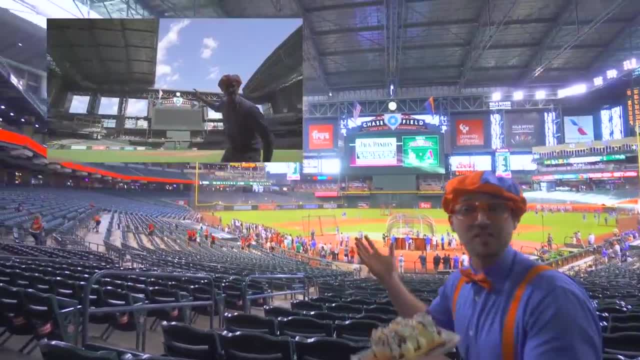 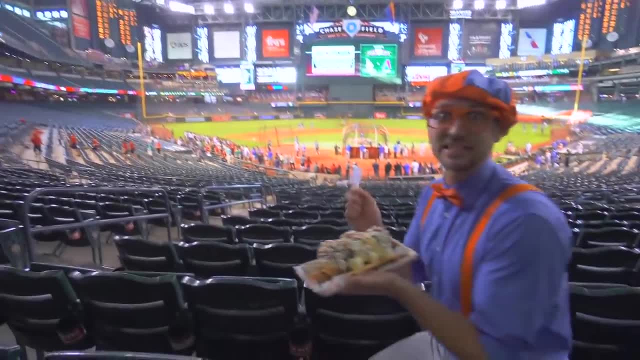 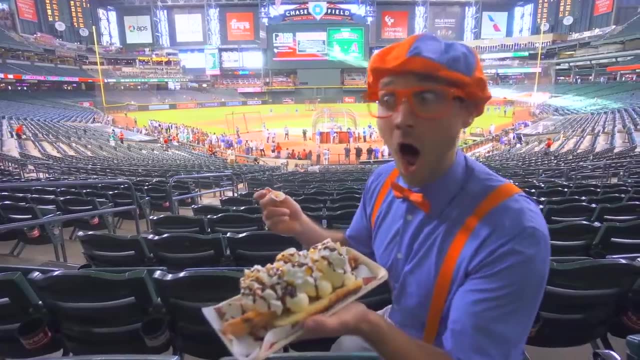 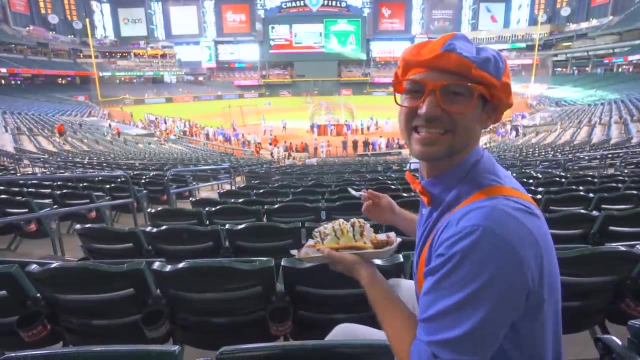 Yeah, And all the players are warming up. Okay, this is the perfect time to try the churro dog. Oh yum, Whoa, That's so good. This is going to be fun. This is going to be fun. 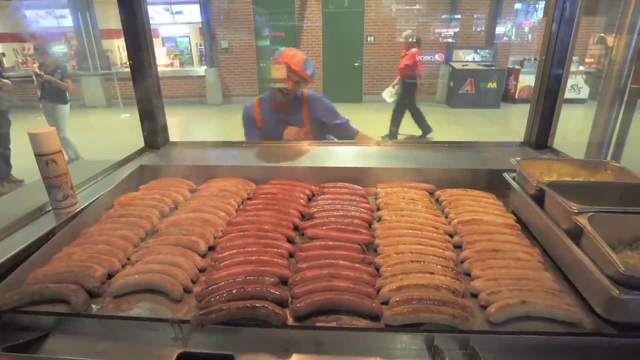 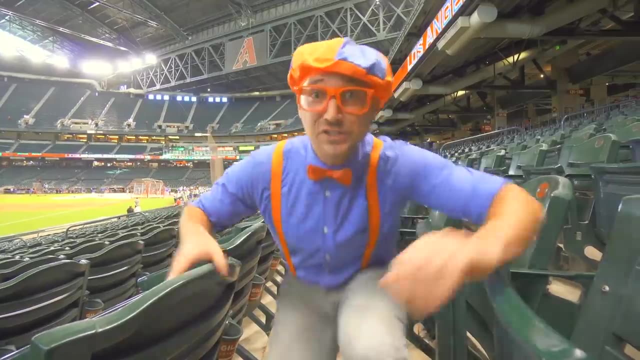 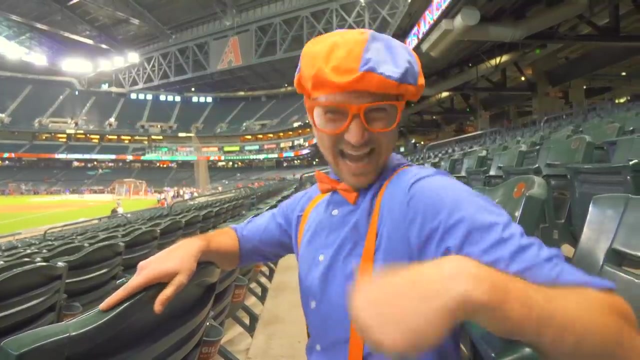 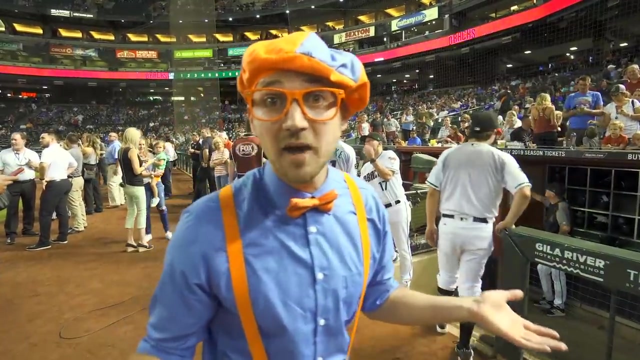 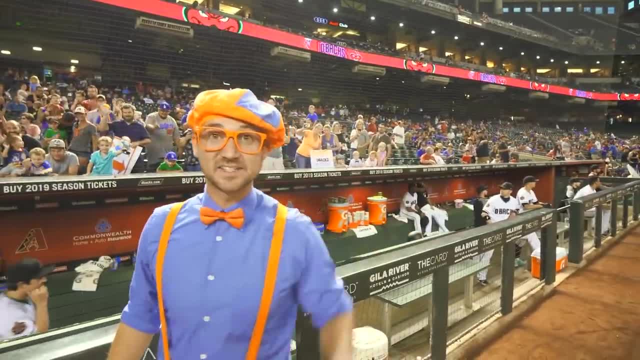 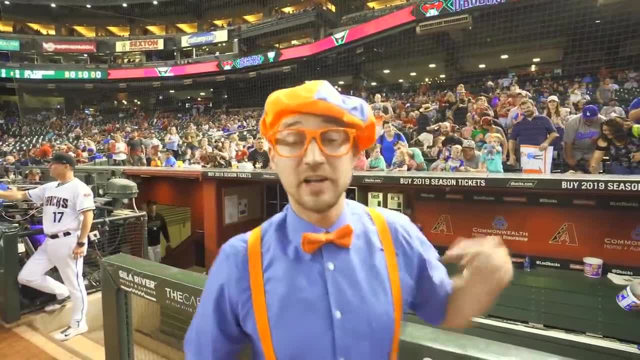 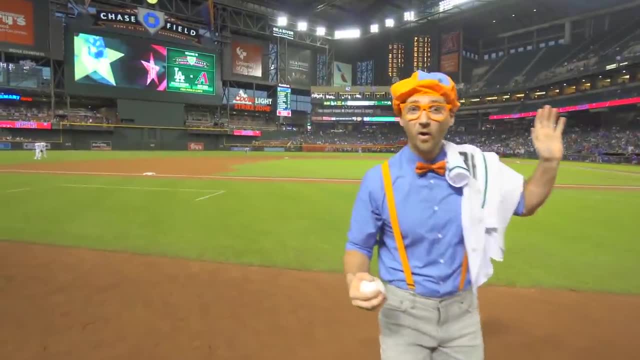 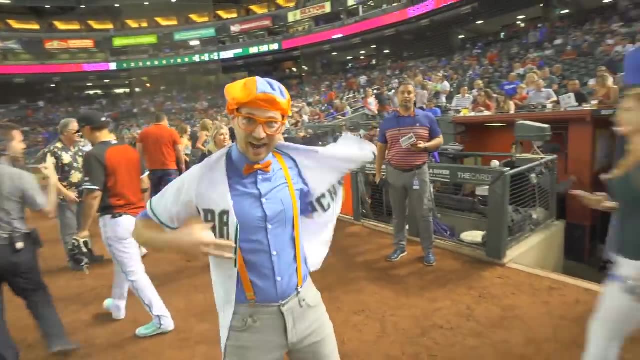 Hello, Some of them are even dressed like me. This is so cool, Whoa. Okay, I'm about to throw the first pitch. I need to put on my jersey. How do I look? Yeah, Check it out. Whoa. 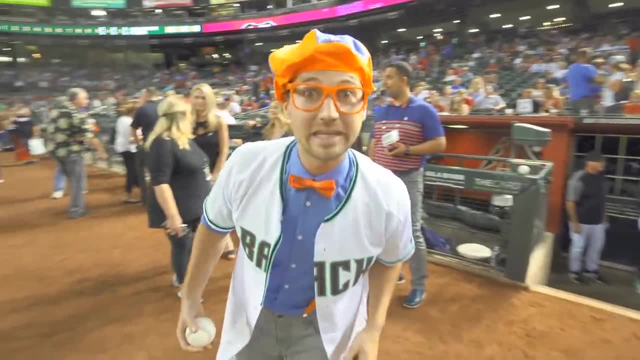 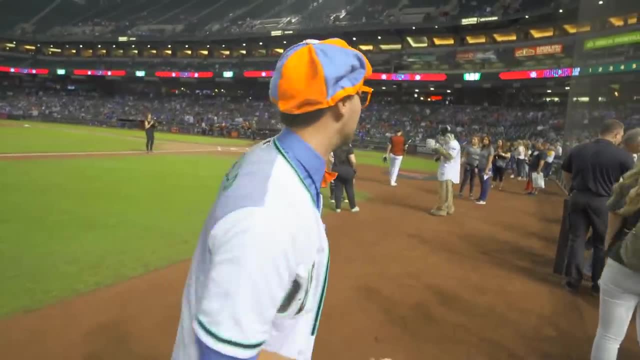 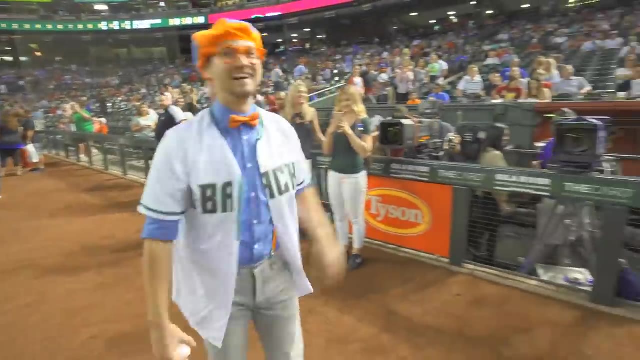 Whoo-hoo-hoo-hoo. Okay, All right, we need to get ready. This is the exact ball I'm going to throw. I don't know where to go. Got to warm up. How do I look? Do I look? pretty good? 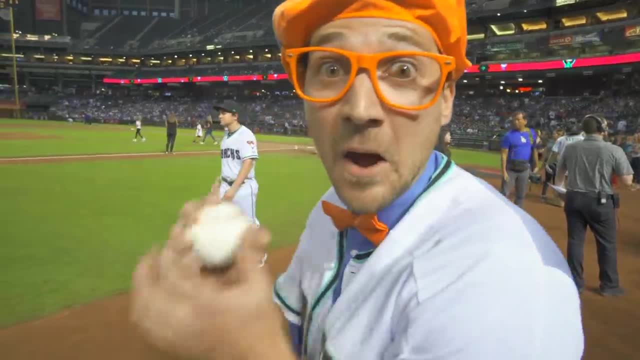 Ha-ha, I'm so nervous. I hope I make it all the way to the top. I'm so nervous, I hope I make it all the way to the top. I hope I make it all the way to the top. I hope I can make it all the way to the catcher. 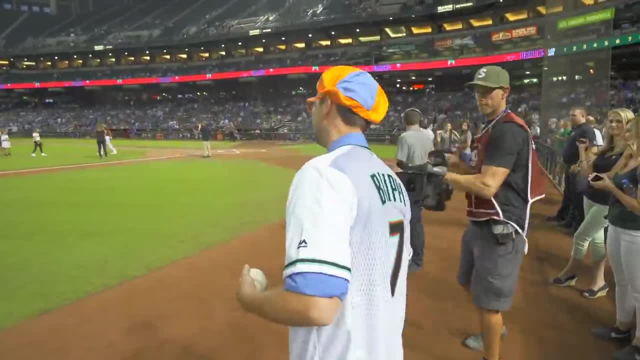 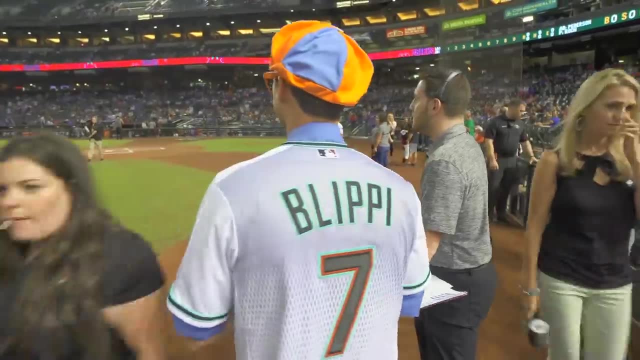 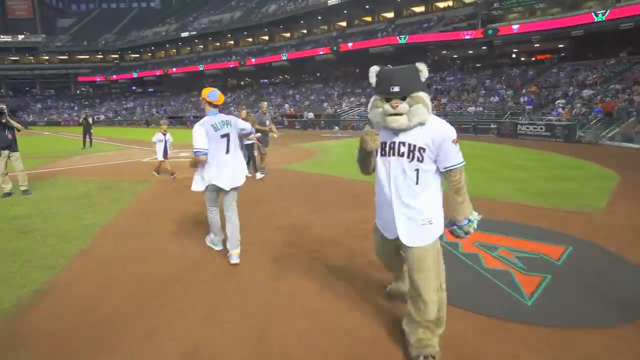 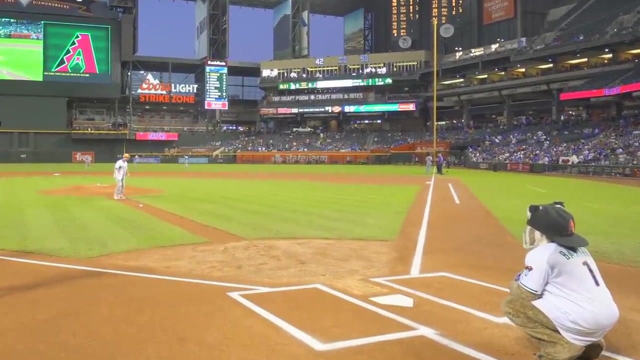 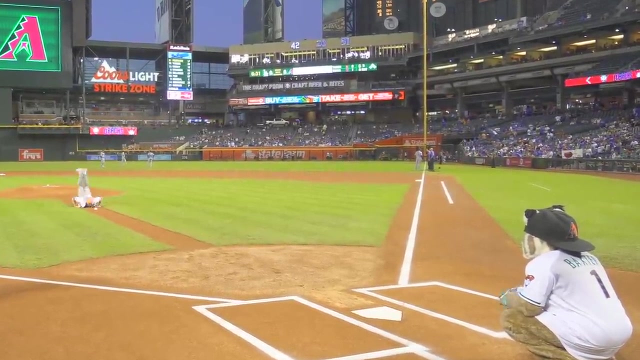 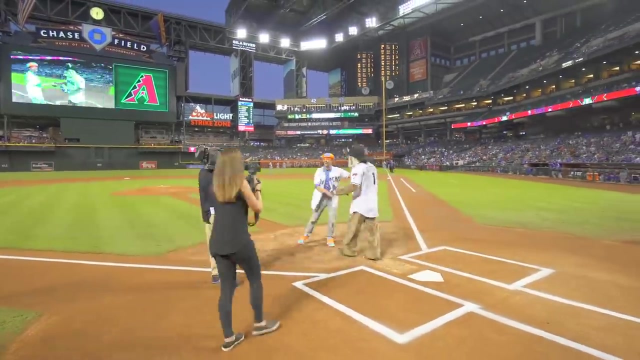 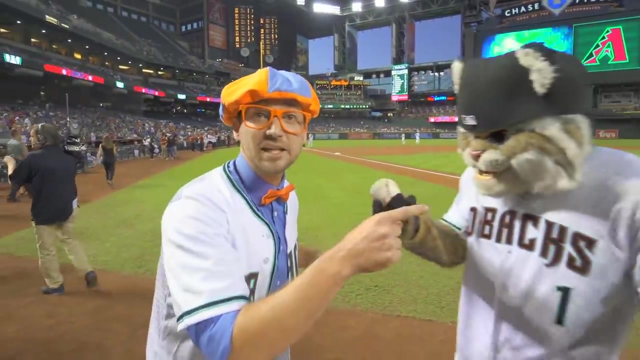 That was really good. Ooh, Baxter's going to catch the ball. Okay, here we go. This is our time to shine. Yeah, Did you see that? I threw it directly to Baxter And I think I did a strike Did. 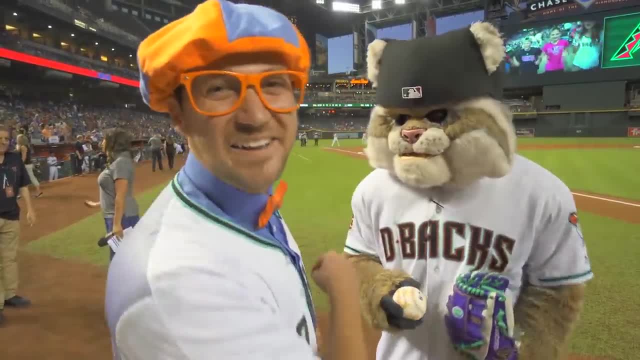 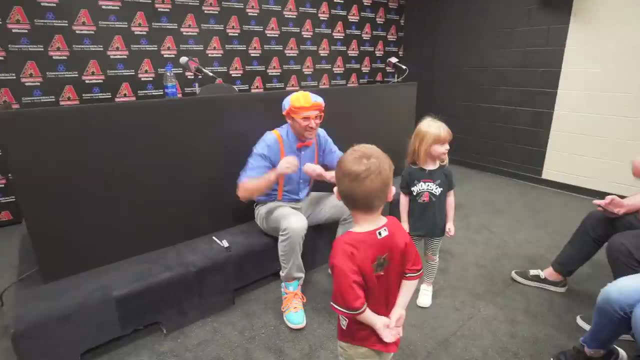 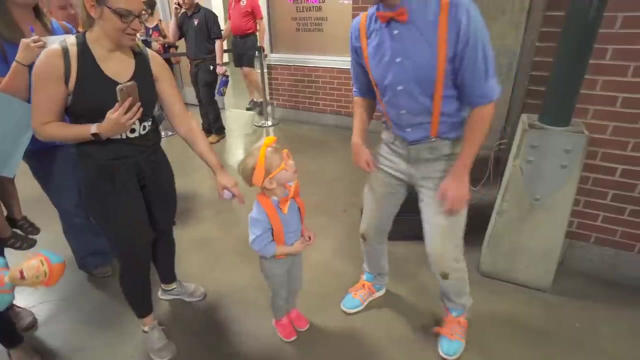 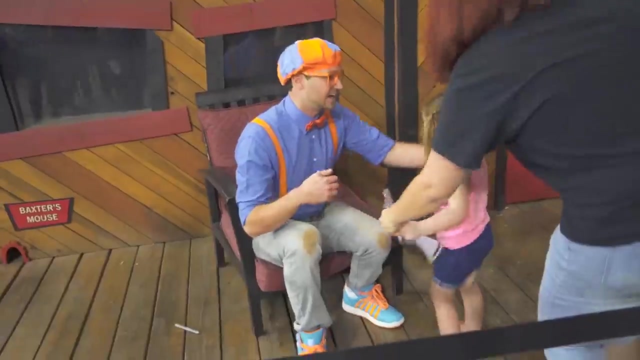 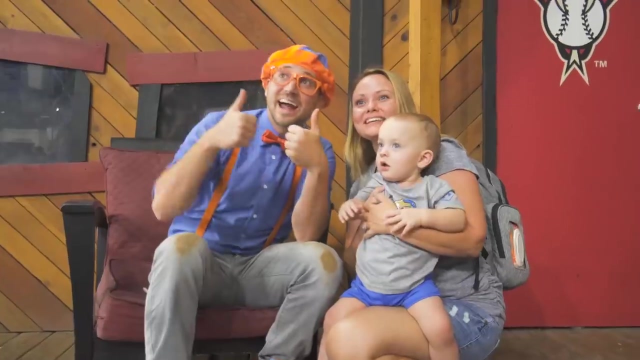 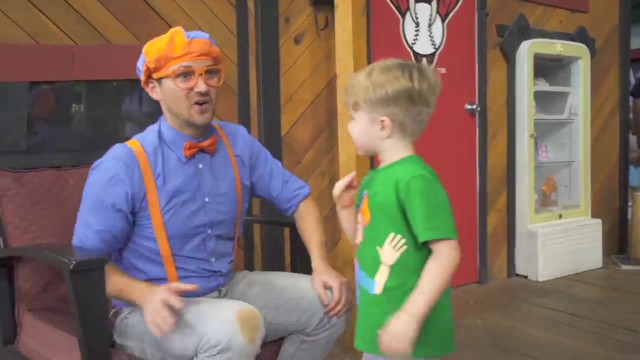 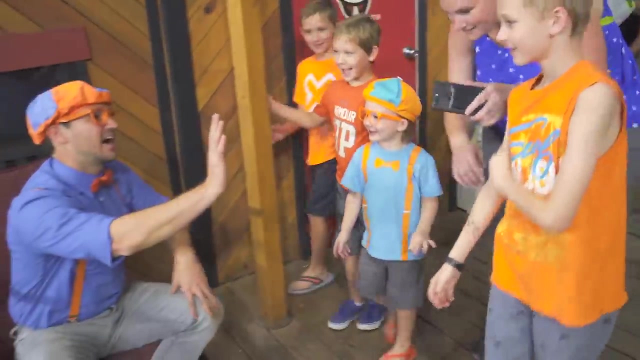 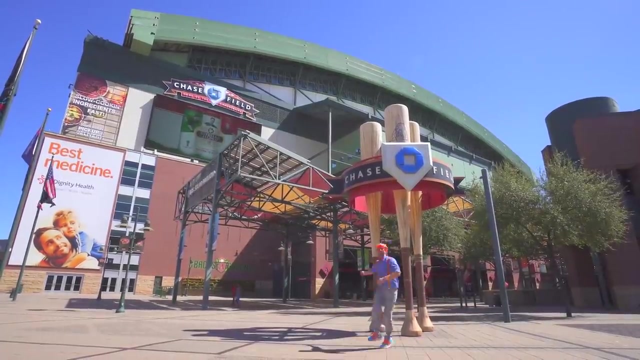 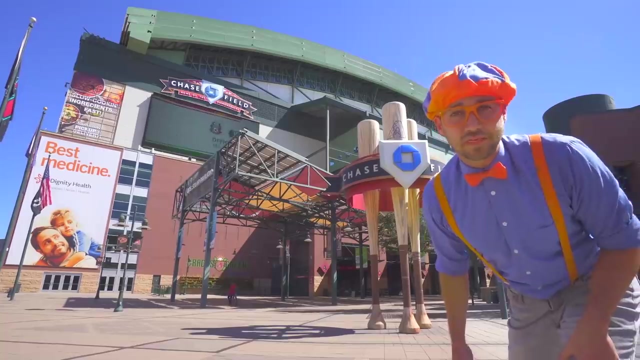 I do a strike. Strike, You're out of there. Woohoo, You're out of there. Whoa, That was so much fun learning about baseball with you. Did you have a lot of fun? Yeah, Yeah, I did too. 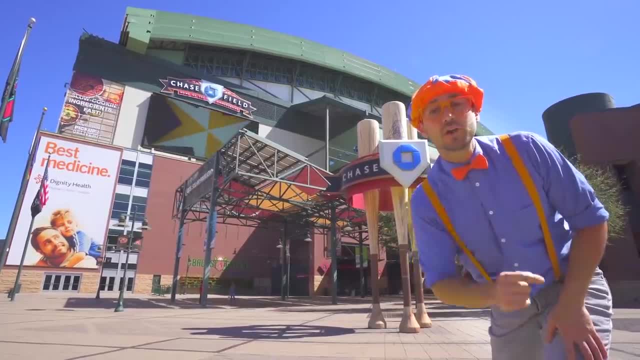 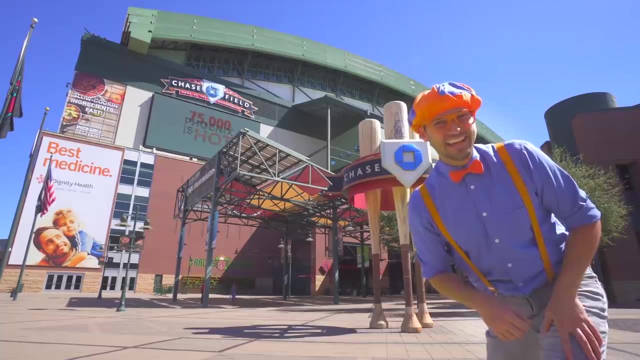 Well, this is the end of the video. See you next time. Bye, Bye. We need to get a flea. I У, uh, Yup, Wow, Here's my flea. Let's try. We got a flea now. Here's a flea now. 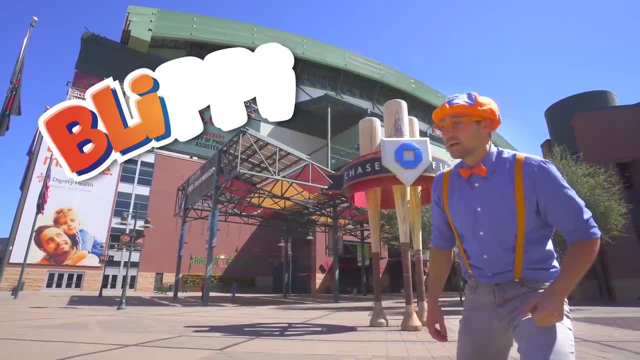 Come see who I drew: Amsterdam, Cleveland, Memphis, Dakota, Berkeley, Tough Fair. These were my first podemos. I won two points, But still there's a flea. Let's see who we need to draw, And even if we don't get 3 points, we still get 3: Sakura. 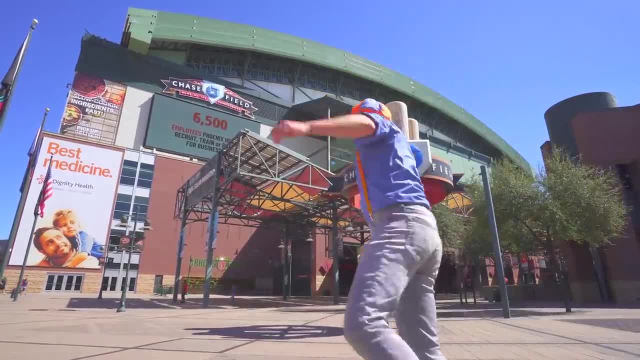 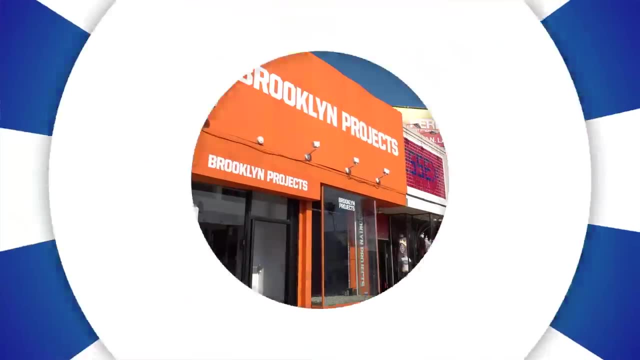 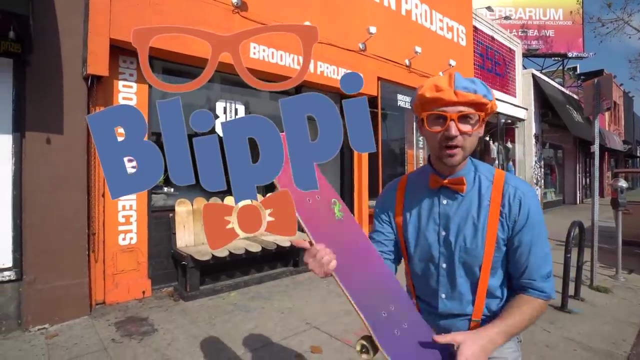 We start. How about a good start, guys? Olá Crisis, There we go, But I almost do a flea Blippi, Fun chordals. uh Yeah, Plea Everyone vocabulary. Hey, it's me Blippi, and look at what I have in my hand. 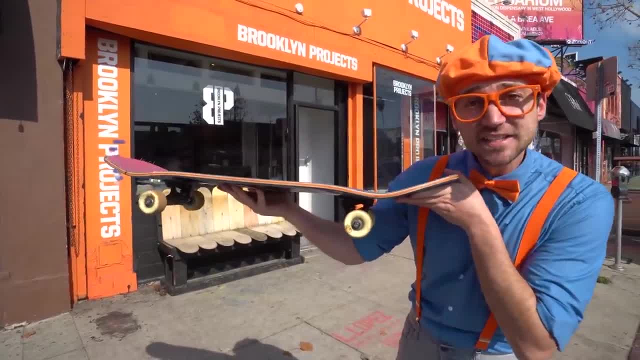 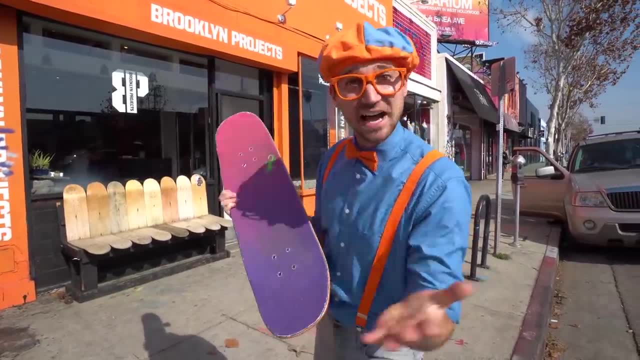 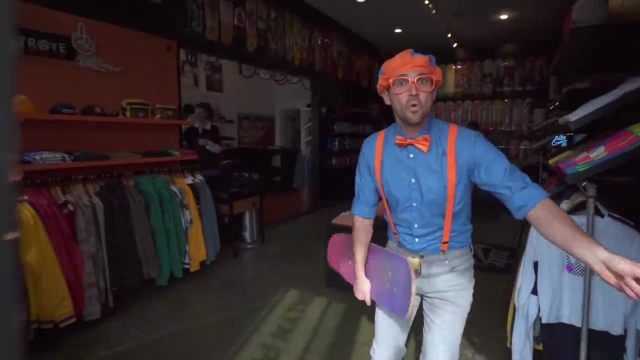 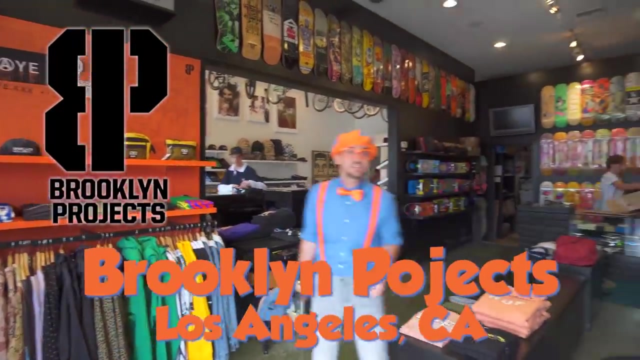 Whoa, do you know what this is? This is a skateboard and I think you and I should learn about skateboarding. Come on, Whoa, look at this store. This is the Brooklyn Projects in Los Angeles, California. Whoa, this place is so cool. 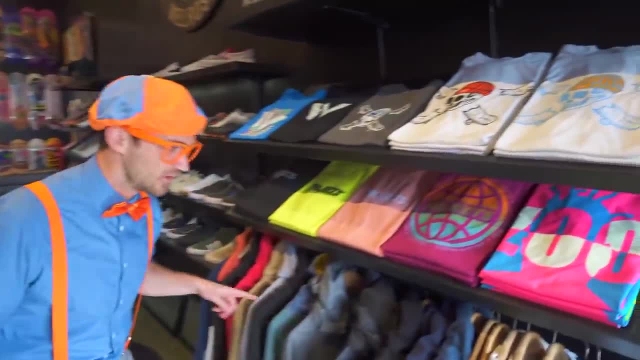 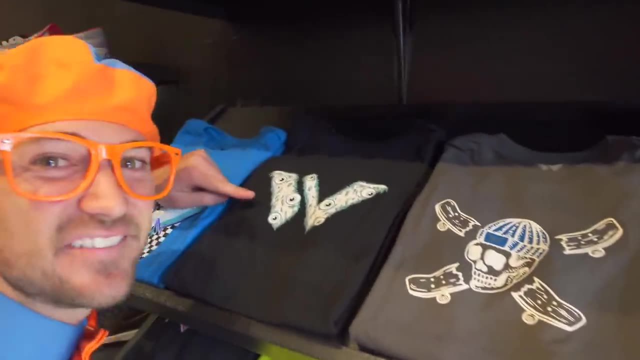 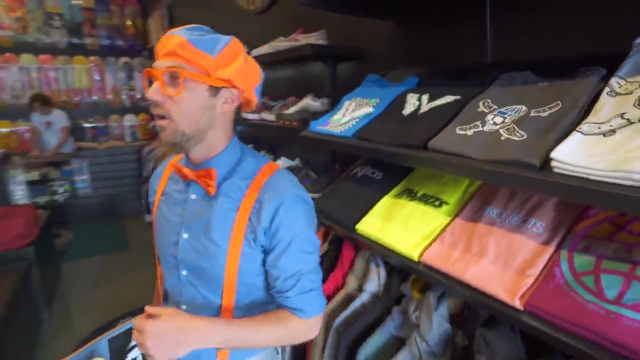 Whoa, check this out over here. Whoa, cool apparel. Whoa, look at these designs up here. Ooh, look at this. It's so fuzzy like a monster and it's the letter W. Pretty cool, Whoa, come check it out. 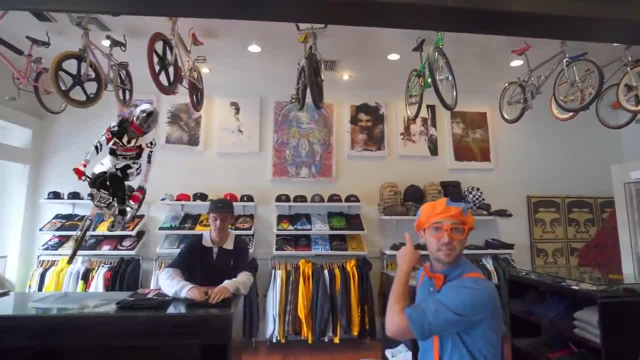 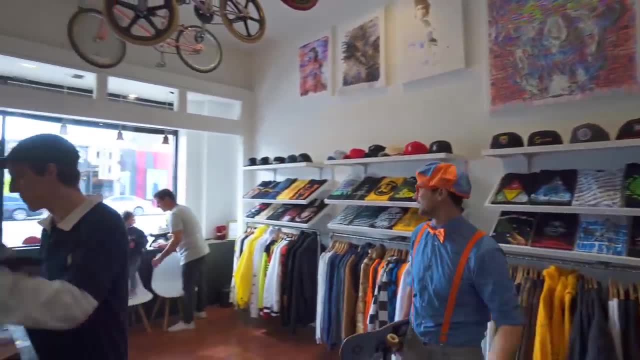 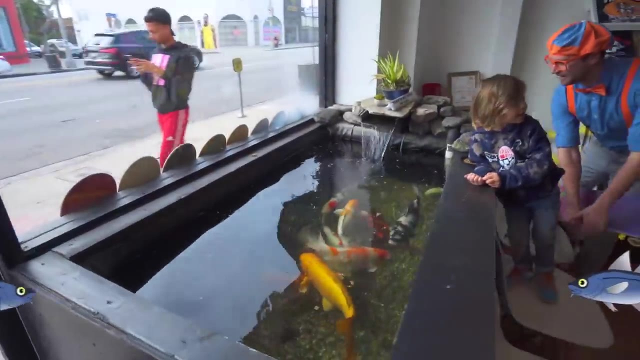 Skateboard deck. There's BMX up there, even BMX bikes. Whoa, this store owner must really love skateboarding and BMX bikes. Whoa, what's over here, Hey, Whoa, what are you doing? Whoa, are you feeding the fish? 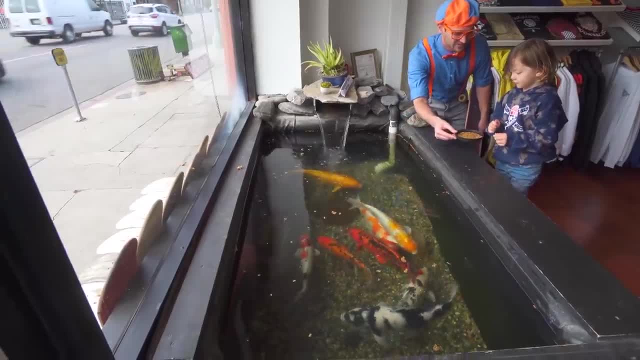 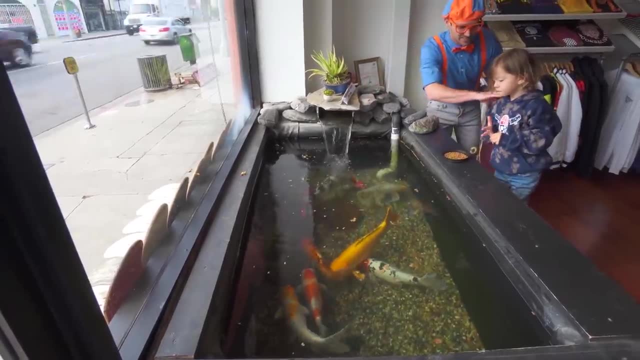 This shop has a bunch of fish Here you go. All right, throw it in there. Whee, All right. bye-bye fish, All right, see you soon. All right, hey, I think it's time to see if one of the workers will help me learn how. 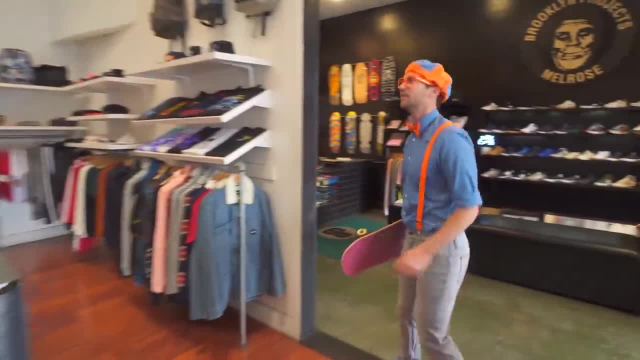 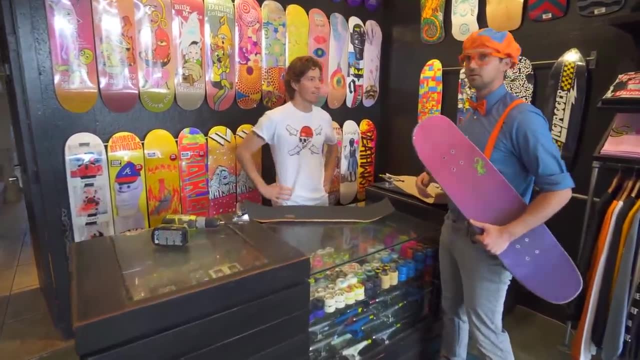 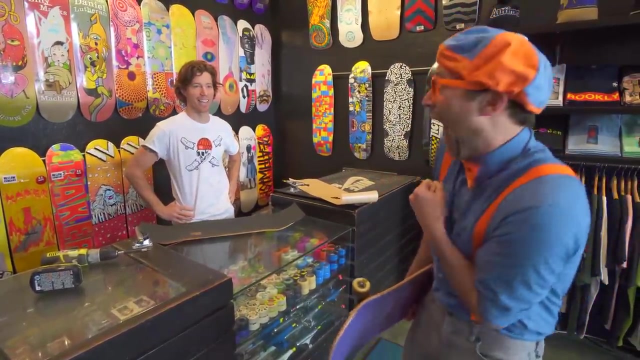 to skateboard. Come on, Whoa, pretty cool, Here's one. Come on, Hey. Hey. good sir, Carry, my s- How's it going? Do you know who that is? That's Shaun White. That's Shaun White. 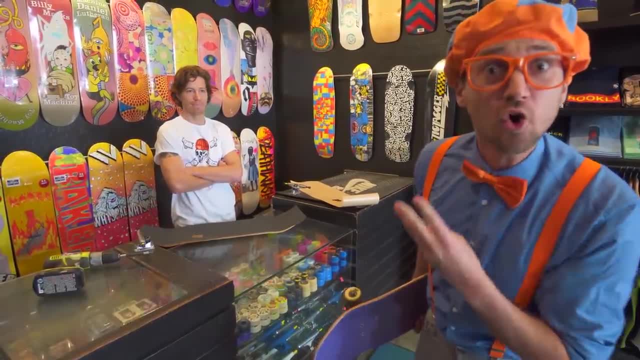 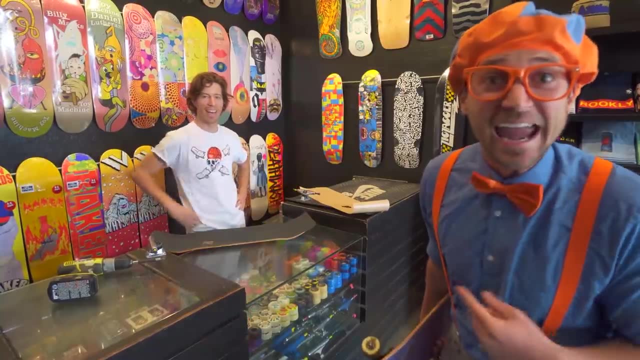 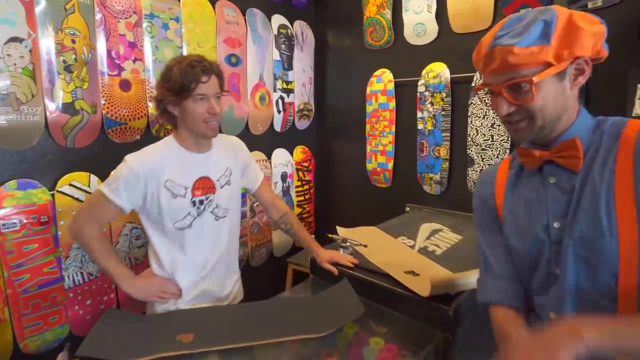 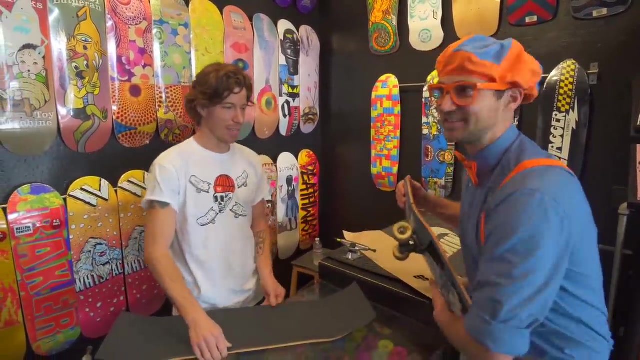 That's Shaun White. what he's won three gold medals in the olympics for snowboarding- one, two, three- and he's a professional skateboarder. let's ask him for help. um, can i help you? i just uh, yeah, just curious if you could uh help me learn the skateboard today. oh, yeah, you want to learn. 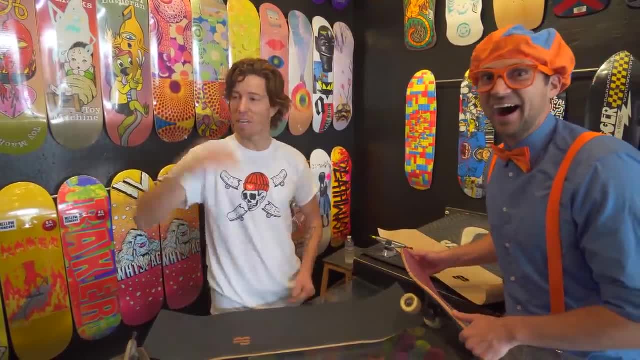 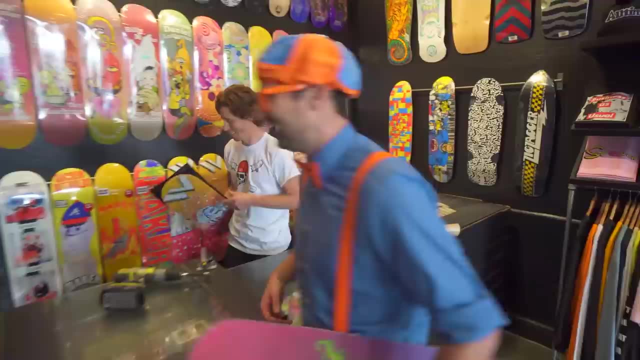 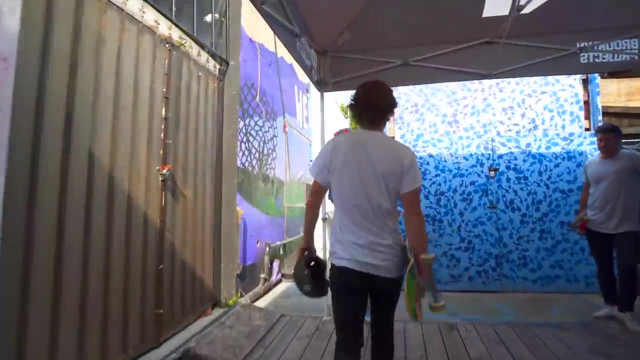 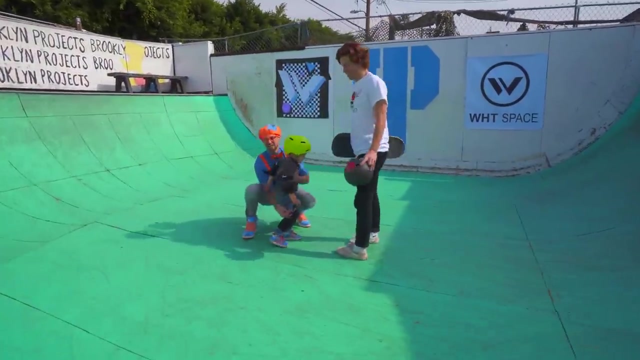 how to skateboard. you know, i've been skateboarding my whole life, love doing big airs and things. i'm just setting this board up and we'll take you out back, show you how to do it. okay, let's go, whoa, check it out. yeah, whoa, this is a big ramp. is this where you skateboard at this? 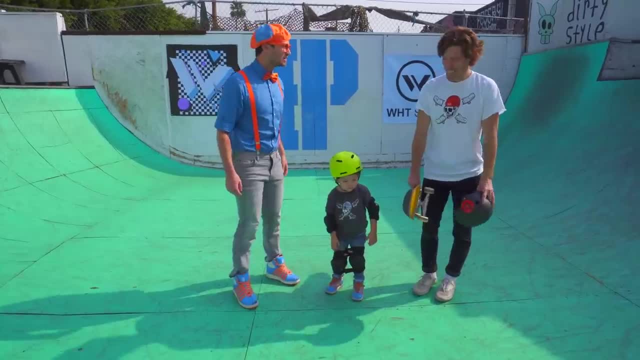 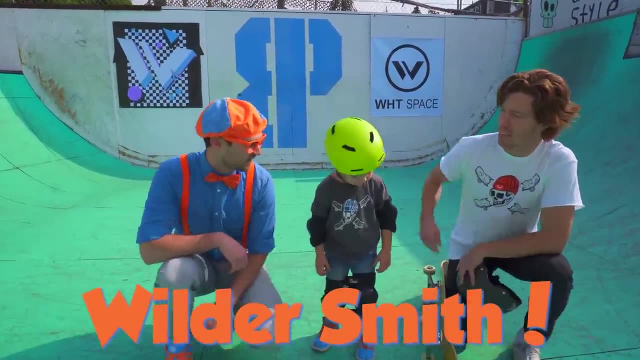 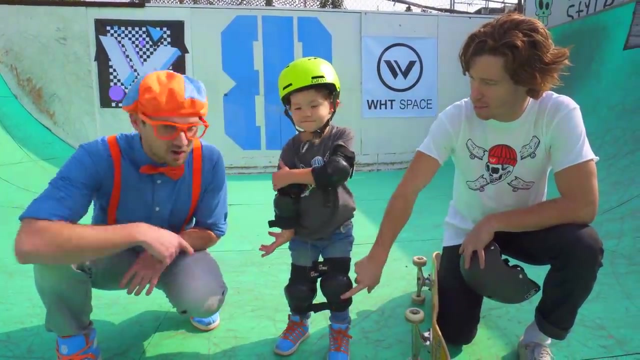 is: oh, pretty cool. all right, well, will you show us? well, hold on, you know you're gonna need some protection of gear first. all right, what's that? check out my buddy wilder here- whoa, he's got a helmet, wow, yep. then he's got his elbow pads right here- yep. and then you got your knee pads down here. 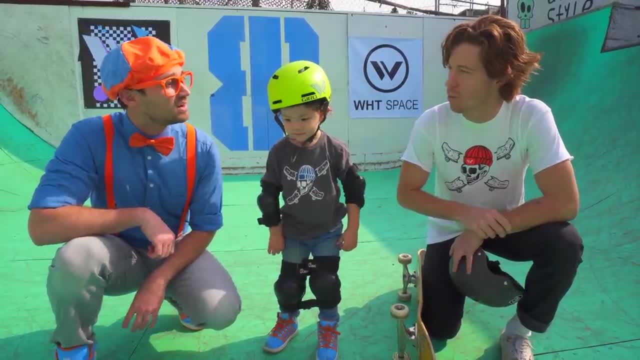 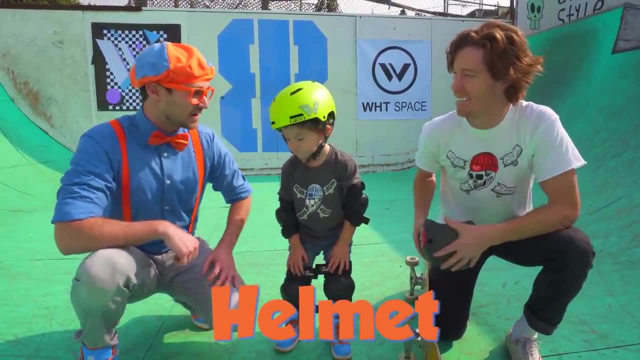 and this is to help protect you for if you fall, just in case of a fall. whoa, that's pretty cool. and what are you gonna wear to be safe? i brought my lucky helmet. okay, well, put it on and let's see your ride. here we go, guys, all right here, you want to come this way? let's go. 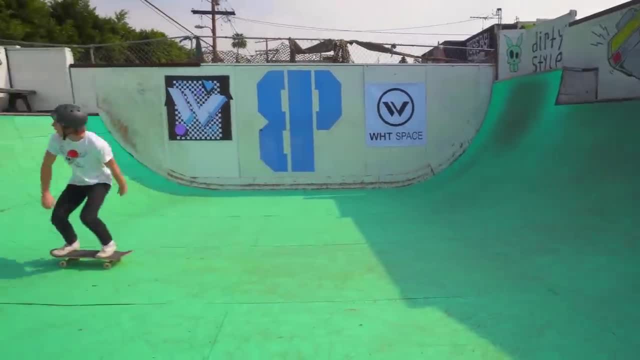 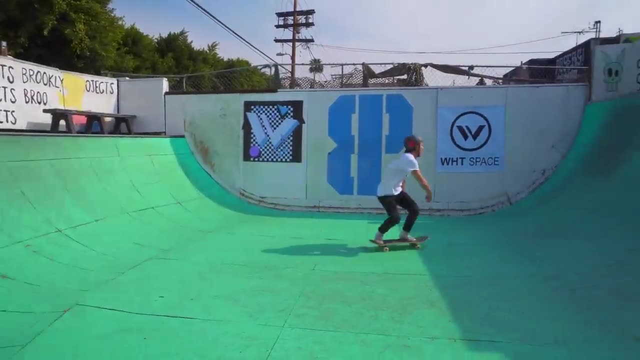 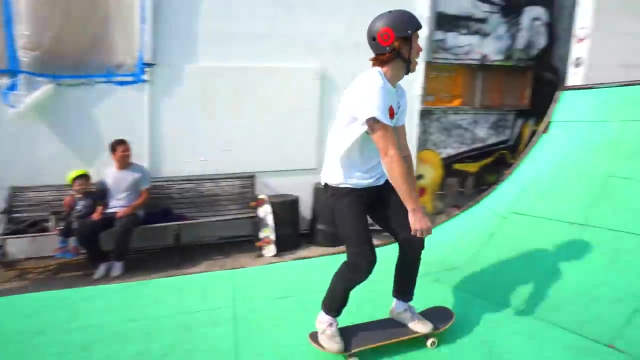 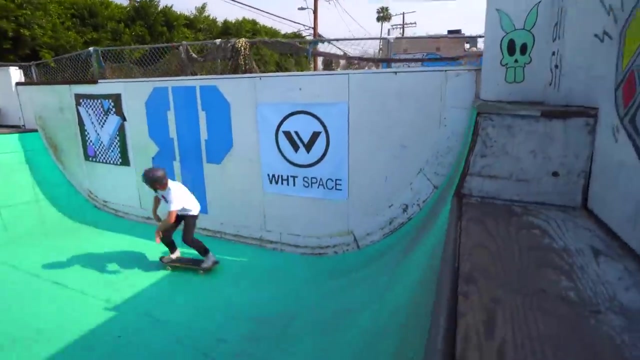 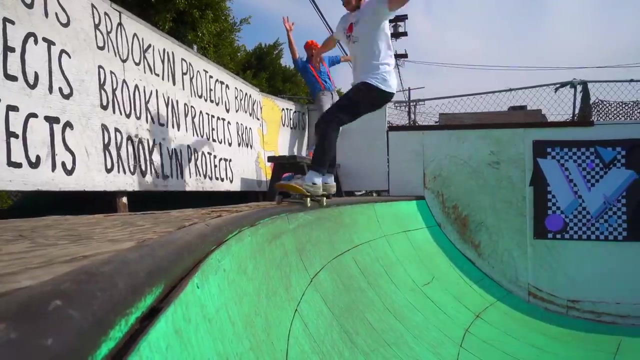 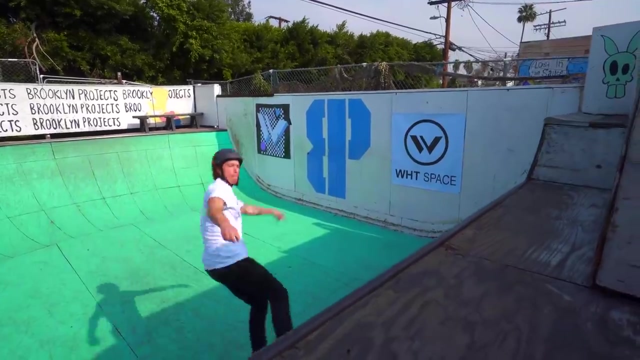 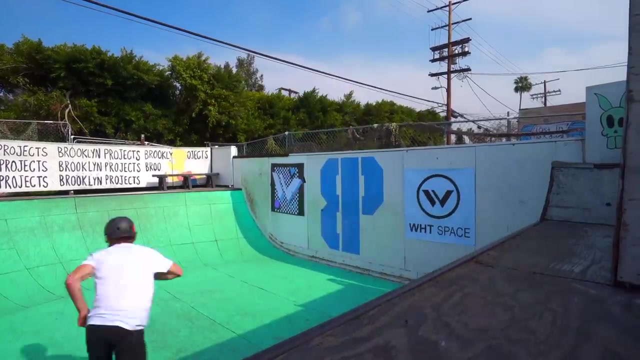 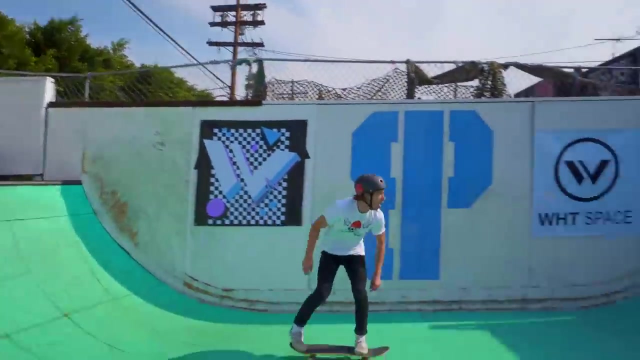 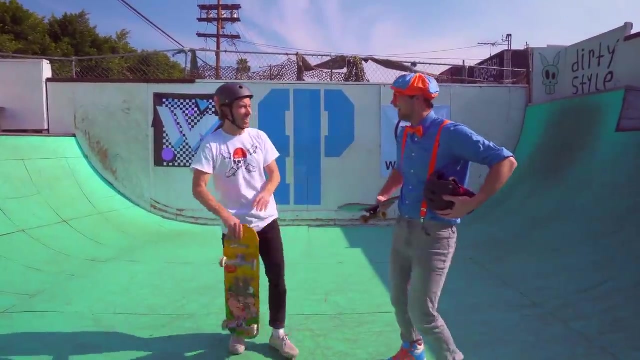 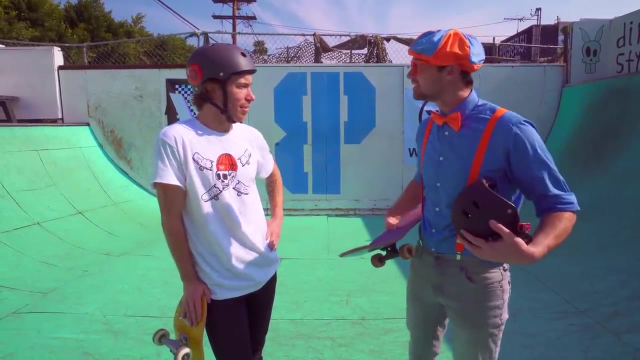 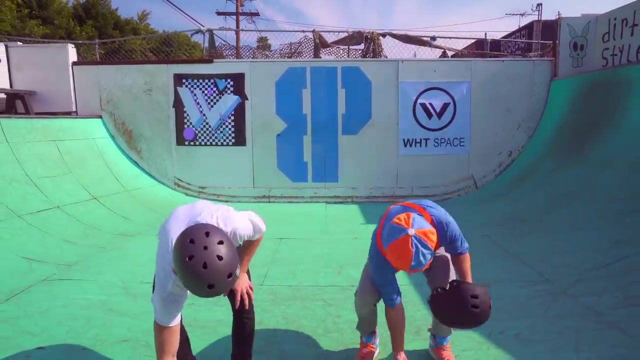 here we go so. so that was so cool. well, you know, i've been working really hard at this for a long time, so if you practice you'll make perfect. oh well, that's good to know. can i try now? of course, okay. okay, first thing, put the board down. okay, i'm gonna put your helmet on. all right, go okay now put whatever front. 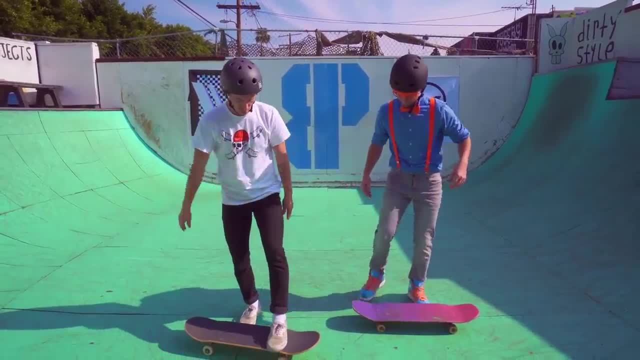 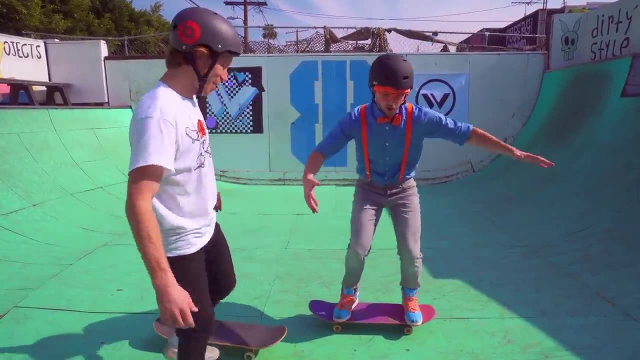 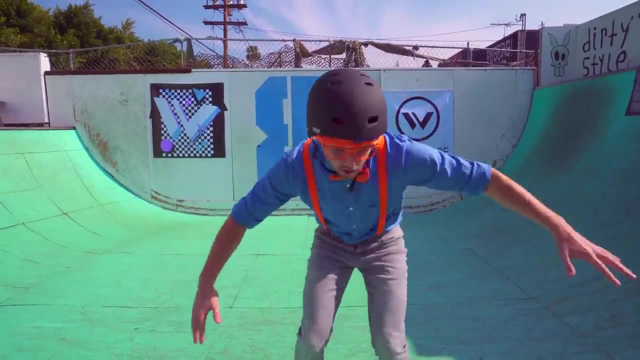 foot feels good, okay, right toward the front of the board, all right. and then you pull the back foot on, oh, and then you keep your knees bent. oh, that's the key. whoa, there you go. whoa, whoa. this is harder than it looks. whoa, oh, oh, all right, that was pretty good, yeah, but i think. 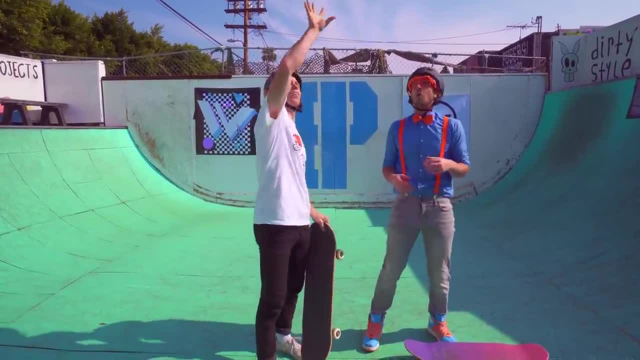 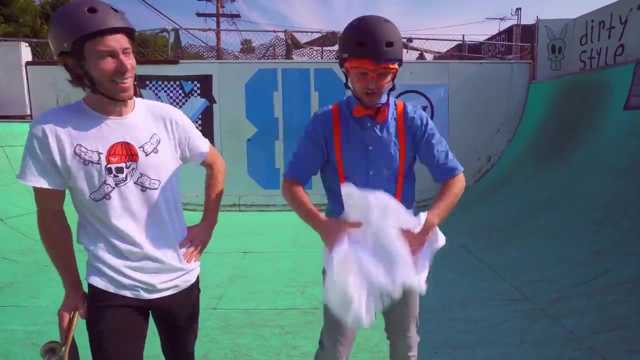 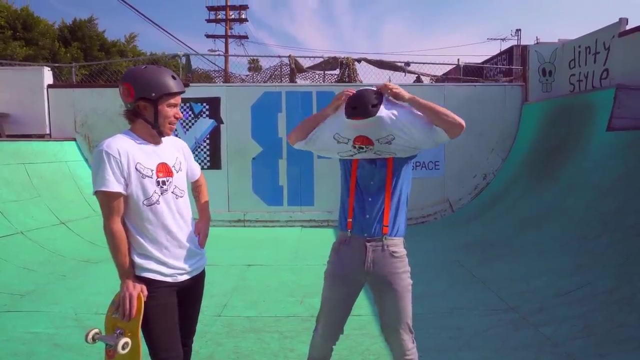 i know what you're missing. what is it? yeah, here we go. whoa got that for you: an official sean white, white space t-shirt. yeah, that's totally what i'm missing. okay, let's put this on right on. here we go. i'll help you there, oh. 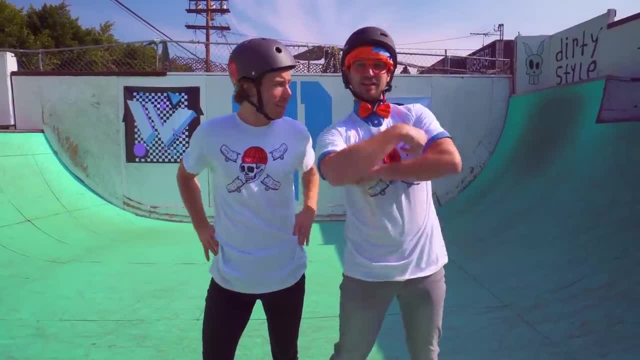 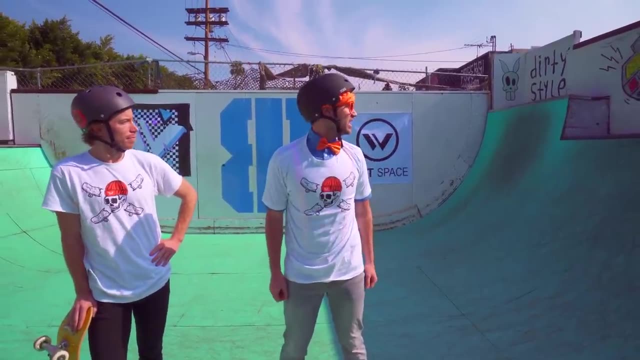 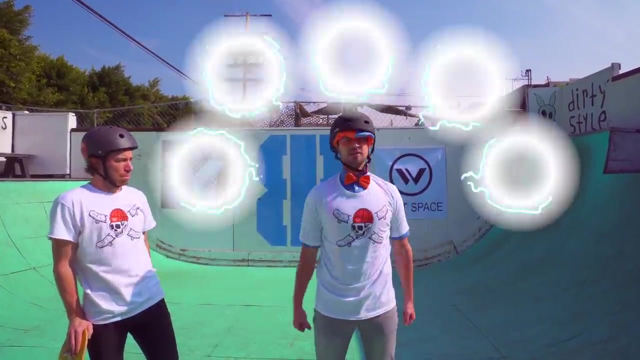 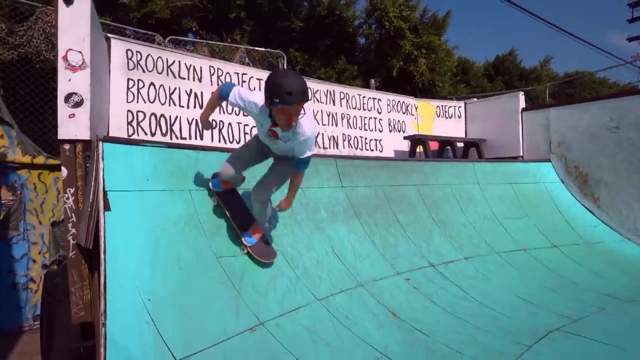 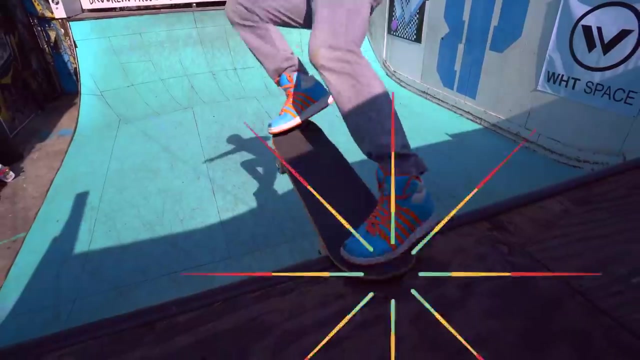 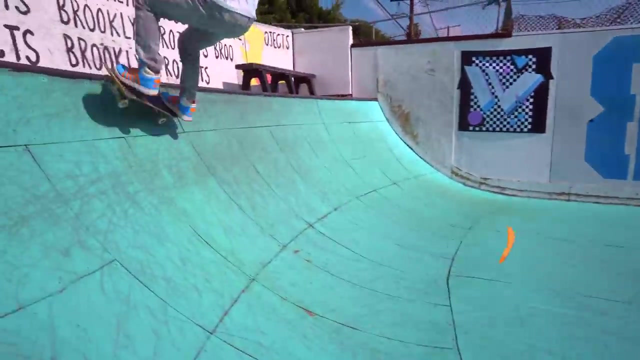 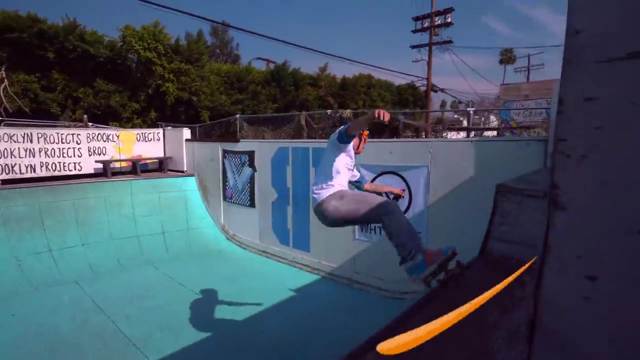 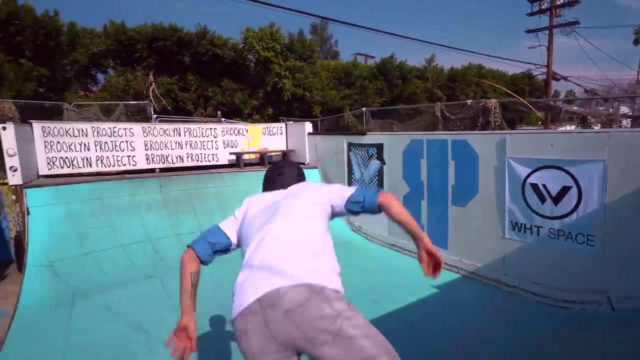 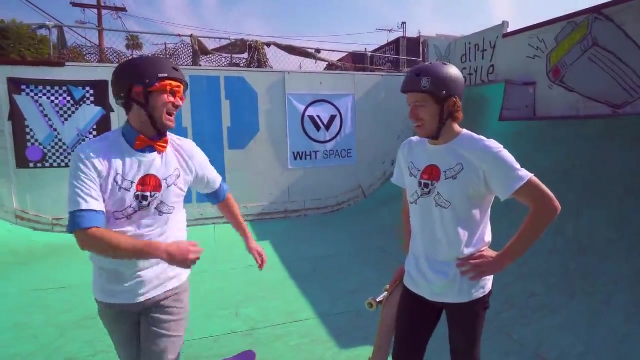 that's silly. okay, all right. how do we look? yeah, oh, and you know what else? yeah, the souls of the animal kingdom: eagle, fox, bottlenose, dolphin, octopus, house cat. i'm ready. so 06, uh, uh, all right. how'd i do flippy? that was amazing, especially for your first time. 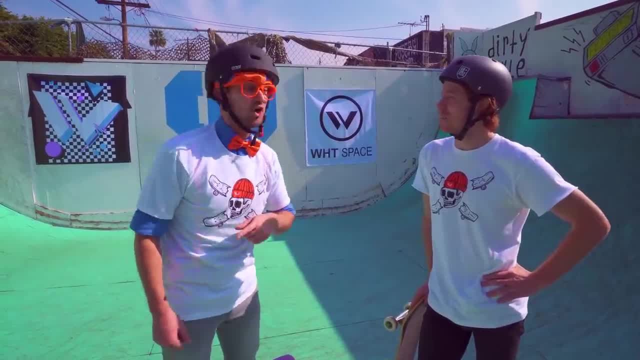 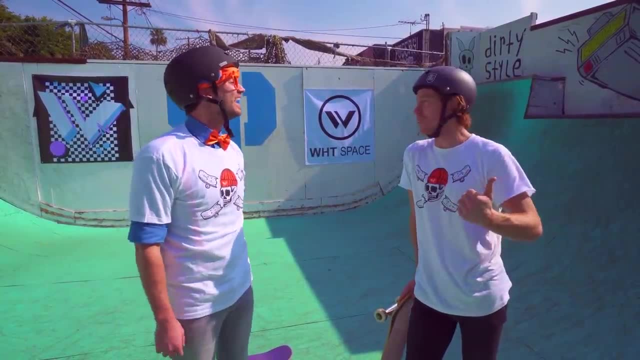 really, yeah. well, thank you very much for teaching me. with a good teacher, you can do a lot of cool things, no problem at all. well, hey, i had amazing time skating with you. i gotta head to another skate park, but we should do this next time you come. so if you'd like to come see me in your skateboard park, 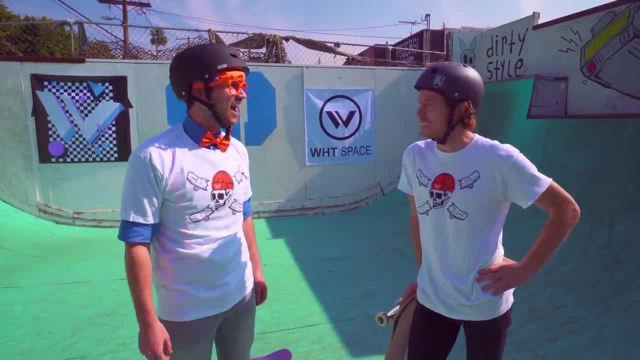 and i can get a hat. thank you very much. i appreciate the advice and the happiness of growing up in your, but we should do this again sometime. Maybe I'll take you to the mountains and go snowboarding- Really, Yeah, try that out. 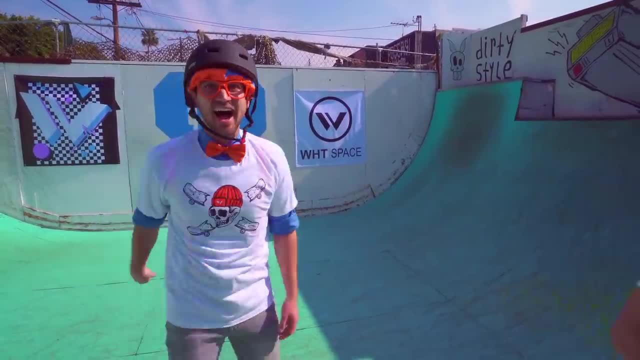 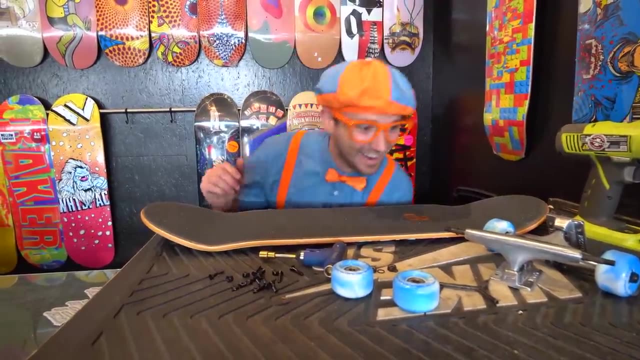 Well, I really appreciate it. All right, See you, bud, See ya, Did you hear that Maybe I'll get to go snowboarding with Shaun White? Whoa, Hey, Whoa, check it out, Let's learn how to build a skateboard. 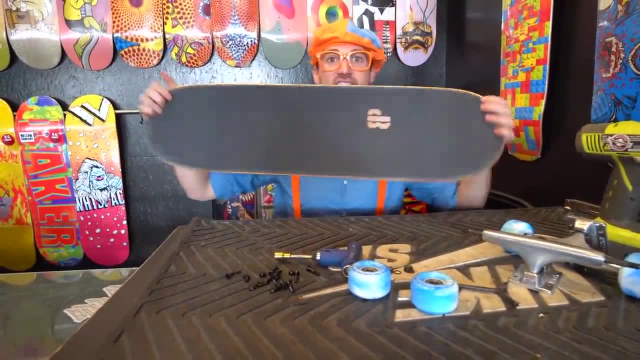 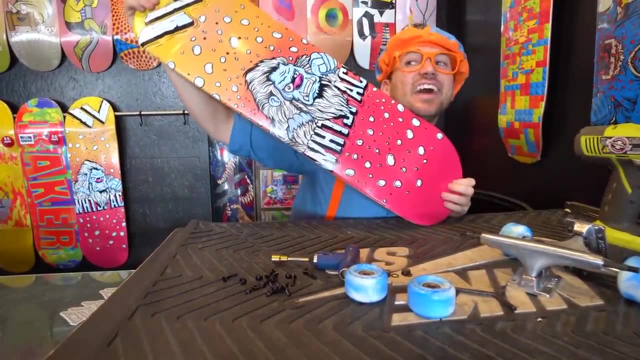 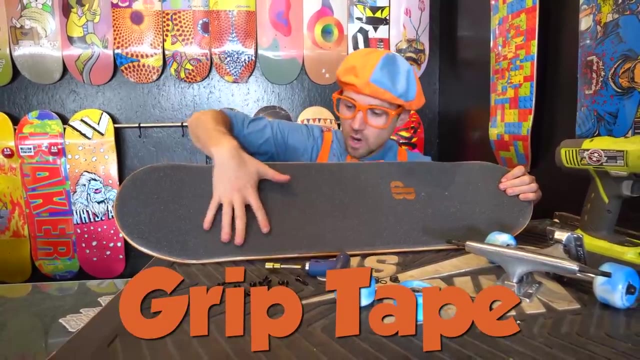 See this: Whoa. This is a skateboard deck- Whoa. And this one has a really cool design. Check it out. Whoa, That's silly. And see this on top: This is grip tape- Whoa, it's kind of like sand and you can't move at all. 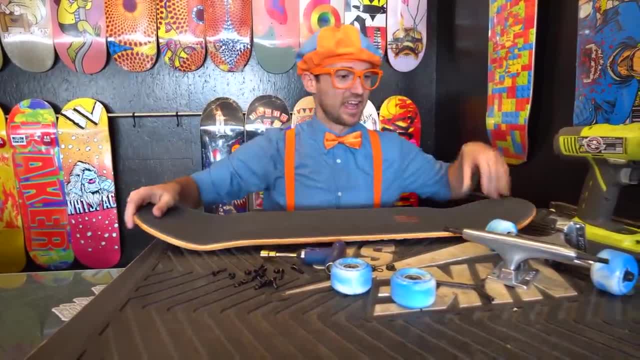 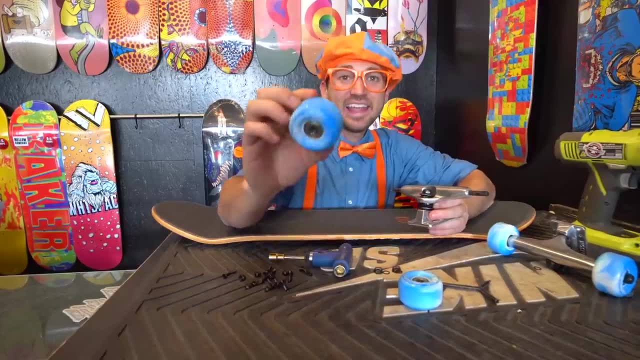 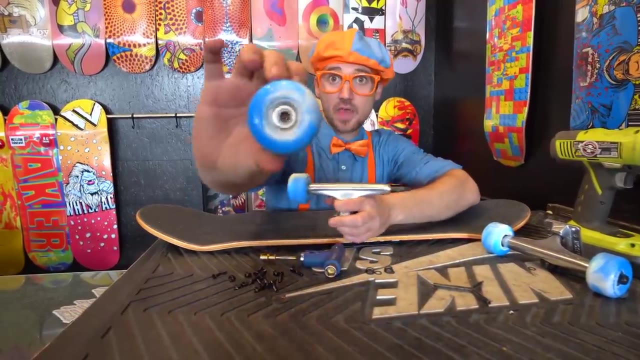 So then, your feet don't slip and slide. Okay, And this is what's called a truck. Ooh, And you know what these are? right, Yeah, wheels, And how these work. you put the wheel on the truck, put the other wheel. 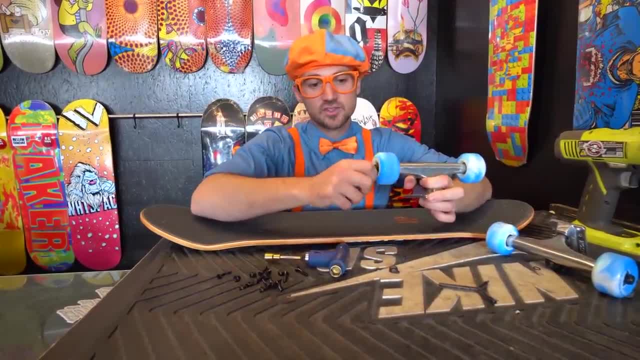 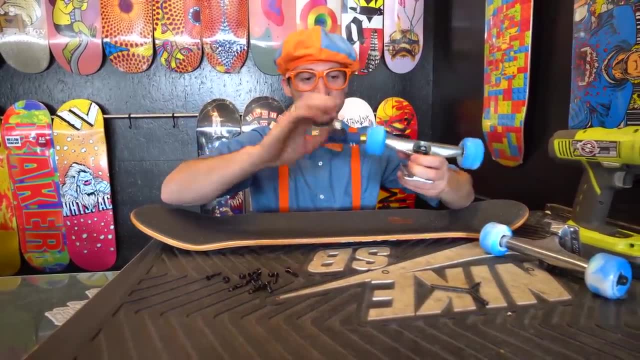 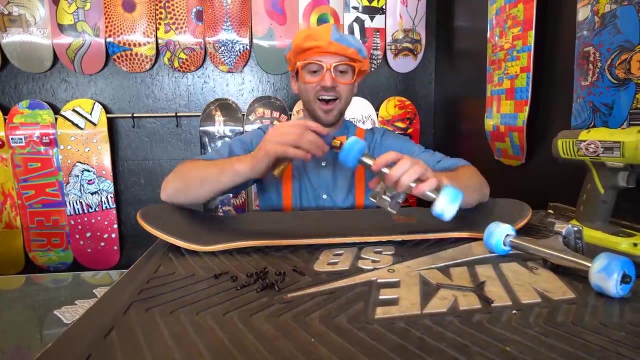 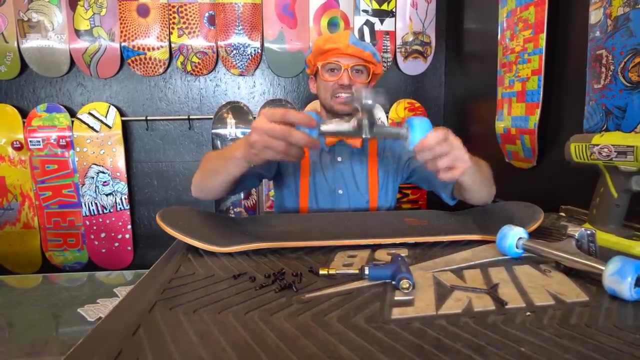 on the truck and then you screw in the nut and make it nice and tight, And then you do the other one. Whoa, All right, There we go. Whee, See it spin. Perfect, All right. So you have two trucks. 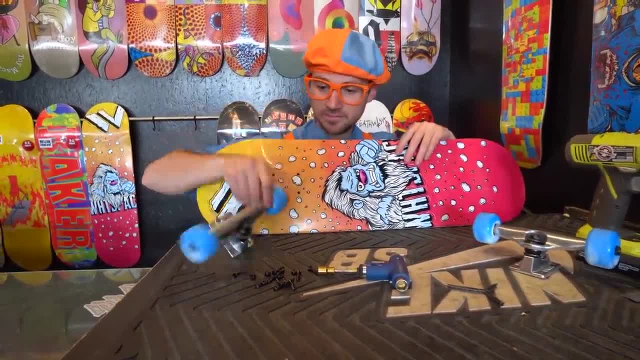 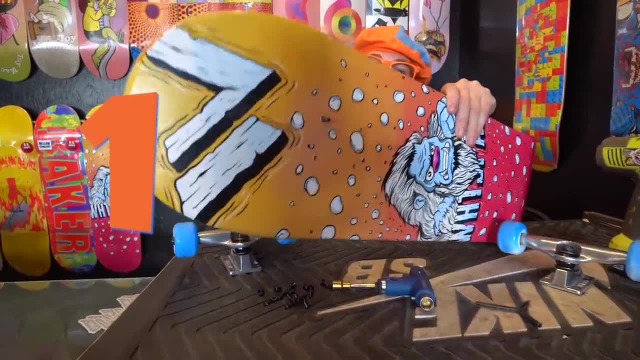 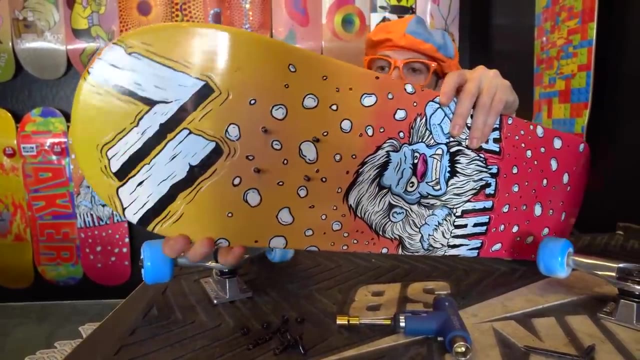 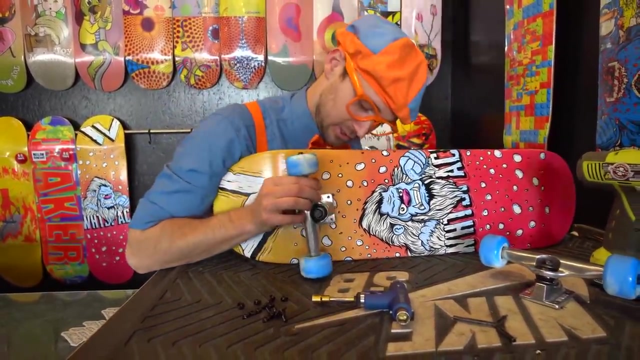 All right, And then put them on the bottom After you put these bolts through. let's put four of them in there: One, Two, Three, Whoa, Four. Perfect, Okay, let's put the truck right here. This is a little tricky. 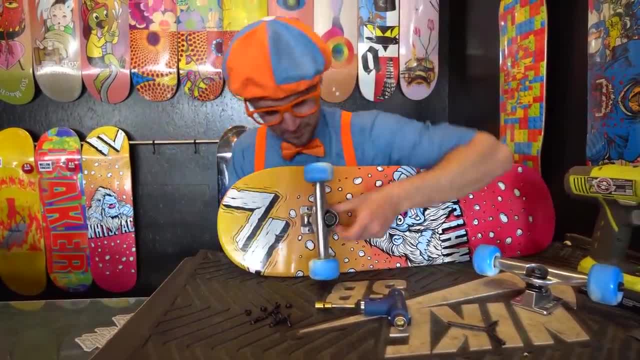 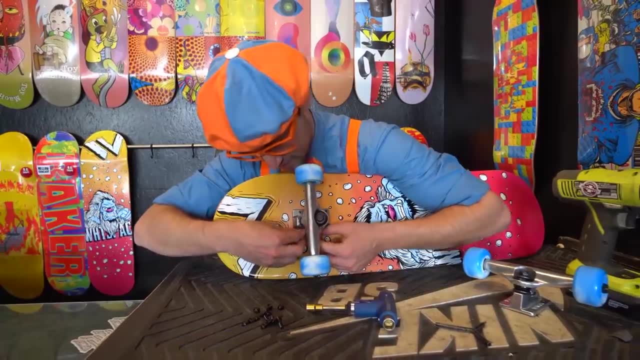 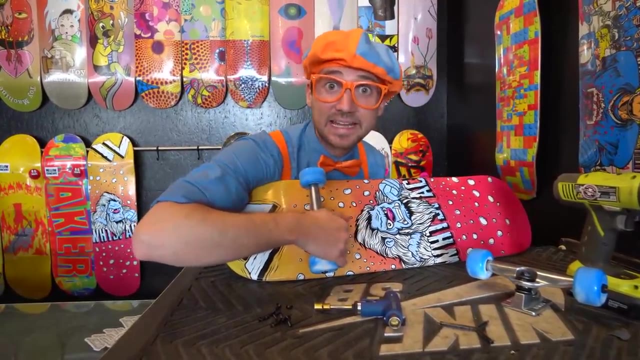 This is just a little tricky, but it's gonna be fun. All right, Let's get this done. Okay, all right, There we go, Alrighty. And then you put some of these right on there And you spin it around. 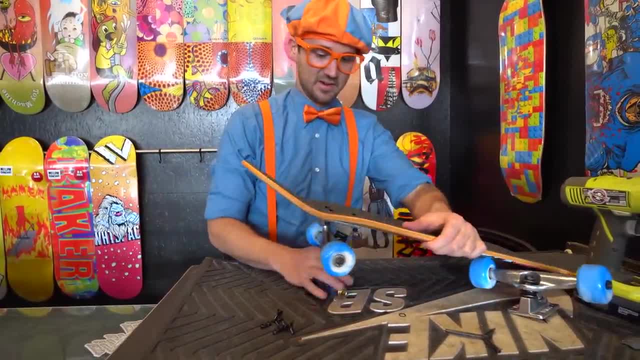 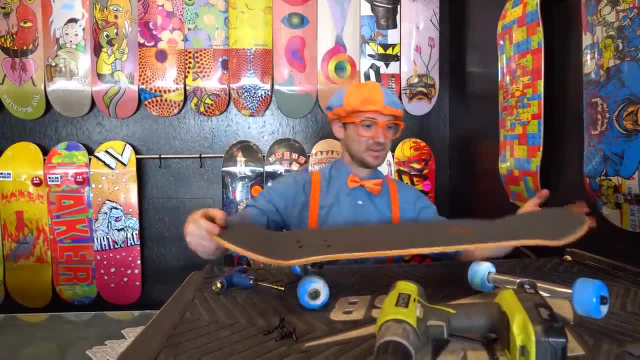 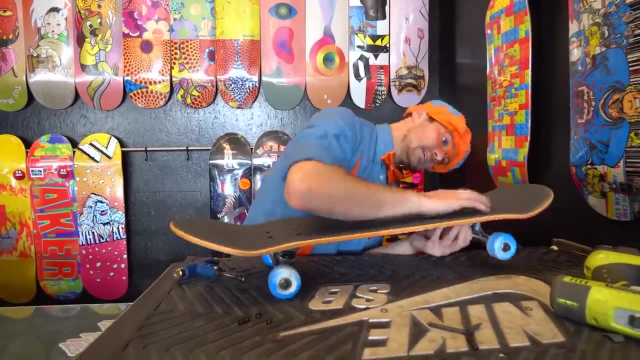 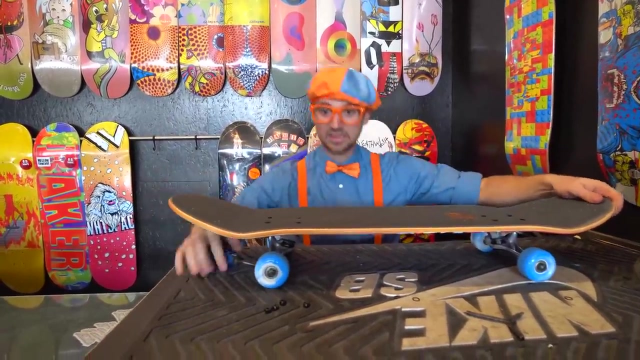 And you make it nice and tight. Okay, watch this. Okay, one of two is done, All right. Oh, there we go, All right. Okay, one of two is done, perfect. and then this other one, and there we go, check it out. it's a completed skateboard. whoa, it's pretty cool, huh. 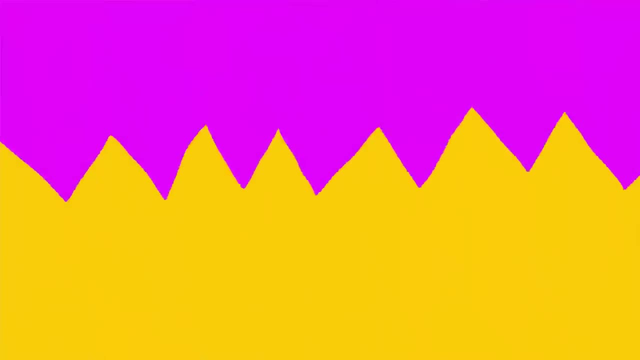 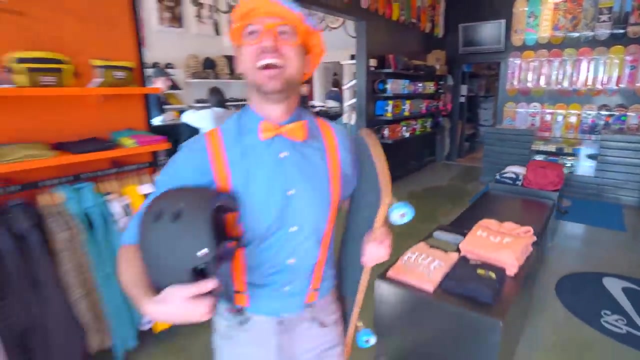 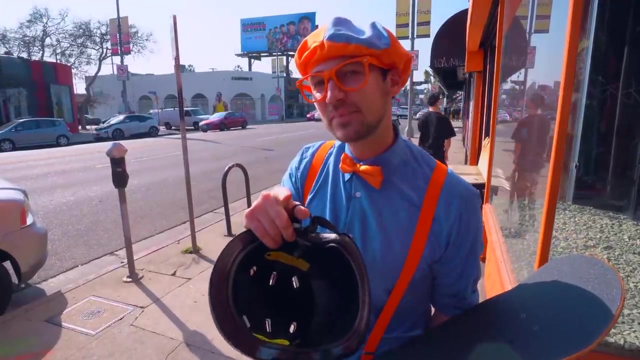 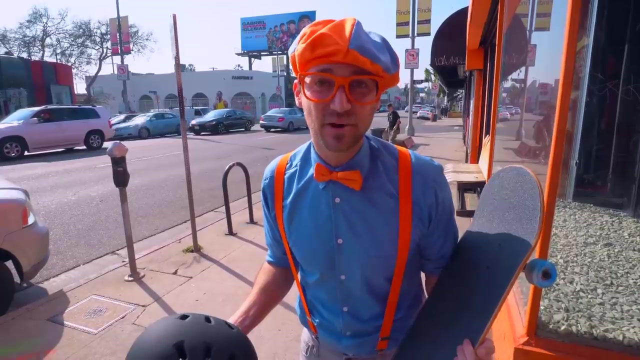 wow, that was so much fun learning about skateboarding with you. if you think skateboarding sounds fun, you should try it, but always remember to wear your helmet and all of your safety equipment. but hey, this is the end of this video, but if you want to watch more of my videos, all 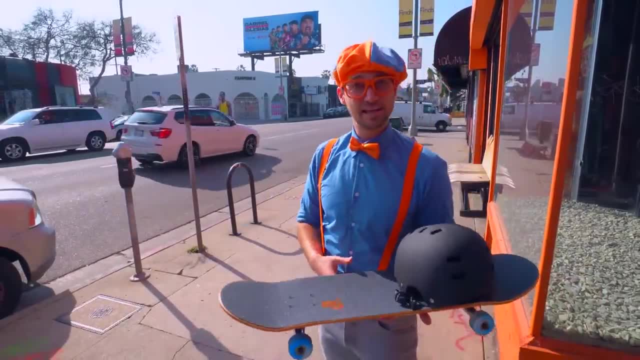 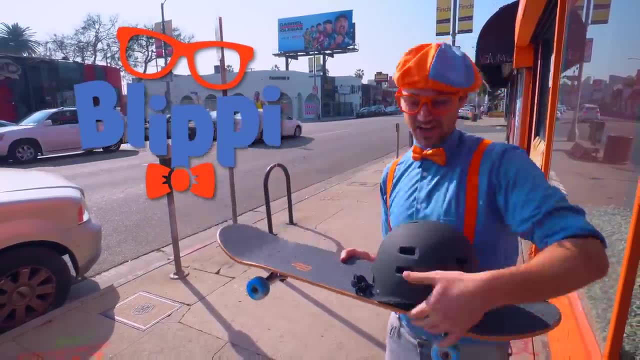 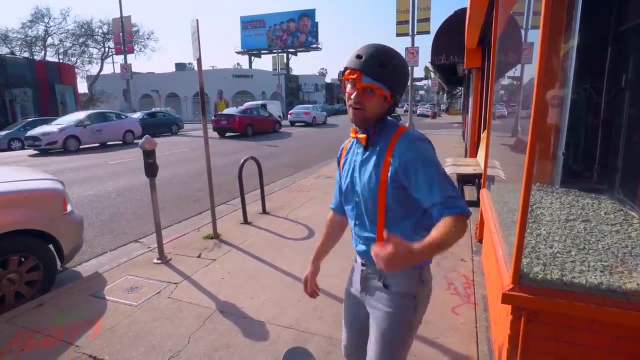 you do is search for my name. Will you spell my name with me? B-L-I-P-P-I Blippi, Good job, All right, Let me put on my helmet. Okay, There we go. Let's go. See you later. 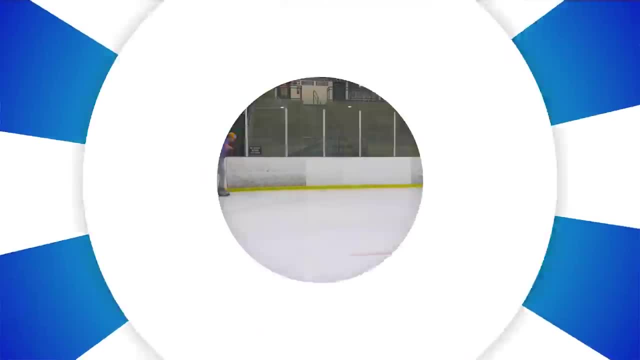 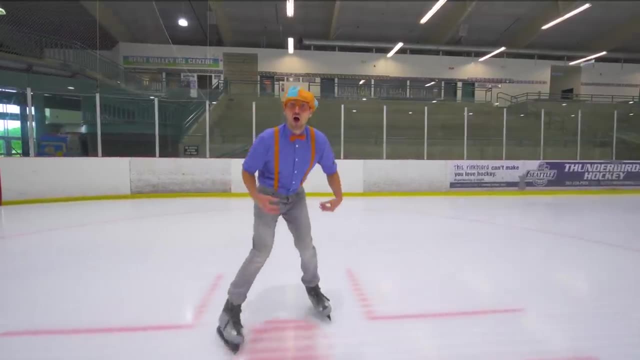 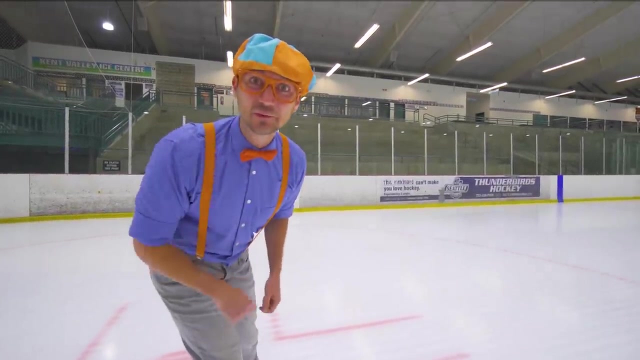 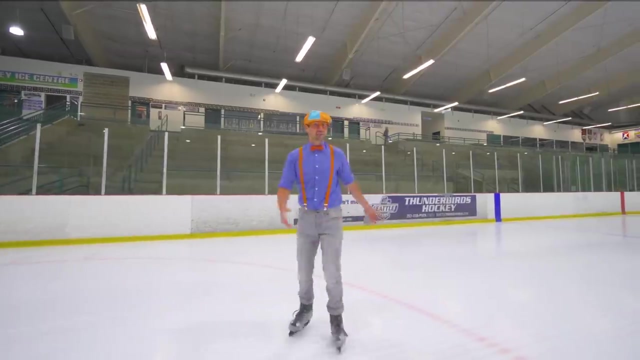 So much to learn about. It'll make you want to shout Blippi. Hey, My name's Blippi. What's your name? Whoa, I really like your name. Look at where I'm at. Whoa, I am at an ice skating rink, And this ice skating rink is the Kent Valley. 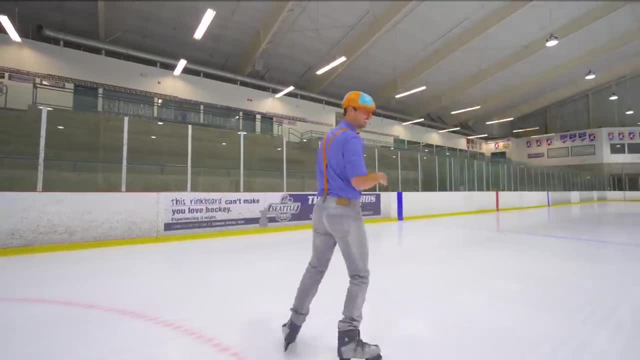 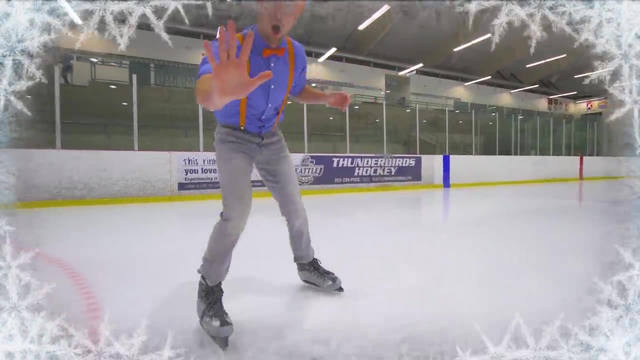 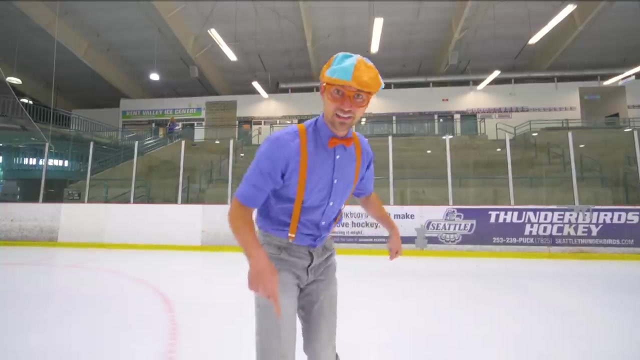 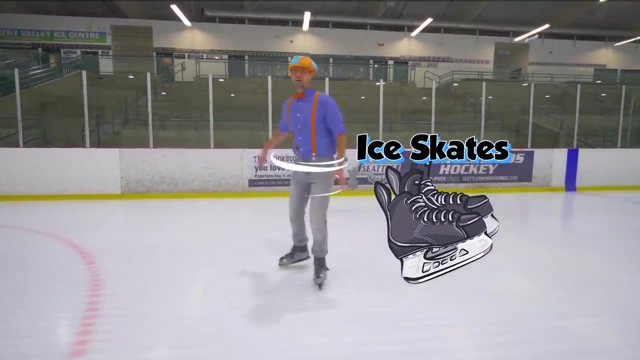 Ice Skating Rink in Kent, Washington. Whoa, The ice is so cold. Whoa, It's really cold, But look at what I'm wearing. Yeah, These are ice skates. Whoa, Look, Whoa. 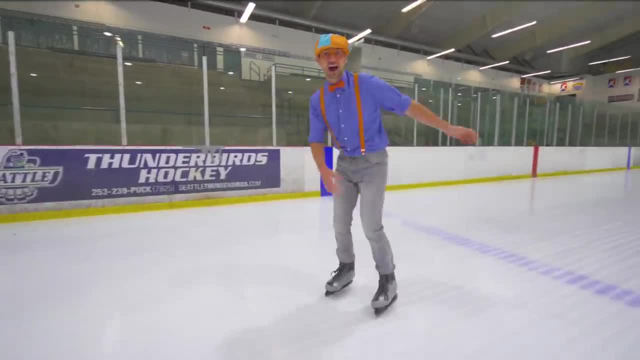 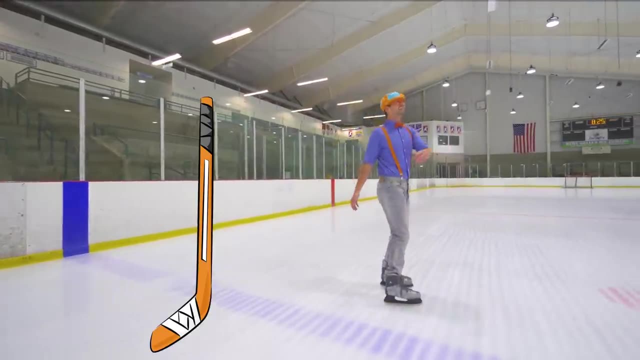 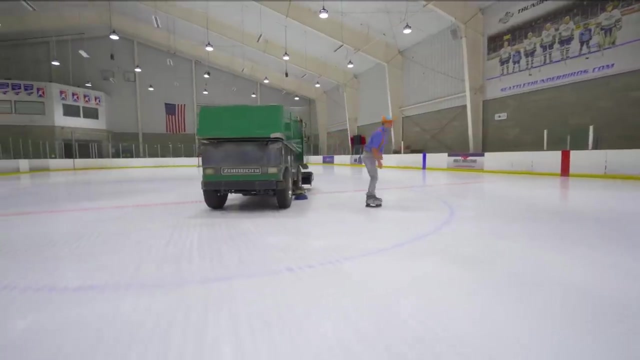 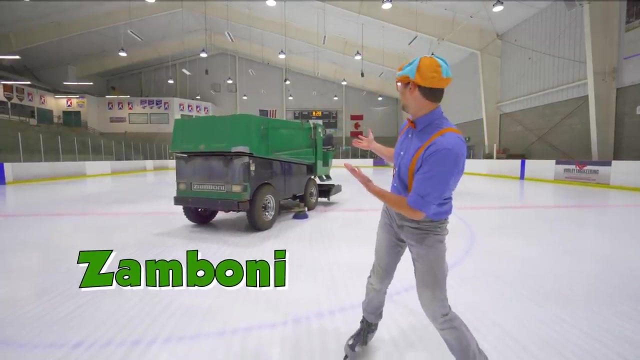 Whoa, I love ice skating rinks because you can ice skate, You can even play hockey. Whoa, What's this? Whoa, This is a Zamboni, And today, you and I are going to learn about Zambonis. 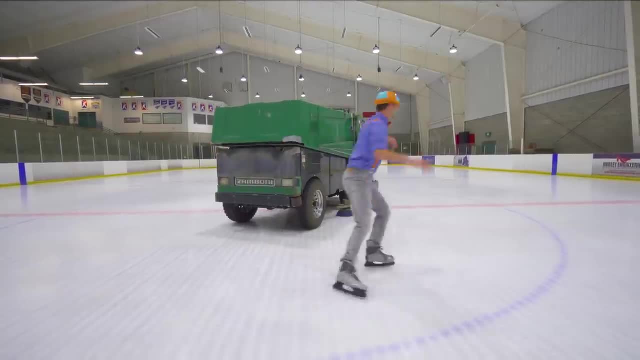 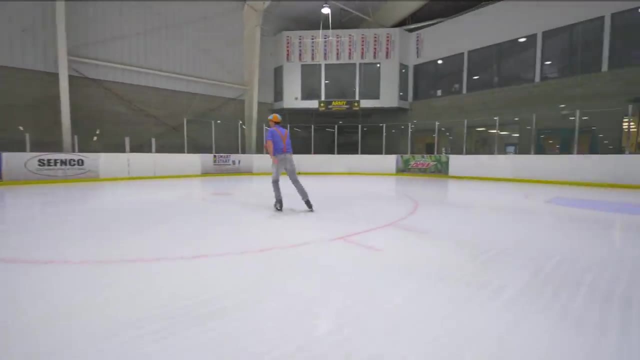 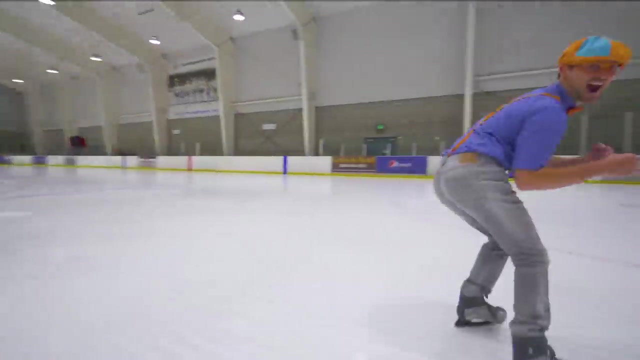 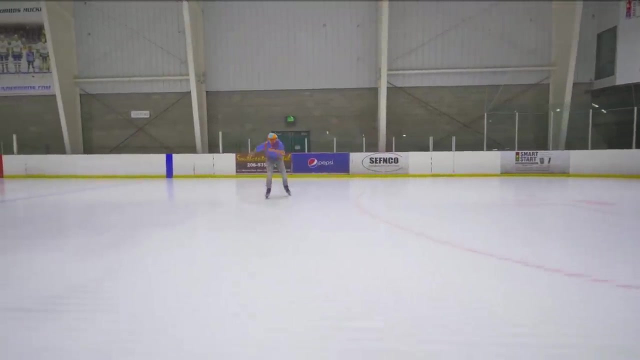 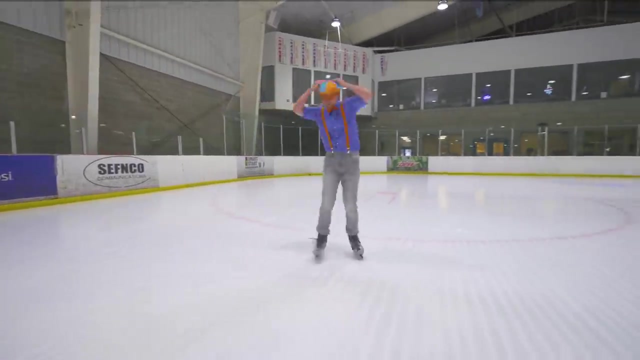 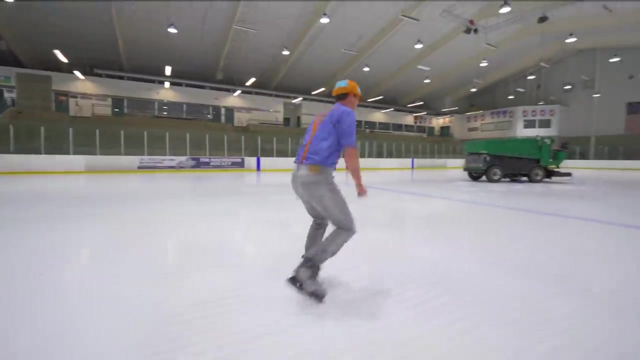 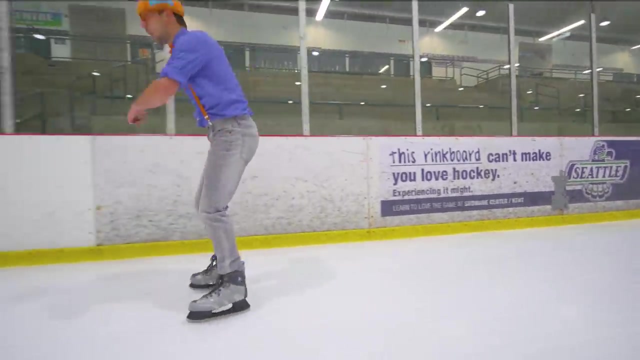 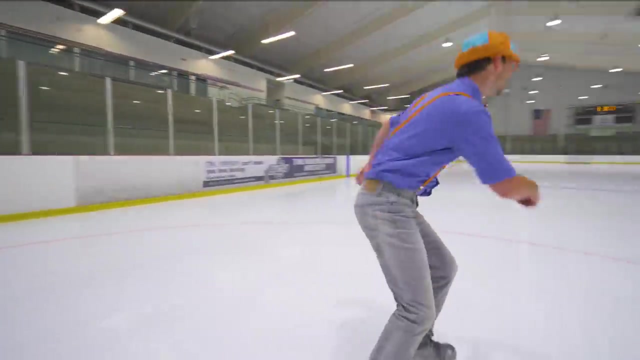 There's a flying supported footprints: Whoa, Whoa, Whoa, Hey, Hey, Hey, Whoa, Hey, Hey. Watch out. Uh, oh, Oh, man sired, Oh, wow, All right, now let's learn a little bit more about the Zamboni. 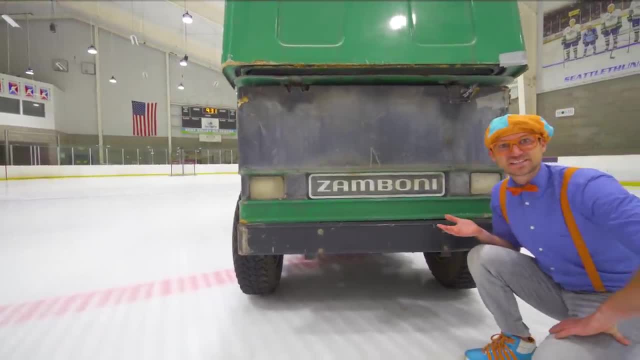 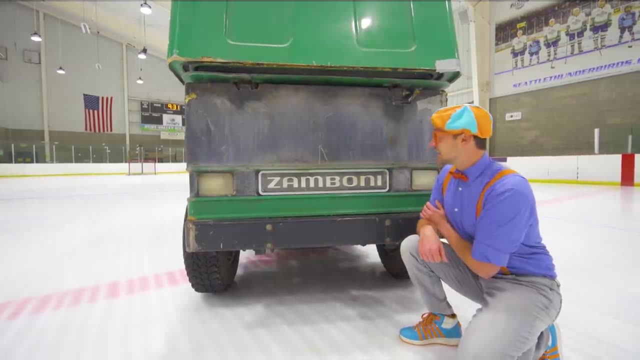 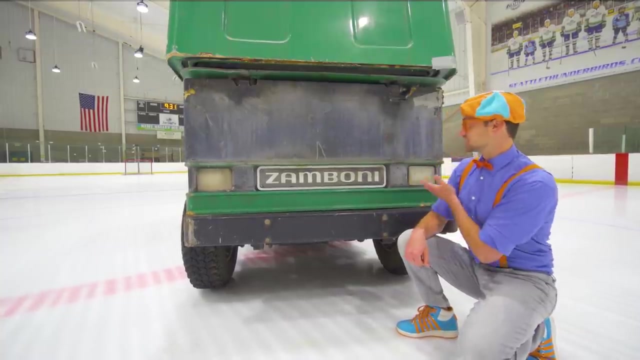 Zamboni- hmm, what a silly name. Look there, it is right there. Let's spell Zamboni together: Ready Z-A-M-B-O-N-I. Zamboni- Whoa, here I go. Whoa. 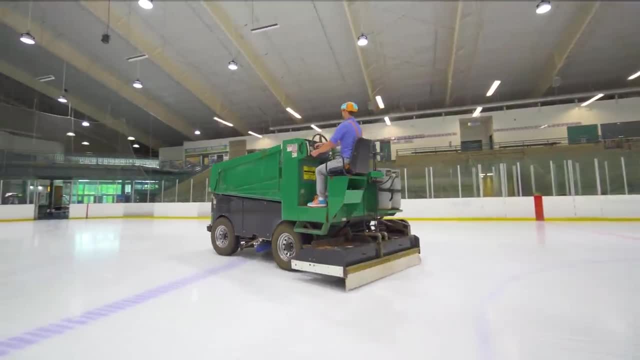 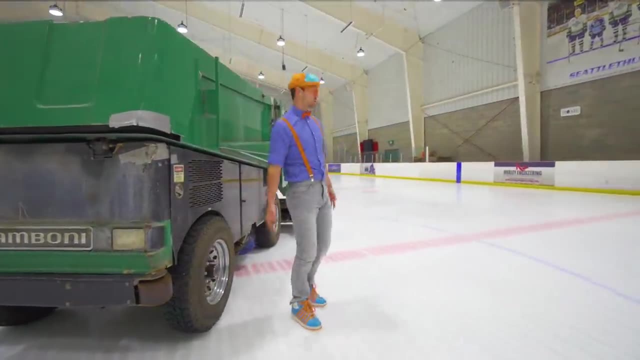 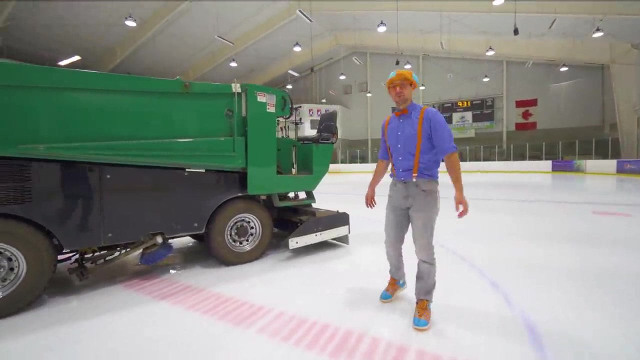 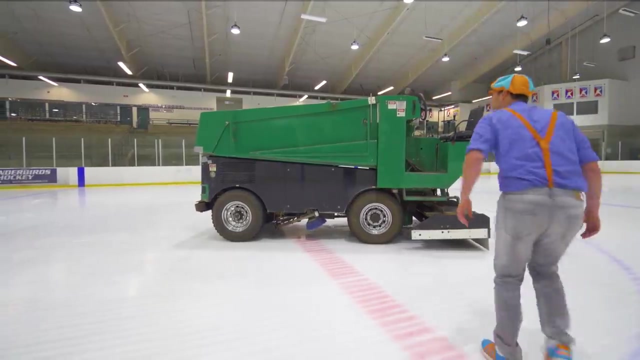 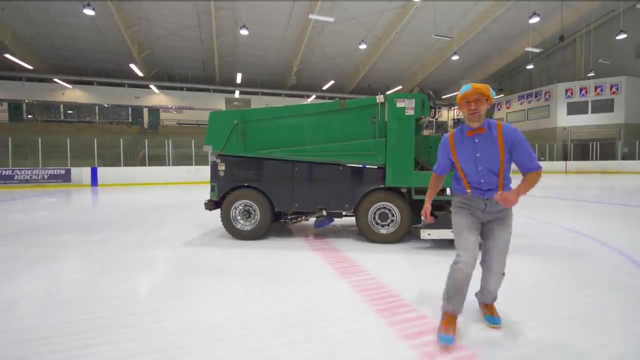 Whoa, Zambonis are used to resurface the ice at the ice rink, the hockey rink. Whoa, what an interesting looking machine. Can you see what shape it looks like? Yeah, it looks like a rectangle. Do you see any other common shapes that Zamboni has on it? 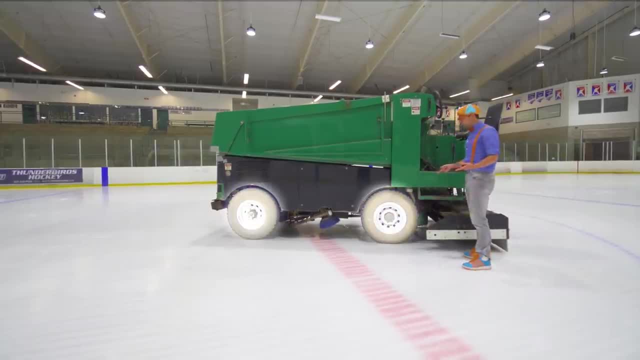 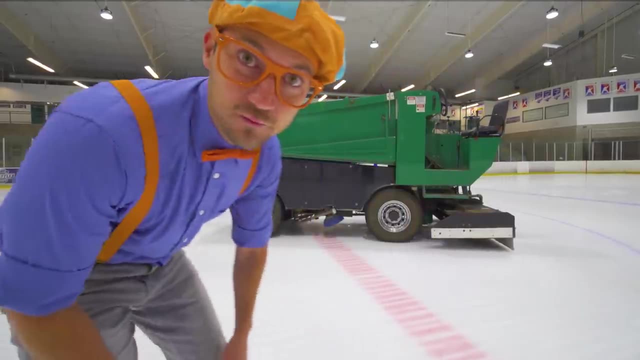 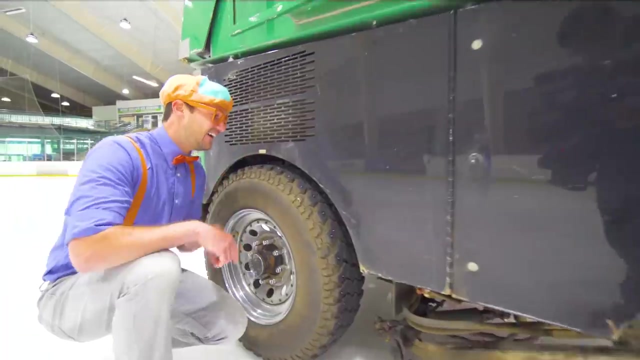 Yeah, The wheels and tires. They are circles. Speaking of wheels and tires, come check them out. Whoa, Looks like those tires have these circles on them. Those are the wheels and tires. Those are the wheels and tires. Those are the wheels and tires. 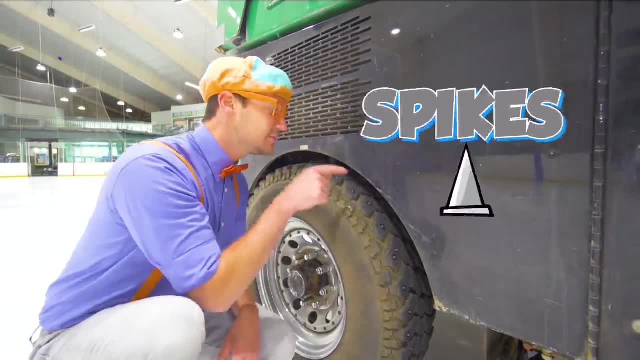 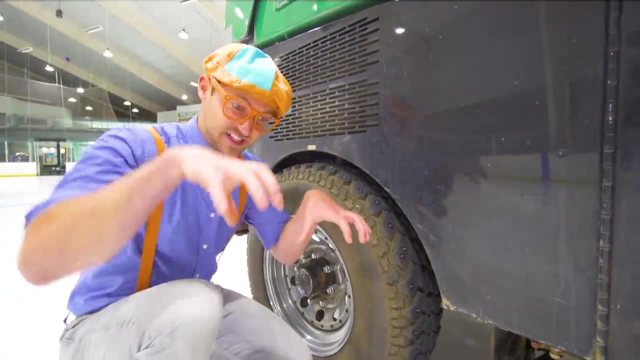 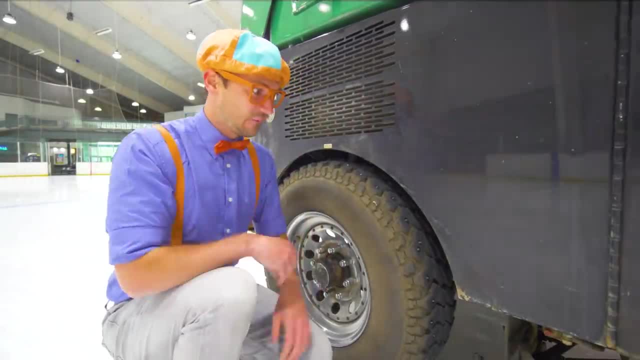 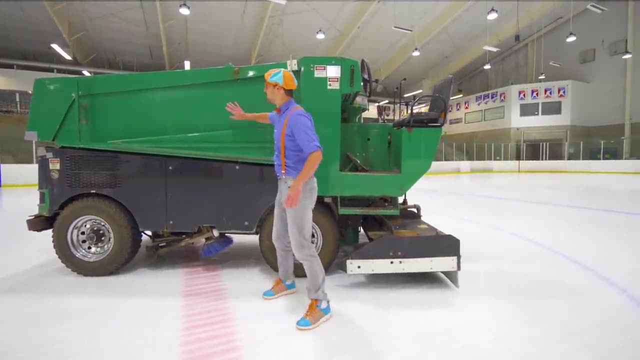 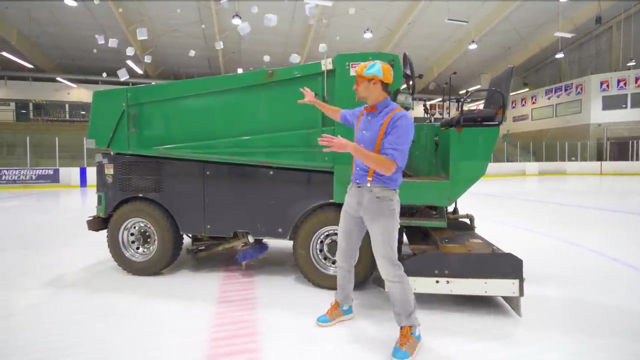 doesn't slip and slide when it drives on the ice. Whoa, All right, let's see what else this Zamboni has. Oh hey, this is the dump tank. When all the ice gets pushed up to the front, this is where all the ice shavings go. 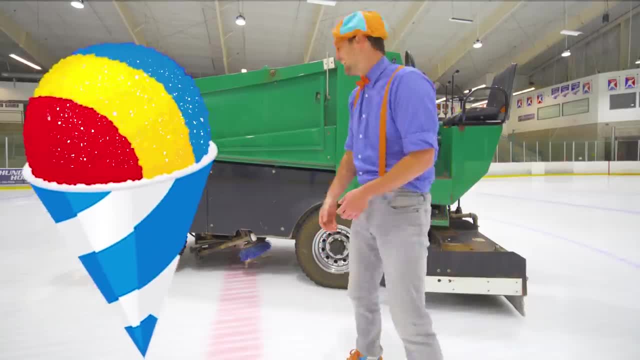 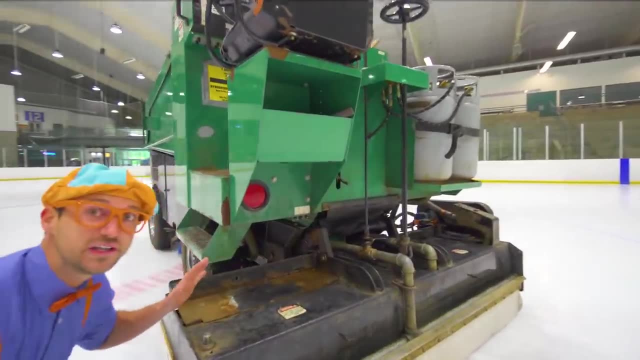 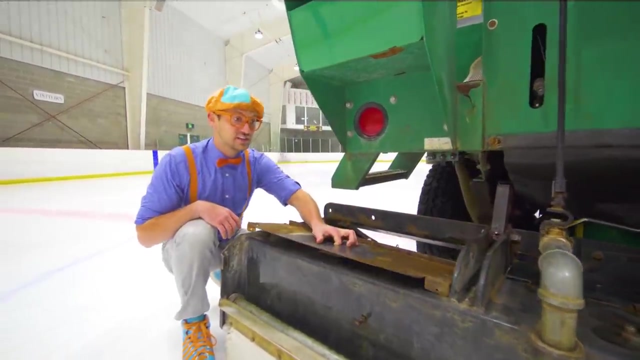 It's kind of like a giant snow cone. All right, come back here. Whoa, This whole unit. this unit is the conditioner, And one cool part of the conditioner is right in here. Whoa, So there's like a razor blade down there. 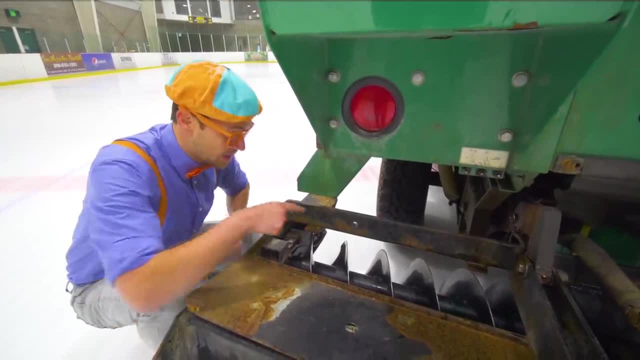 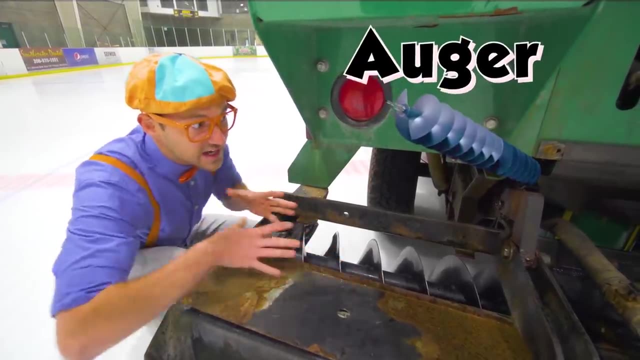 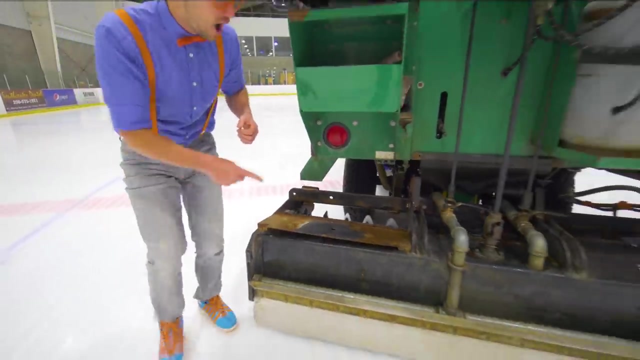 That shaves the ice. it's really hard to see. But this, yeah, it Looks like a spiral. This is an auger that pushes all the ice to the center, then goes to the top, and then goes to the dump tank. And look at this, here's some pipes. 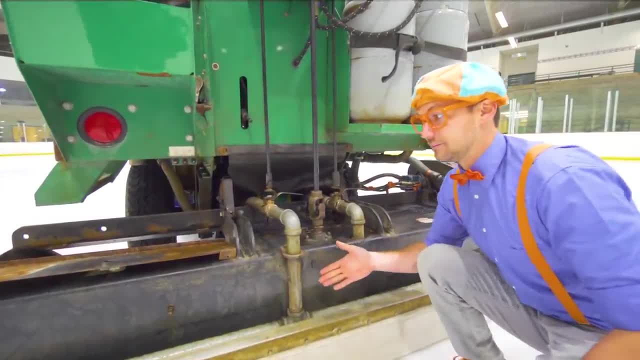 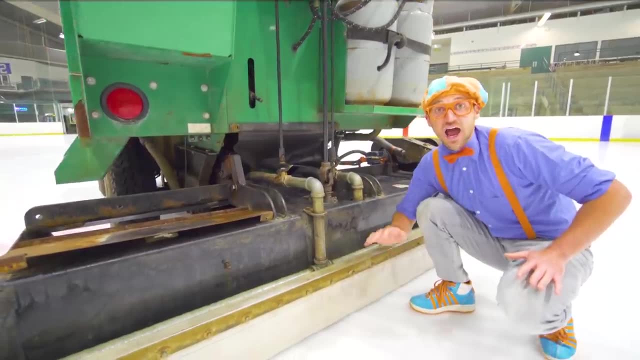 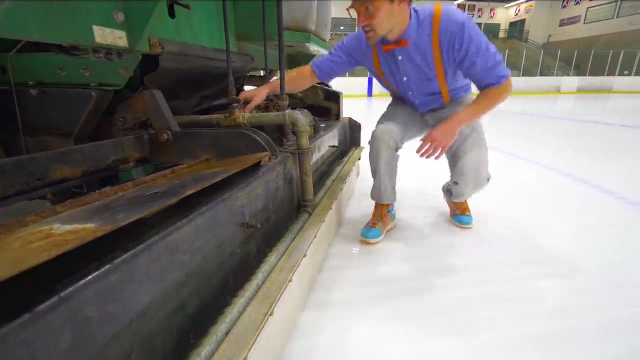 So what? these pipes have have water in them and they spray water up down to the bottom of the ground, left to the right, and then from there the water goes on the ice and then it melts and makes it really smooth and flat. okay, watch this. 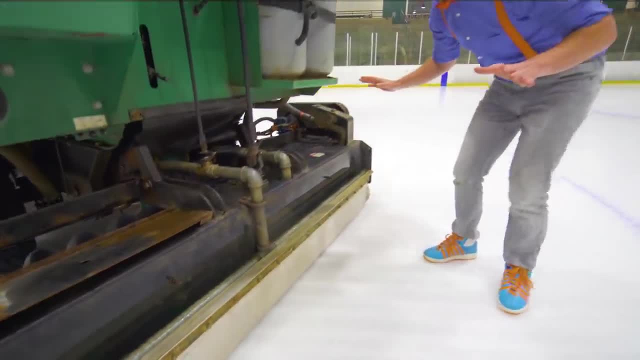 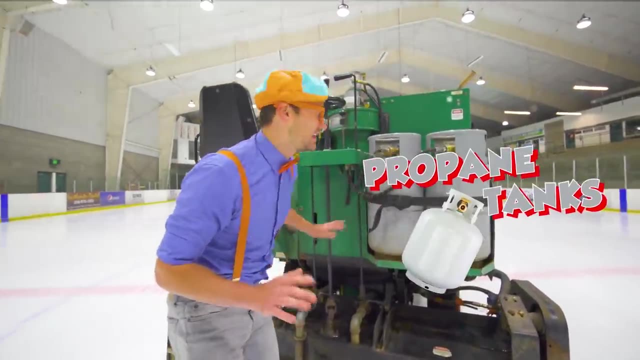 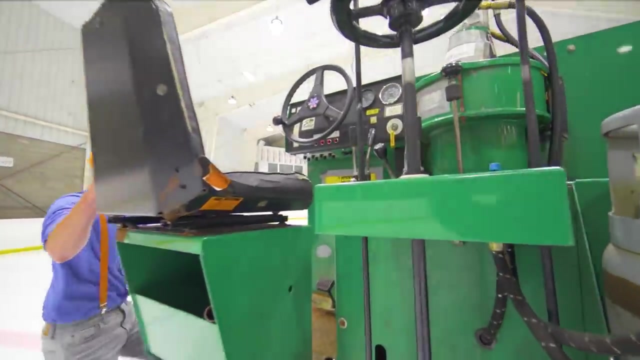 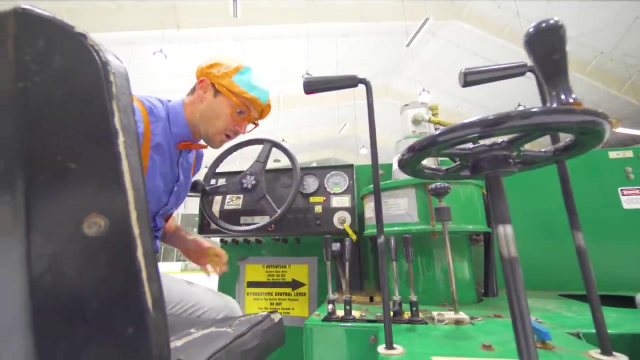 whoa, okay, all right. all right, I think it's time to turn on the Zamboni. see these? these are propane tanks. this is what powers the Zamboni. all right, let's fire it up. turn on the key? whoa, all right, check this out. 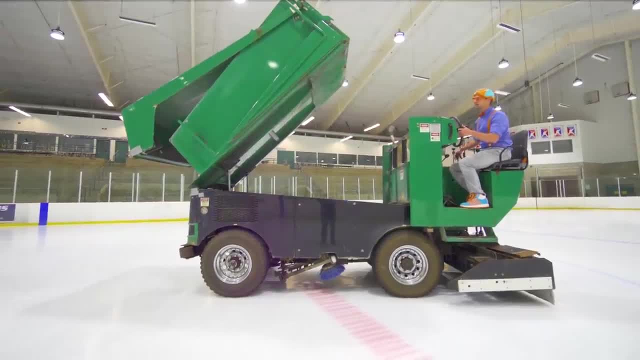 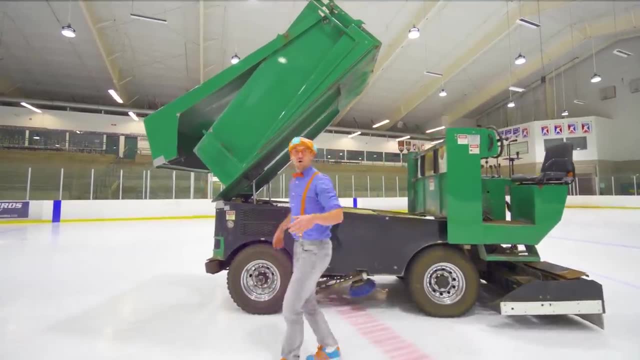 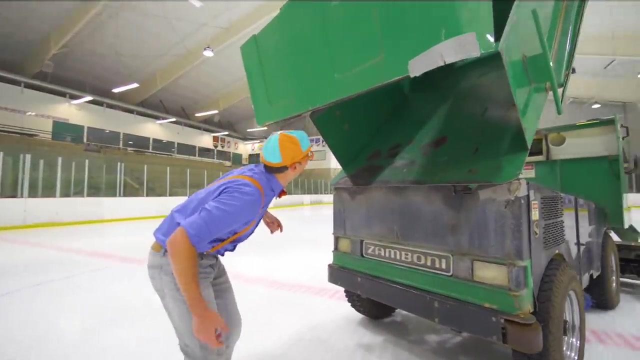 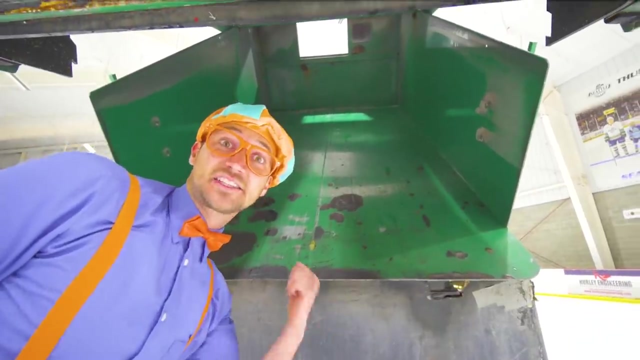 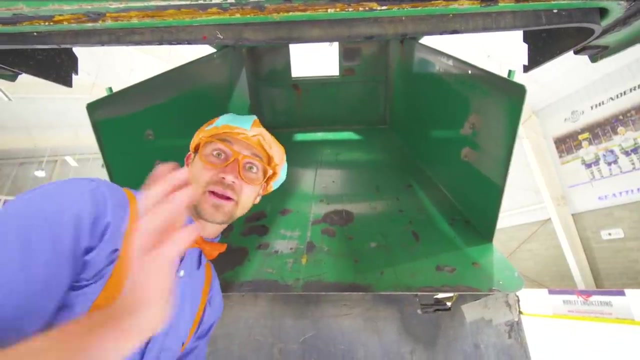 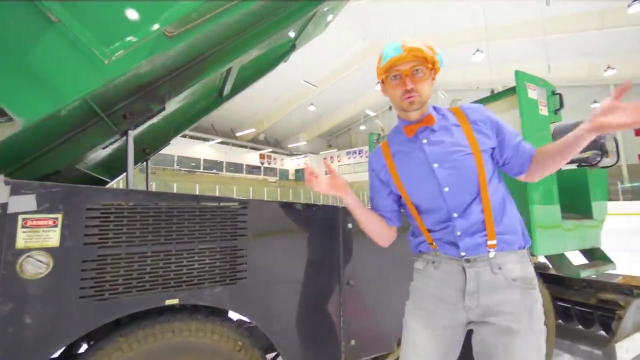 whoa, all right, check this out really loud. but that's the dump tank, that's where all the ice goes, and then you dump it into the ice bin, and then you dump it into the ice bin and then the back. okay, but come over here. it's really loud because that is the motor. 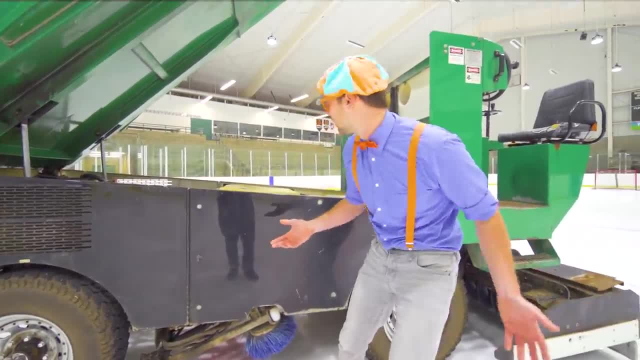 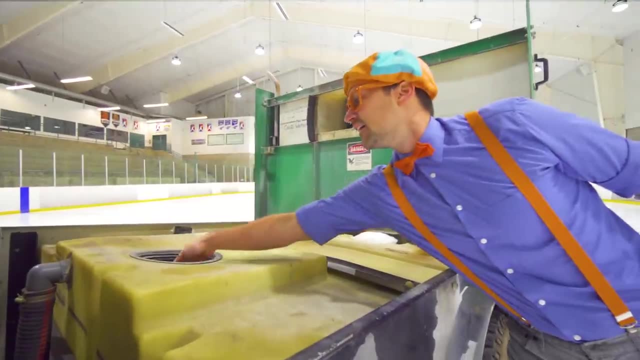 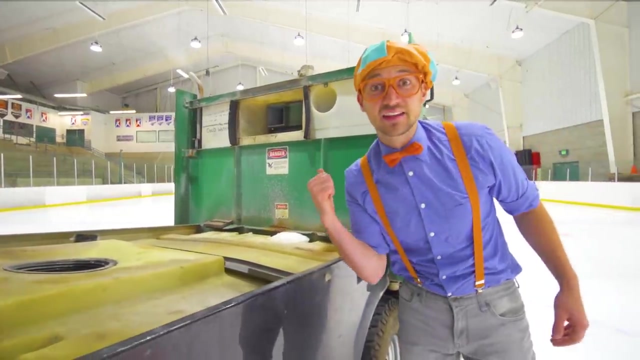 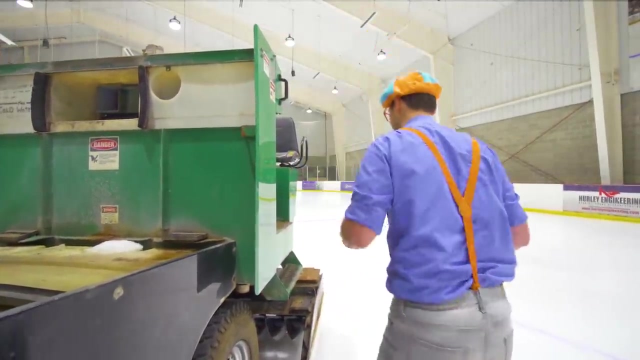 that's what provides the Zamboni with all of its power. ooh and right here, this is the water tank. that's where the back of the Zamboni gets all of its water from. all right, I'm gonna go resurface the ice rink. 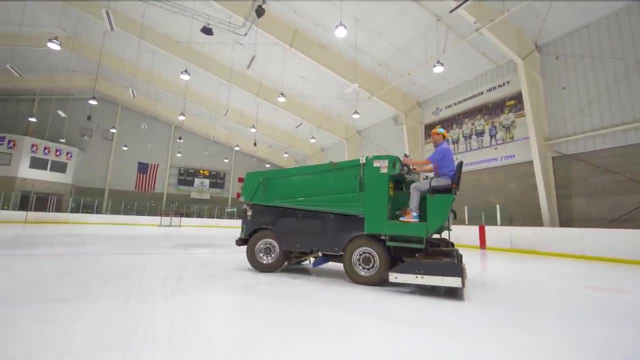 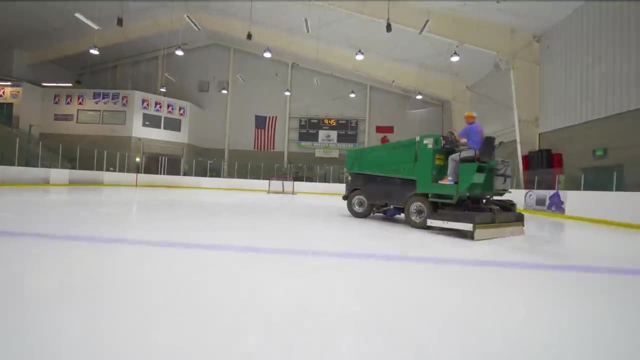 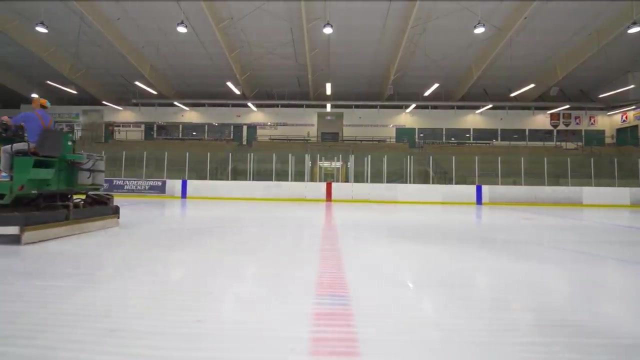 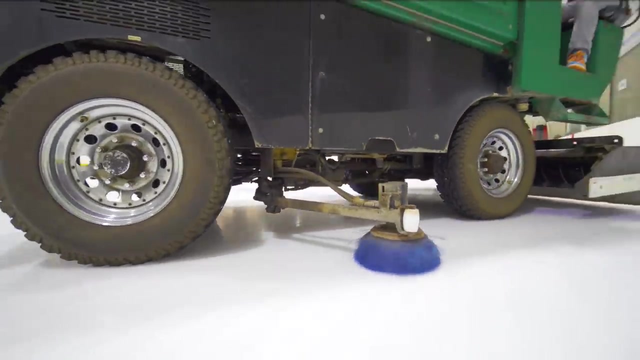 you gonna do that, all right, and there we go. as I just told you, I love being stopped here, you know. you ask yourself: can you talk me through the doors? why isn't the chosen seat coming up? okay, I'm gonna get on the Champion Team, whoa. 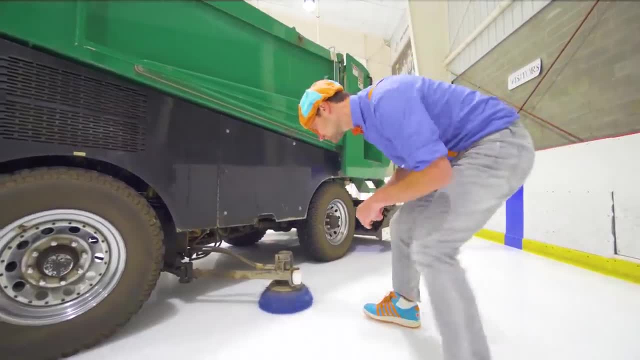 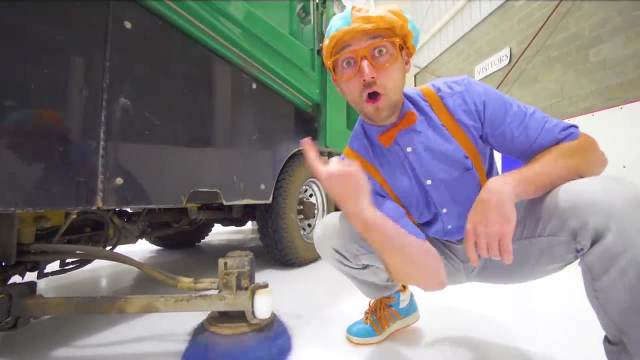 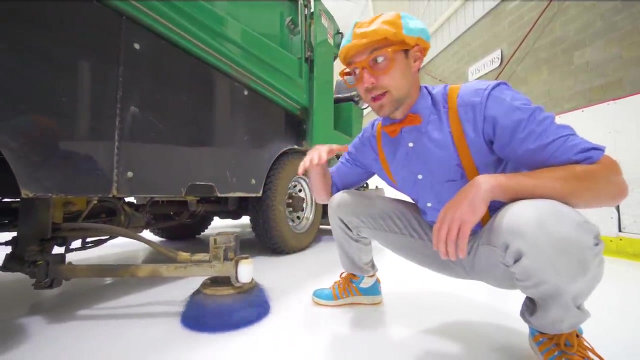 man, oh, oh, you see that, look at me run. you see me short. brothers said: come on, baby, so I'll follow you, face of the board all around the ice rink and pushes all of everything in the middle for the augers and the blades to then get push the top to the forward and then you can recondition the ice. 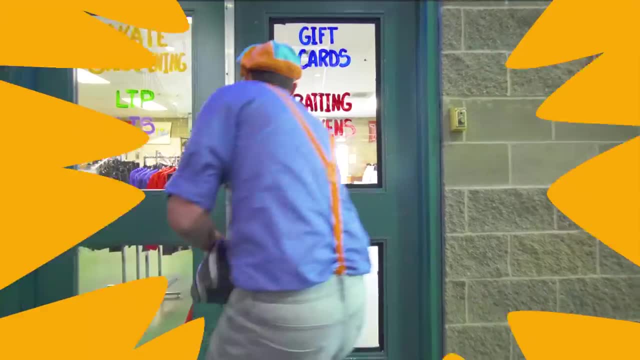 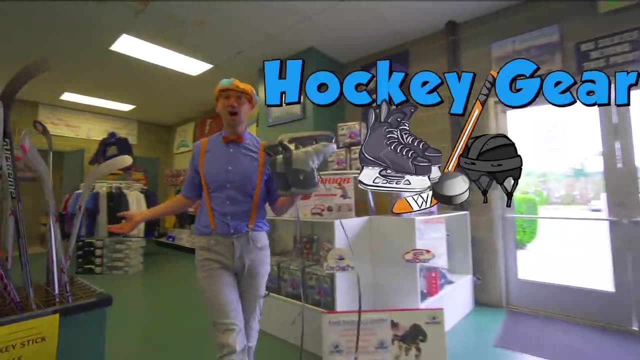 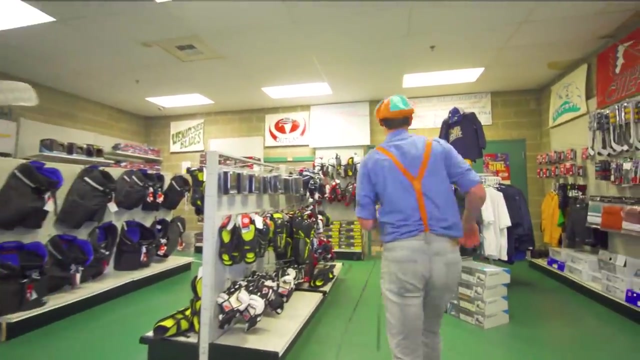 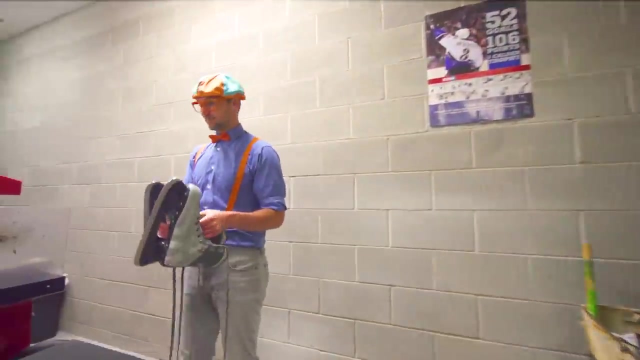 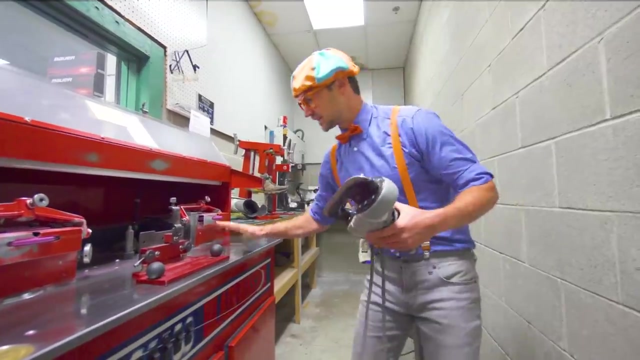 wow, board brush- whoa, this is the pro shop. this is where you get all of your hockey gear- whoa, hockey sticks- so cool. all right, we'll look at those later, but right now, we need to sharpen my blades on my skates. all right, and this is the sharpening room. wow, so cool. all right, this is the. 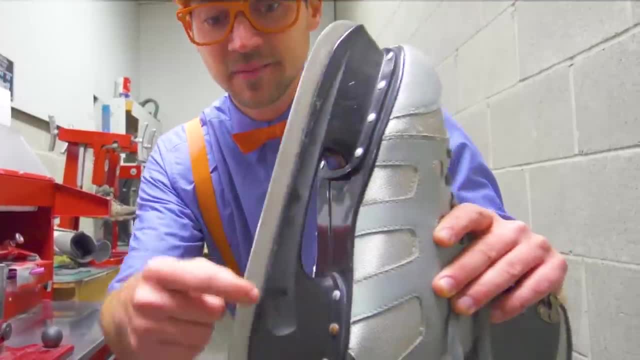 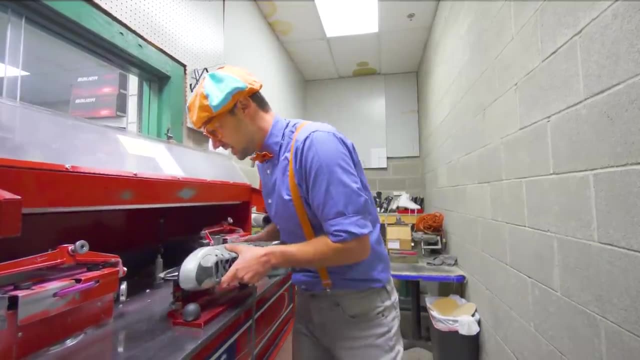 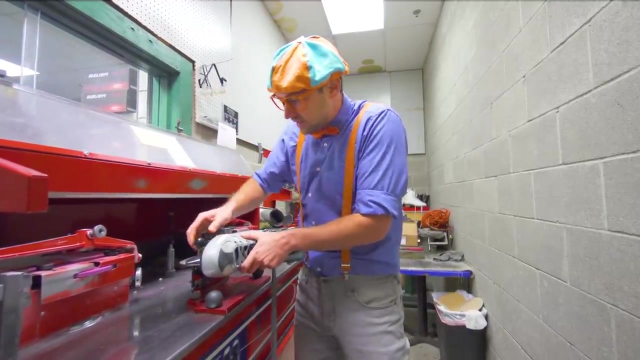 blade master. yeah, see this. there's metal on the bottom of this skate and we need to sharpen it. this is the sharpening station, so let's put the skate right here, slide this, tighten that just a little bit, pull that up. now it's ready to sharpen. 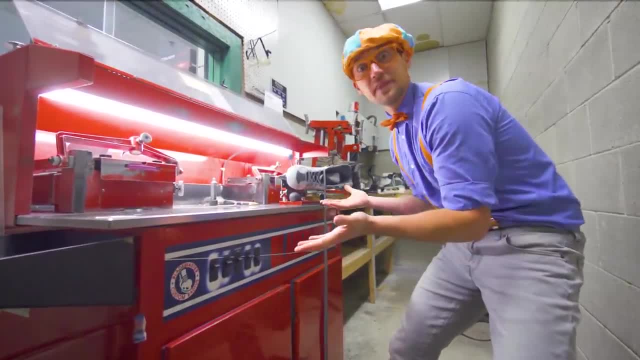 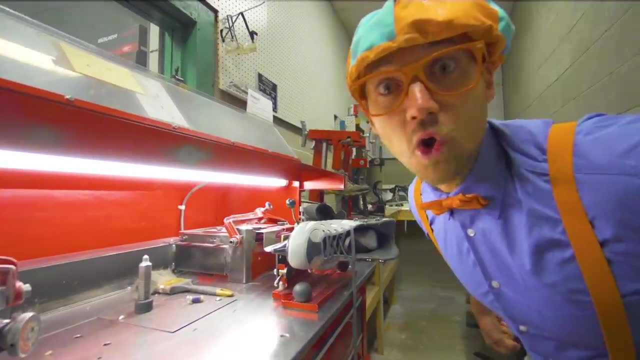 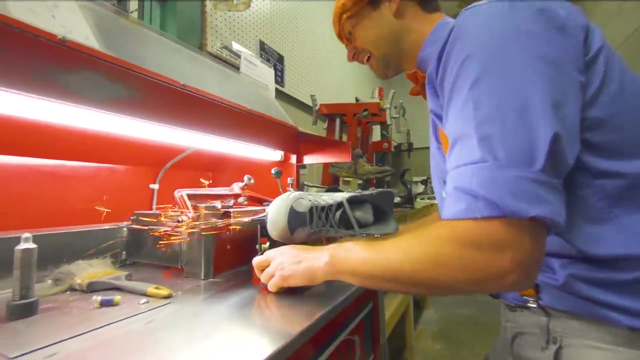 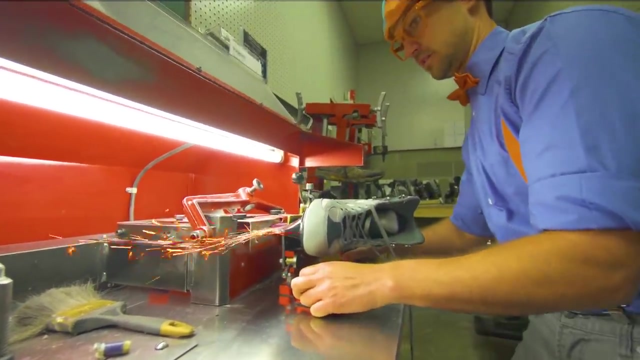 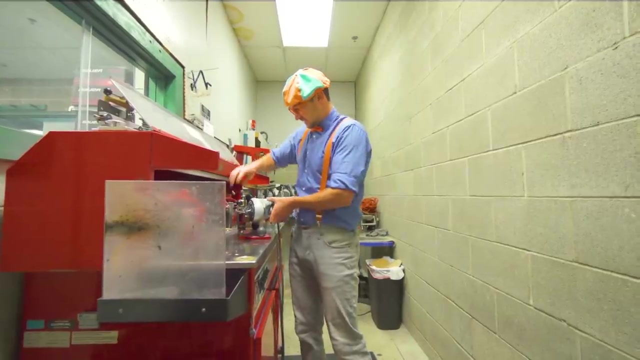 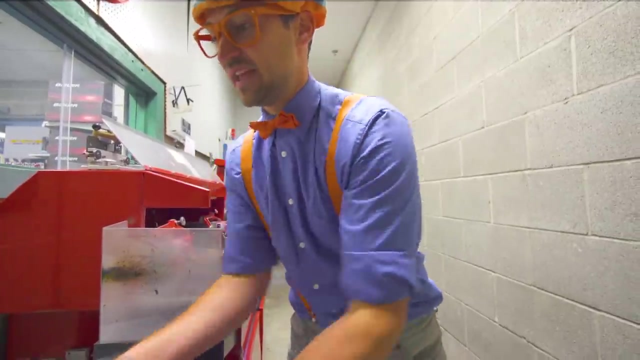 okay, turn on the light. and then there was light. all right, here we go. oh, do you see those sparks? here we go. whoa, all right, ah, that's sharp. all right, now we're ready. all right, let's go check out some hockey gear. all right, let's go check out some hockey gear. 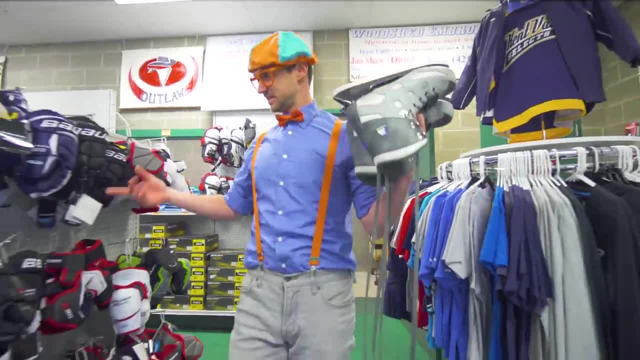 let's go check out some hockey gear. let's go check out some hockey gear. oh, some pads, yeah, a lot of pads. oh, some pads, yeah, a lot of pads, because ice is really hard. you don't want to. because ice is really hard, you don't want to. 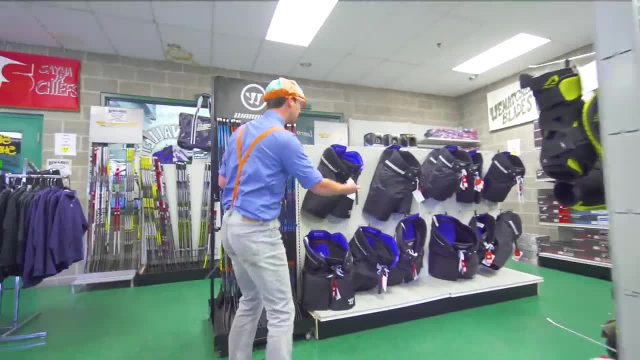 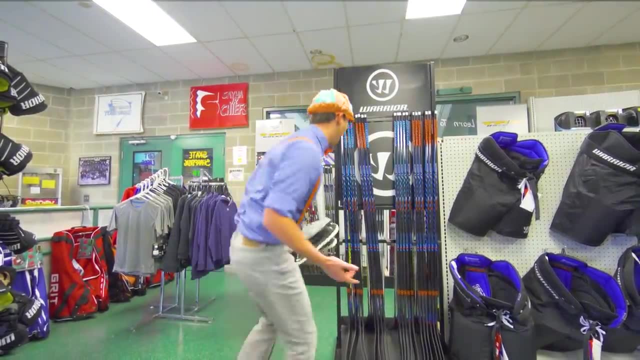 because ice is really hard. you don't want to fall down. fall down. some more pads. do you see what i see? some more pads. do you see what i see? some more pads. do you see what i see? orange and blue hockey sticks. orange and blue hockey sticks. 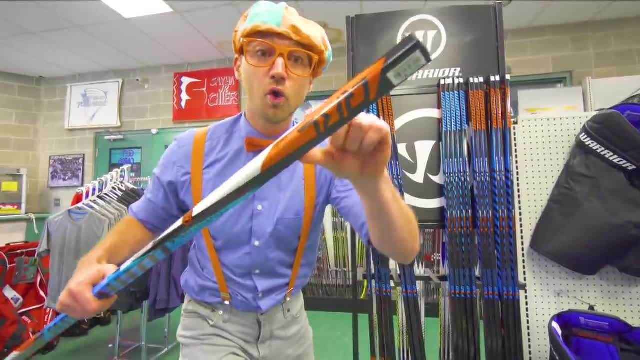 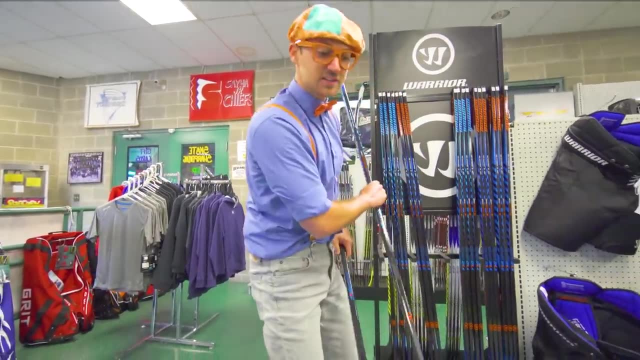 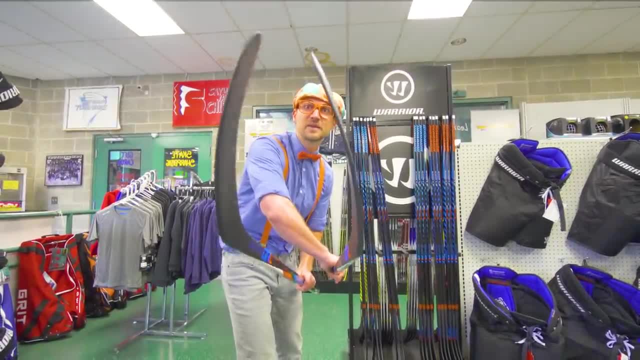 here's two different kinds of hockey. here's two different kinds of hockey sticks, sticks, sticks. do you see how they curve differently? do you see how they curve differently? do you see how they curve differently? see this one curves that way. see this one curves that way. see this one curves that way and this one curves that way. 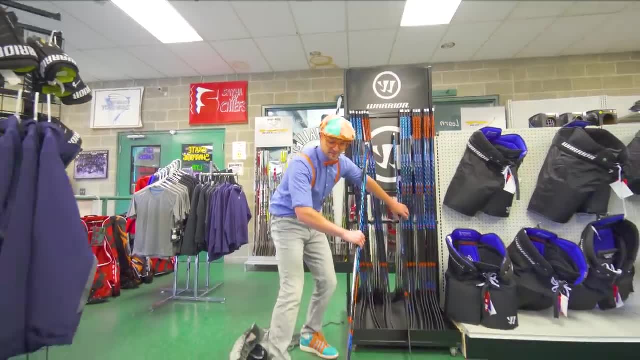 and this one curves that way and this one curves that way. wow see, i'll give you an example. wow see, i'll give you an example. wow see, i'll give you an example. so you take this one and you fling the. so you take this one and you fling the. 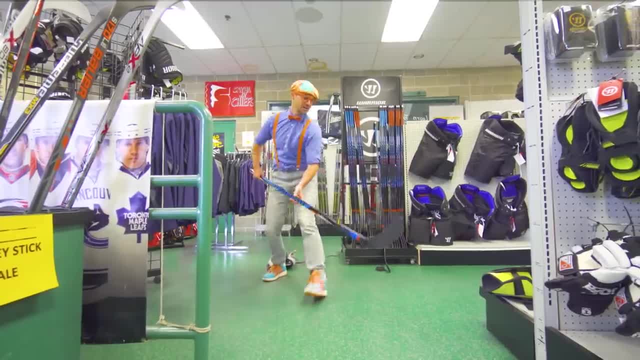 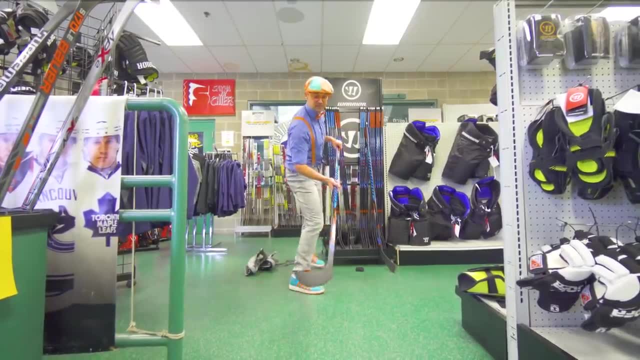 so you take this one and you fling the puck this way, puck this way, puck this way, because it curves that way. but this one, it curves the other way, so you it curves the other way. so you it curves the other way, so you fling the puck that way. 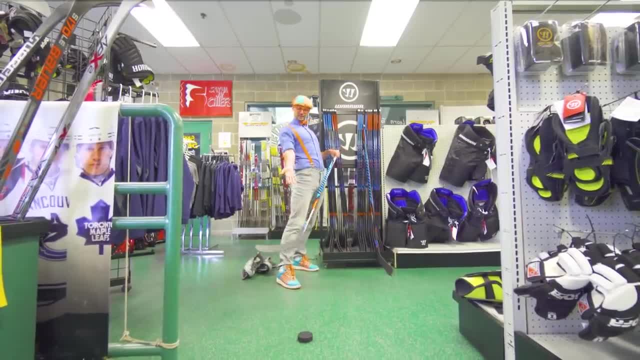 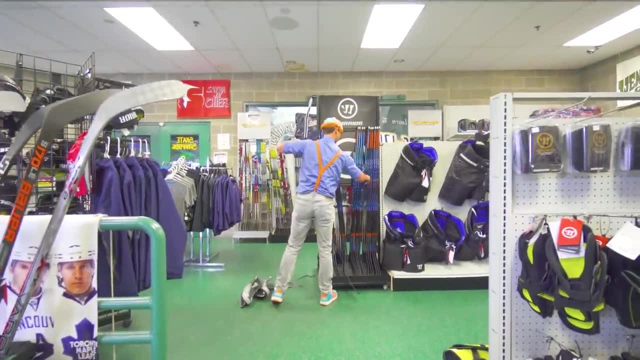 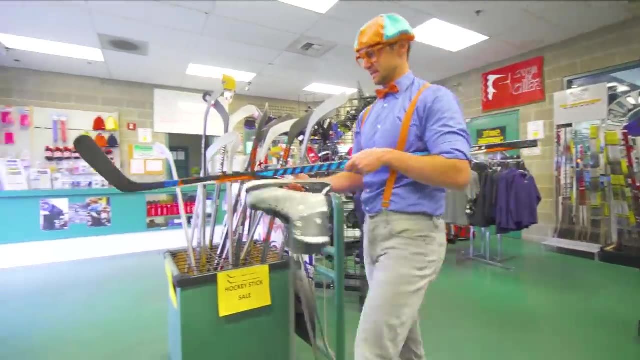 fling the puck that way, fling the puck that way. oh hey, look a perfectly placed. oh hey, look a perfectly placed. oh hey, look a perfectly placed. hockey puck, hockey puck, hockey puck. all right, okay, all right, okay, all right, okay. i got the perfect stick, i got my skates and 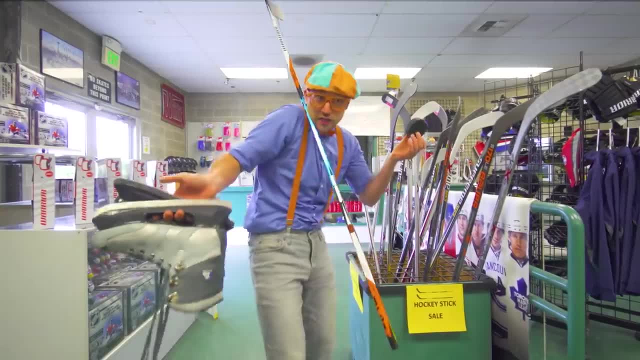 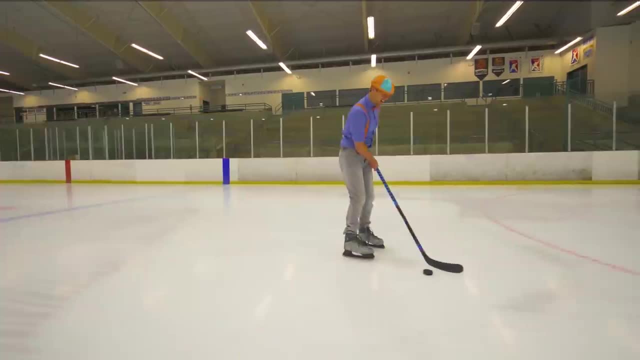 i got my skates. and i got my skates and i got the hockey puck. so now i got the hockey puck. so now i got the hockey puck. so now let's go play some hockey. let's go play some hockey. let's go play some hockey. 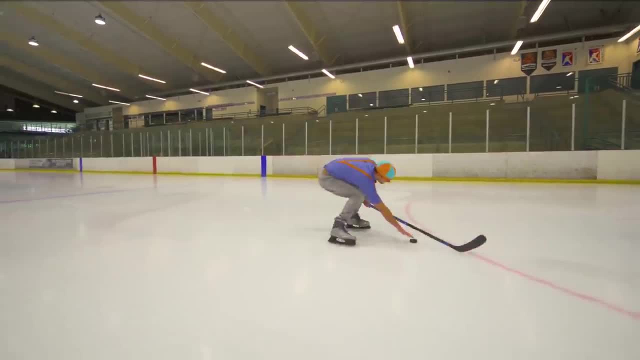 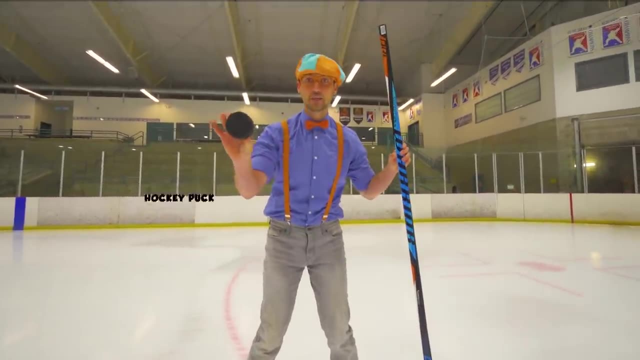 whoa, whoa, whoa. all right, all right, all right, now that we have our hockey stick, now that we have our hockey stick, now that we have our hockey stick and our hockey puck- another fun thing to- and our hockey puck. another fun thing to- and our hockey puck. another fun thing to do at ice skating rinks is learn to. 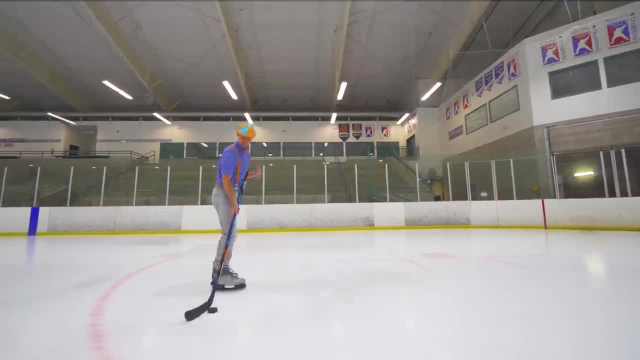 do at ice skating rinks is learn to do at ice skating rinks is learn to play, play, play, and maybe at your ice skating rink, they, and maybe at your ice skating rink, they, and maybe at your ice skating rink, they have learned to play as well, where you. 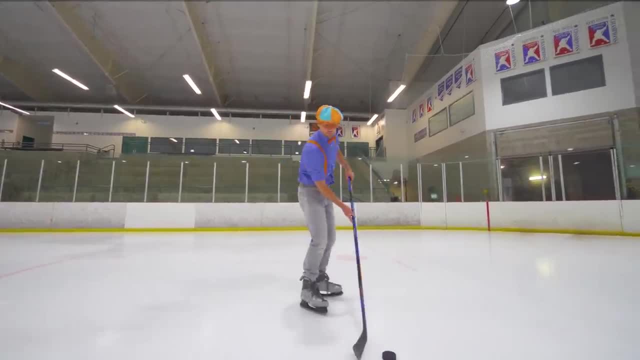 have learned to play as well, where you have learned to play as well, where you, as a child, can learn to play hockey and, as a child, can learn to play hockey and, as a child, can learn to play hockey. and the point of hockey is to get the puck. 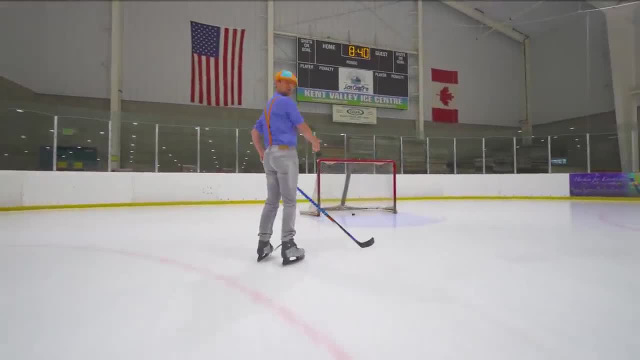 the point of hockey is to get the puck. the point of hockey is to get the puck using the stick, into using the stick, into using the stick, into the hockey goal. the hockey goal, the hockey goal. whoa, whoa, whoa, check it out, check it out. 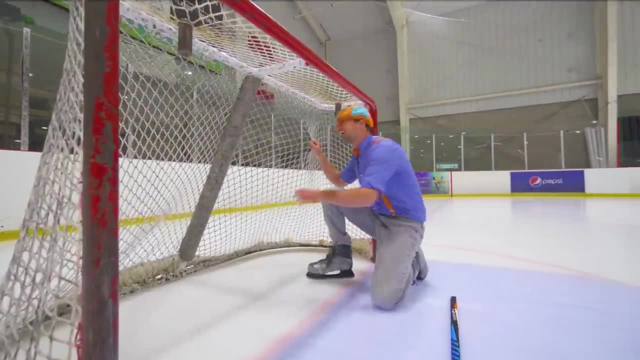 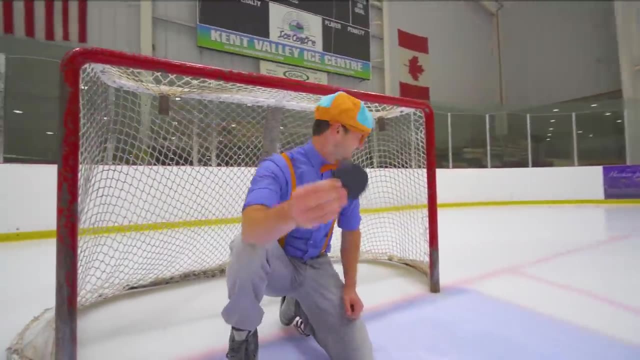 check it out. this, this, this is the goal- is the goal, is the goal? whoa, whoa, whoa, whoa, whoa, whoa. so what you do like i said, take the puck. so what you do like i said, take the puck. so what you do like i said, take the puck and get it inside the hockey goal past. 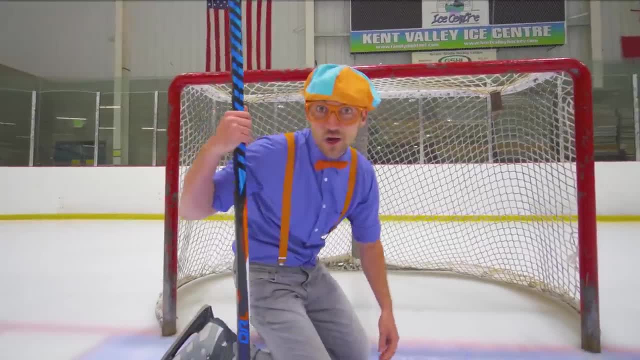 and get it inside the hockey goal past and get it inside the hockey goal past this line with the hockey stick, this line with the hockey stick, this line with the hockey stick. all right, let's try it again. all right, let's try it again. all right, let's try it again. it's gonna be a little bit easier because. 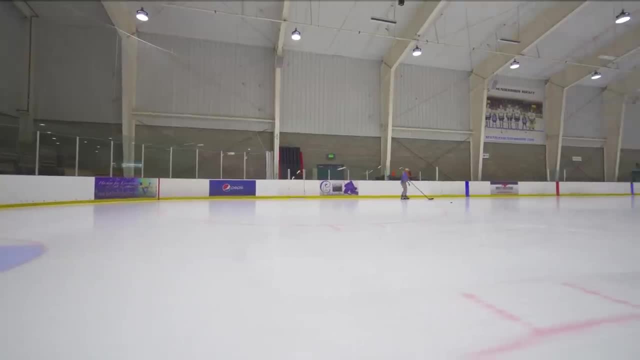 it's gonna be a little bit easier. because it's gonna be a little bit easier because normally there's a goalie right there. normally there's a goalie right there. normally there's a goalie right there. it's so much fun playing hockey. it's so much fun playing hockey. 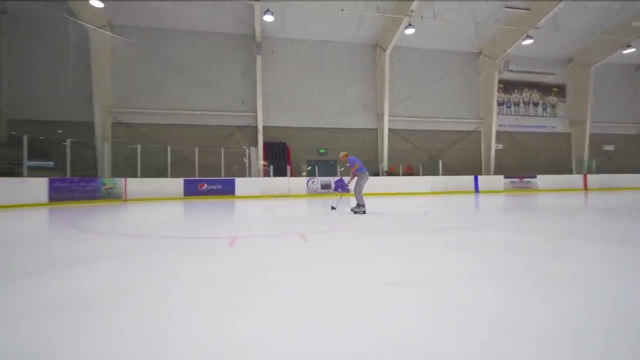 it's so much fun playing hockey because the puck slides on the ice, just because the puck slides on the ice, just because the puck slides on the ice, just like my skates, like my skates, like my skates. oh i miss, oh i miss, oh i miss. that's okay. 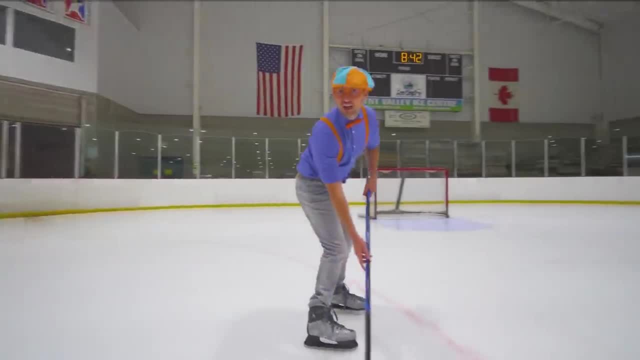 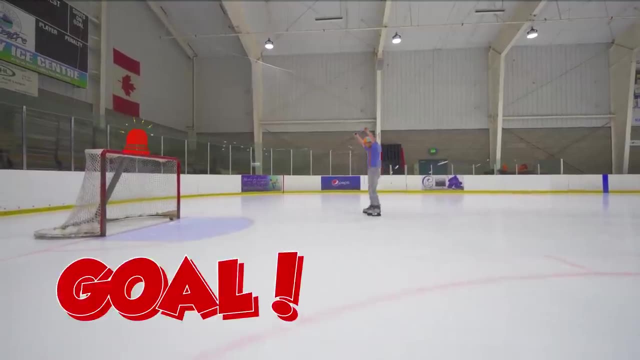 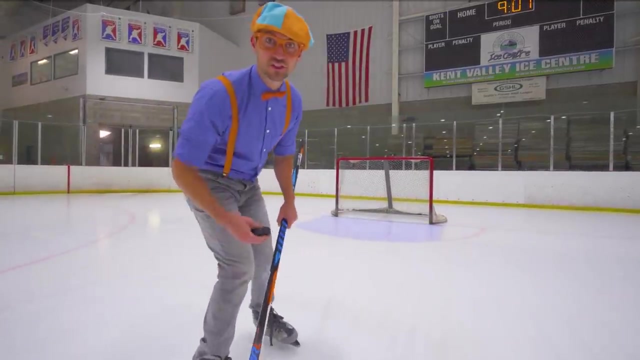 that's okay. that's okay because when you play sports, if you miss, because when you play sports, if you miss, because when you play sports, if you miss, you just have to try again like this and eventually you'll win and eventually you'll win and eventually you'll win. this right here is a specialty move. it's 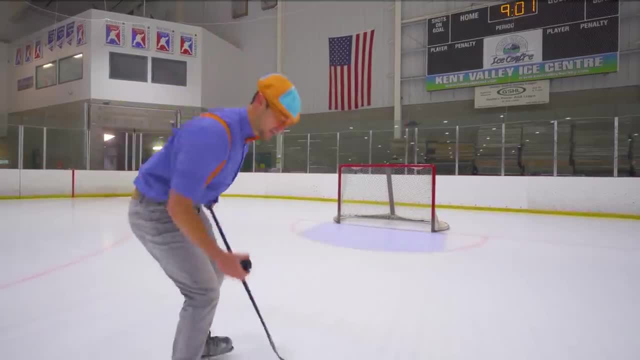 this right here is a specialty move. it's this right here is a specialty move. it's called a knuckle puck, called a knuckle puck, called a knuckle puck. you take the puck, you take the puck. you take the puck, put it down vertically, like that. 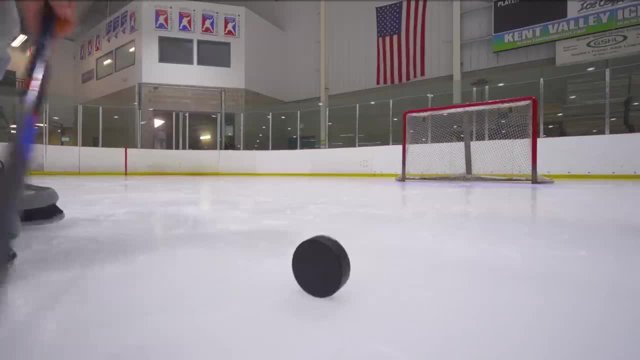 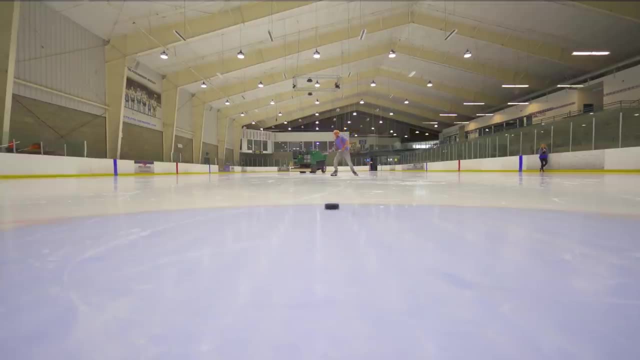 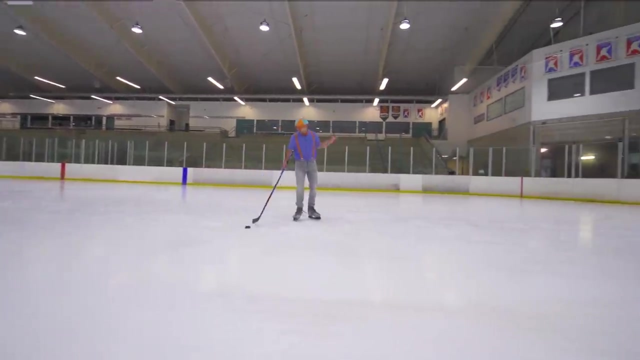 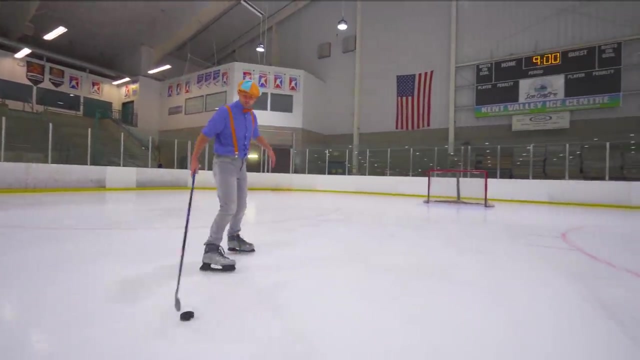 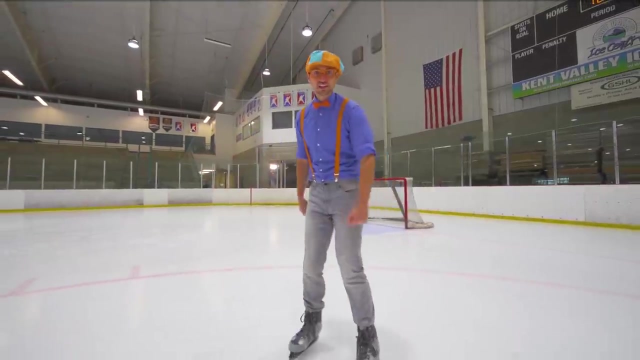 put it down vertically, like that, put it down vertically, like that, and give it a whack, and give it a whack, and give it a whack. check this out now. check this out now. check this out now for the next activity, for the next activity, for the next activity. i have a handle. 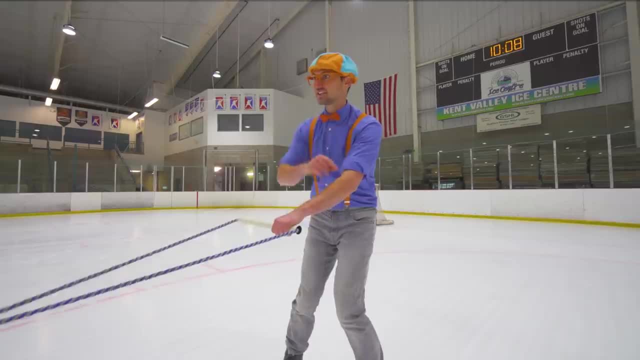 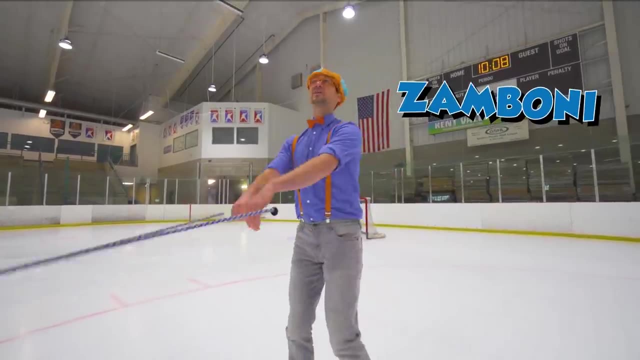 i have a handle. i have a handle and a rope and it's attached to the back and a rope and it's attached to the back and a rope and it's attached to the back of the zamboni, of the zamboni, of the zamboni, and for this sport i call it zamboni. 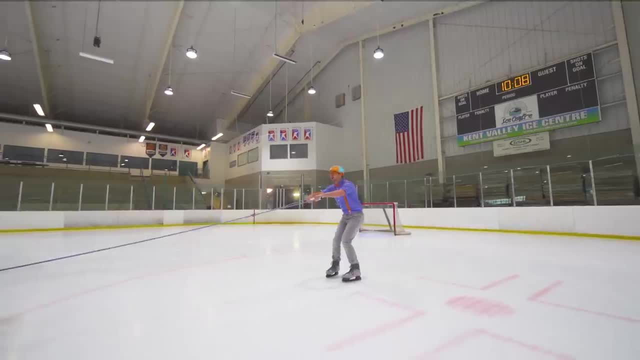 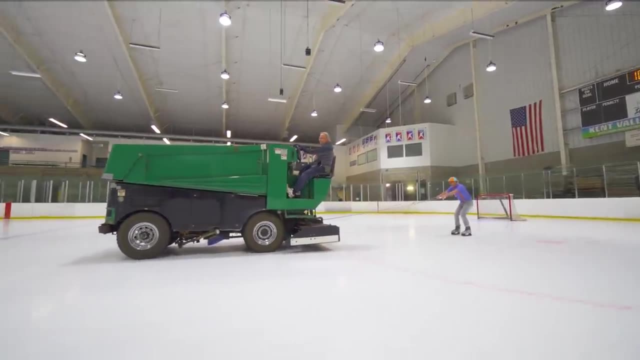 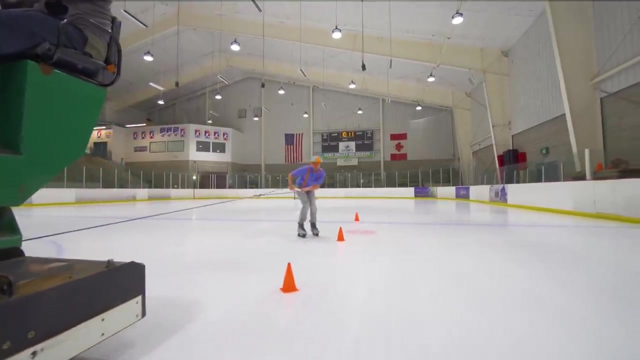 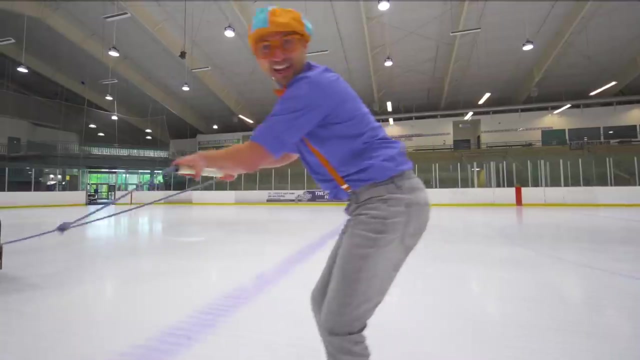 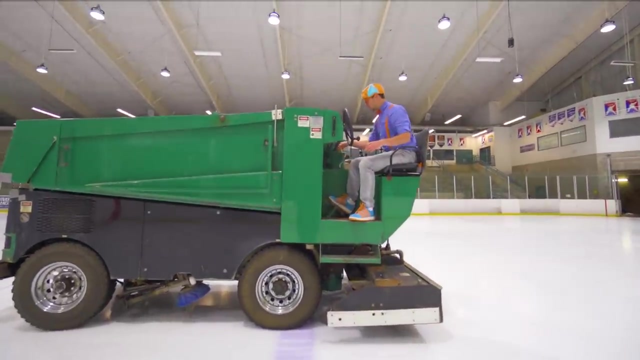 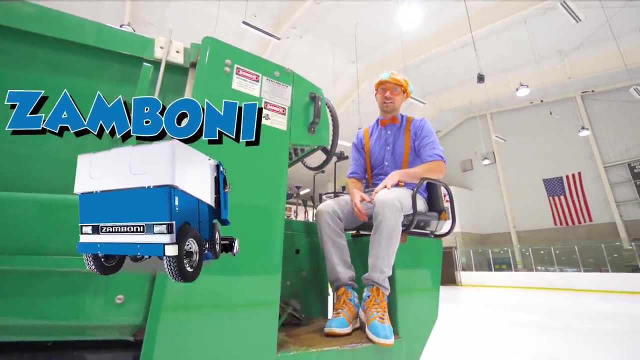 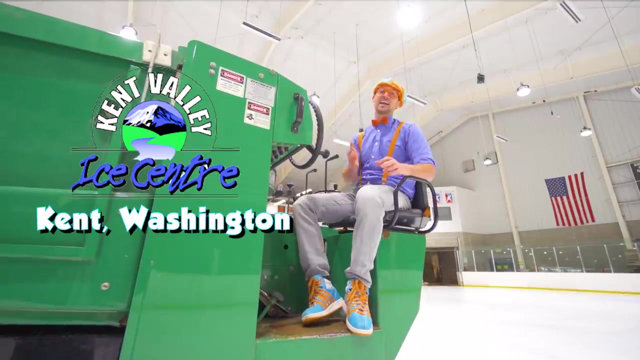 and for this sport, i call it zamboni. and for this sport, i call it zamboni skating. all right, all right, all right. that was so much fun learning about the zamboni with you, as well as hockey and ice skating. special thanks to the kent valley ice center. wow, what a fun time with you. 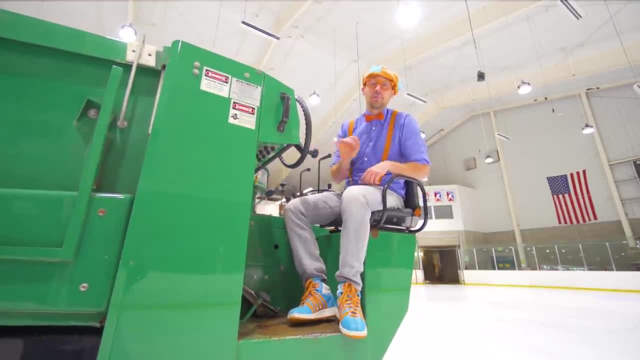 all right, that was so much fun learning about the zamboni with you, as well as hockey and ice skating. special thanks to the kent valley ice center. wow, what a fun time we had. well, this is the end of this video, but if you want to watch more of my videos, well, this is the end of this video. but if you want to watch more of my videos, well, this is the end of this video. but if you want to watch more of my videos, all you have to do is search for my name. all you have to do is search for my name. 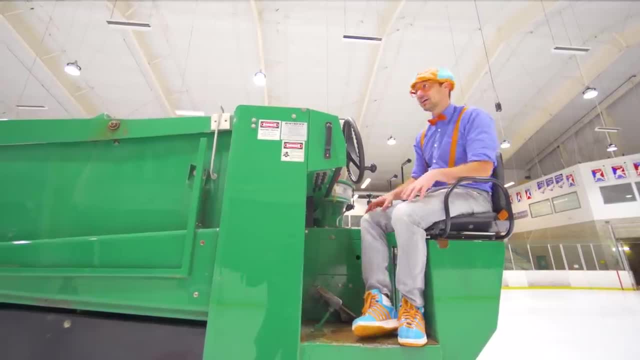 all you have to do is search for my name. will you spell my name with me? will you spell my name with me? will you spell my name with me? okay, okay, okay. b-l-i, b-l-i, b-l-i, p-p-i, p-p-i, p-p-i, plippy.